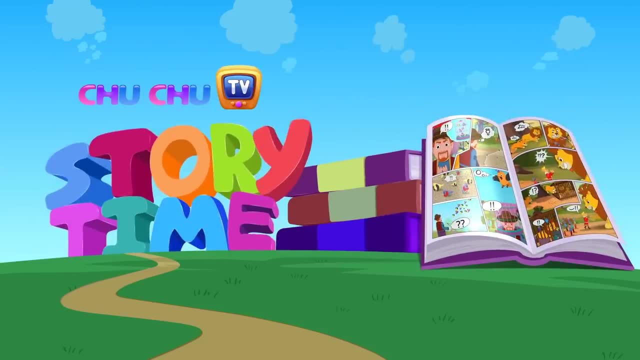 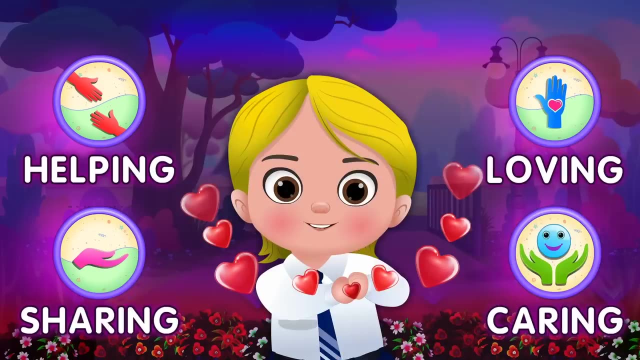 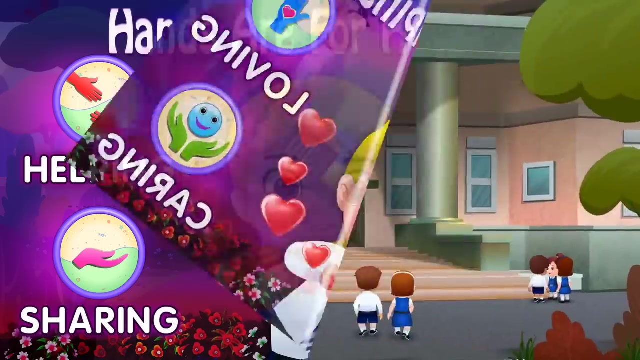 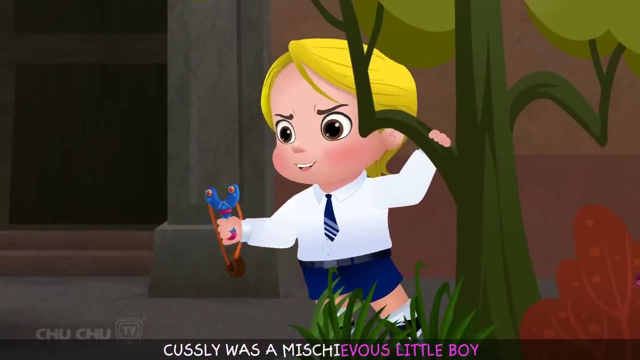 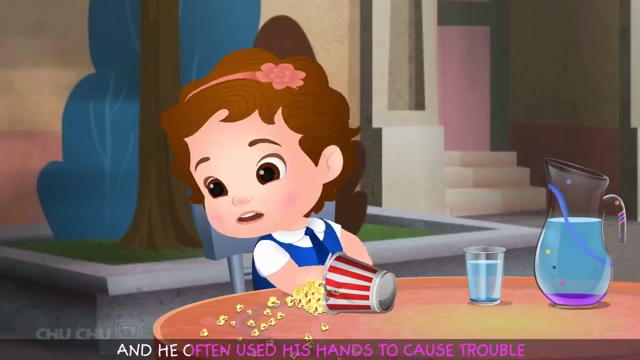 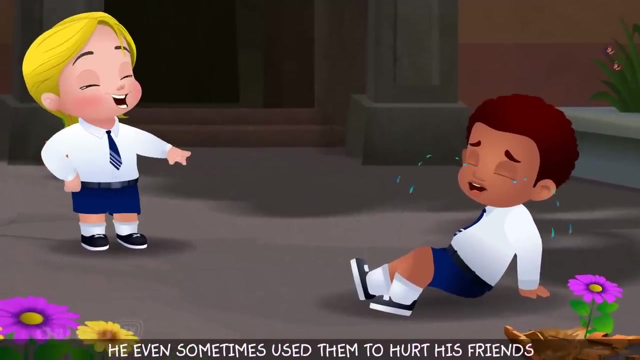 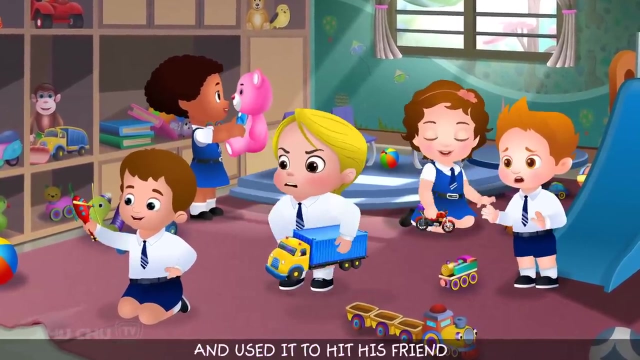 Chuchu TV Story Time. Custly was a mischievous little boy. He didn't know how to do nice things And he often used his hands to cause trouble. He even sometimes used them to hurt his friends. One day in the playroom, Custly picked up a toy truck and used it to hit his friend. 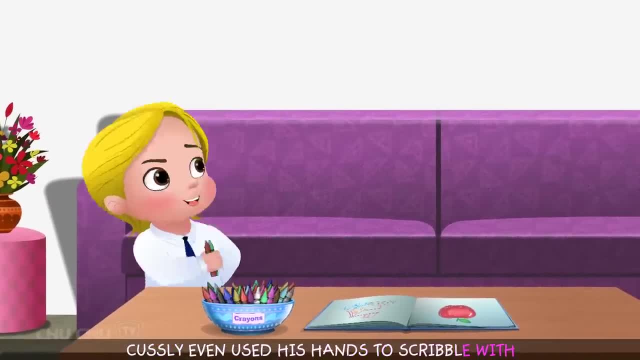 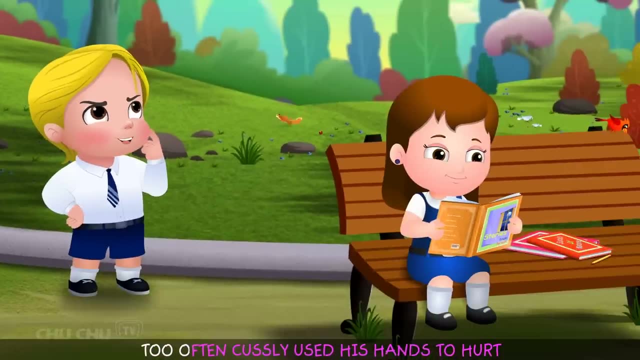 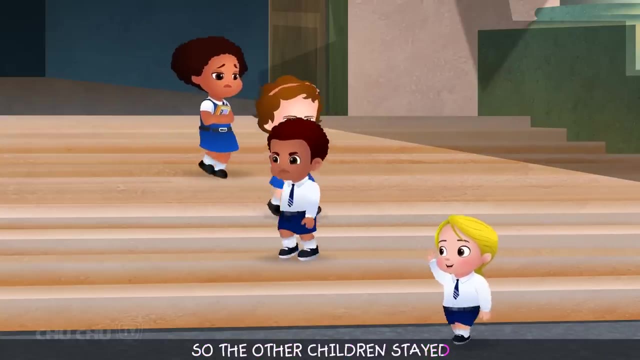 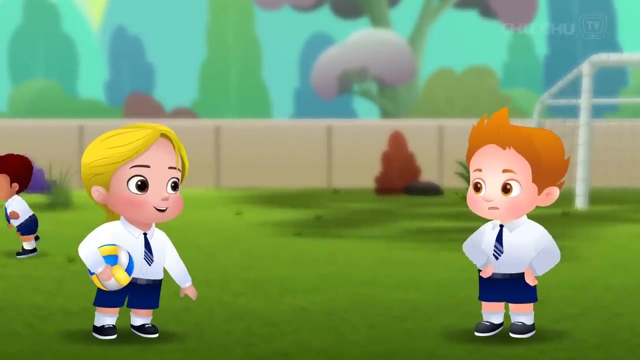 Custly even used his hands to scribble with his friends. It ran all over the clean white wall. Too often Custly used his hands to hurt and ruin things, So the other children stayed far away from him. This made Custly angry. 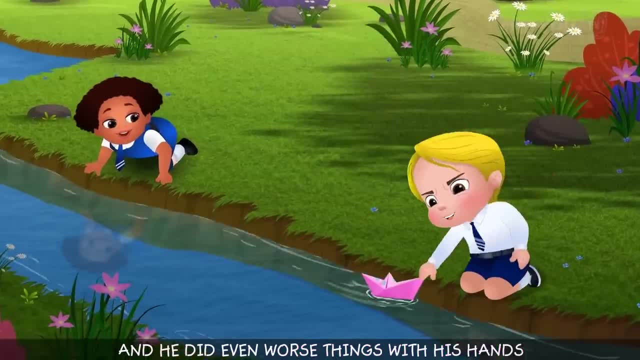 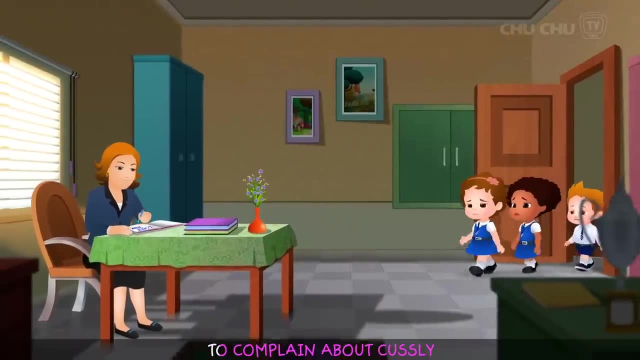 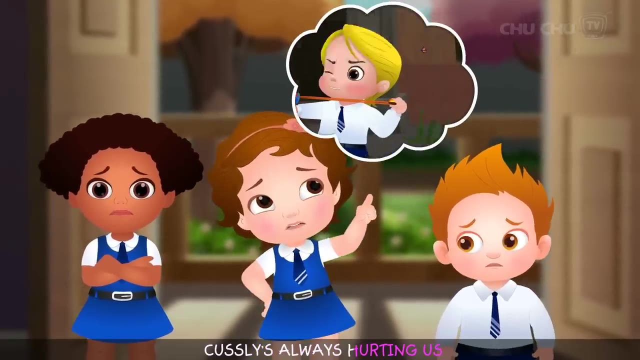 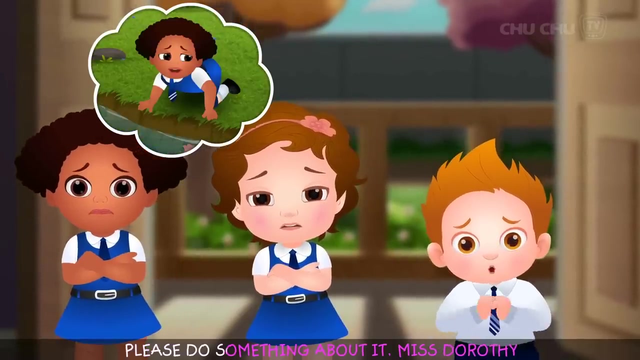 And he did even worse things with his hands. One day the children went to their teacher to complain about Custly. Miss Dorothy, Custly's always hurting us. He breaks and ruins everything. Please do something about it, Miss Dorothy. Hmm. 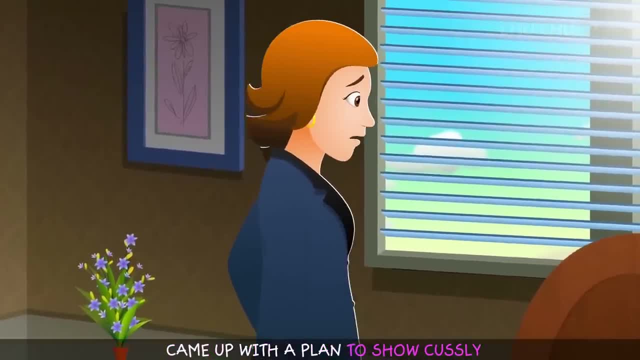 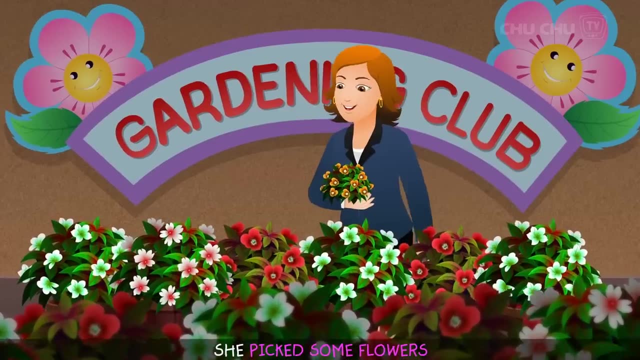 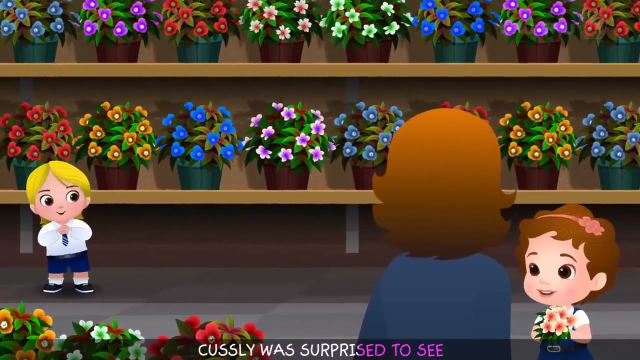 Miss Dorothy came up with a plan to show Custly how he could use his hands to make everyone happy. She picked some flowers and gave one to each of the children. Custly was surprised to see how the children smiled each time Miss Dorothy handed out a flower. 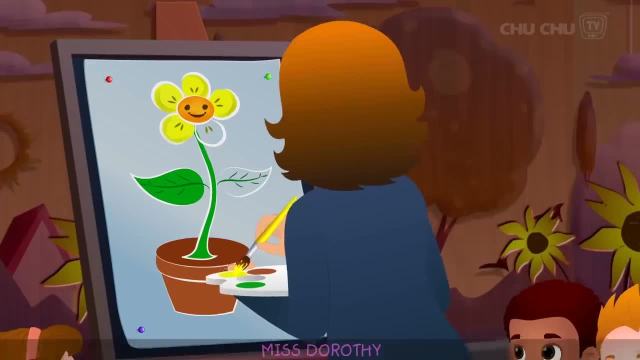 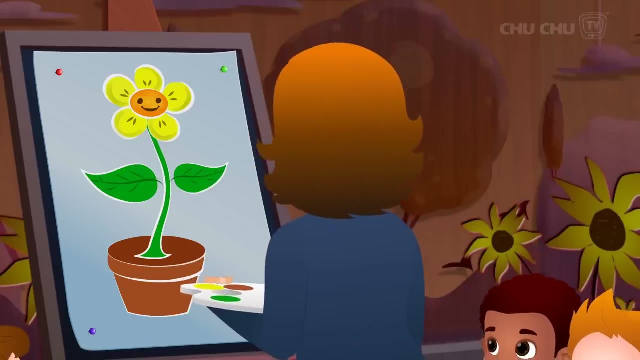 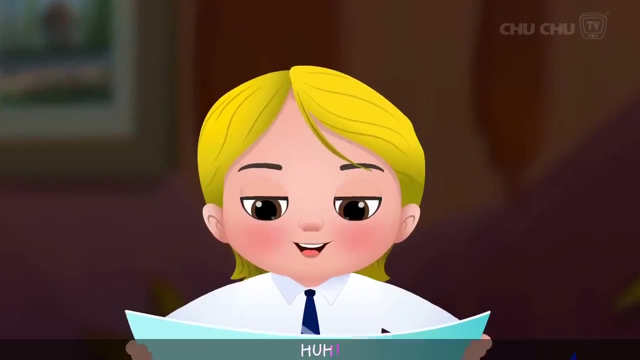 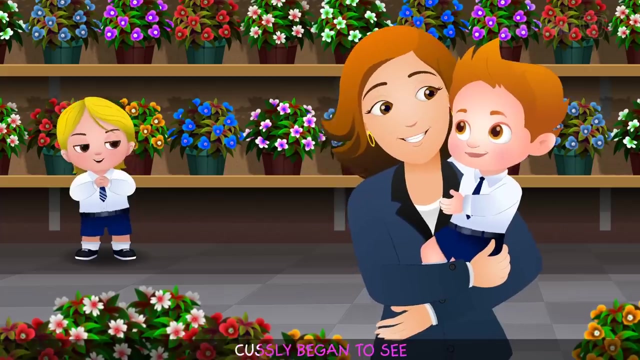 Huh. Miss Dorothy then painted a beautiful picture And Custly saw how everyone smiled at the picture. Huh. Next, Miss Dorothy used her hands to hug some of the children. Custly began to see how much joy hands could bring. 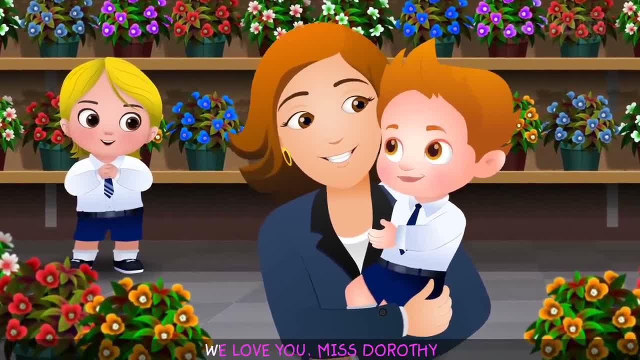 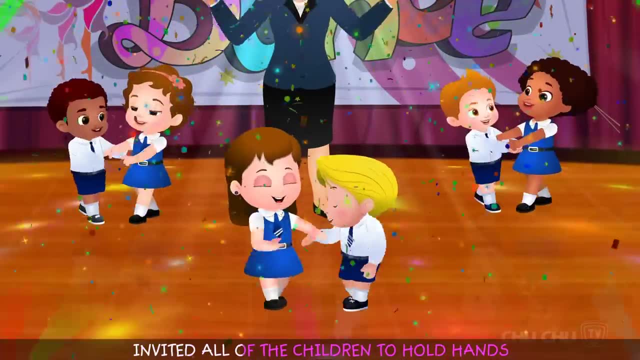 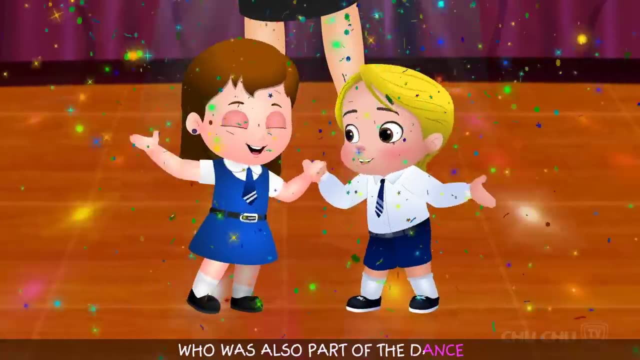 I love you, little one. We love you, Miss Dorothy. One day, Miss Dorothy invited all of the children to hold hands and dance around together. Custly, who was also part of the dance, found that he was feeling very happy too. 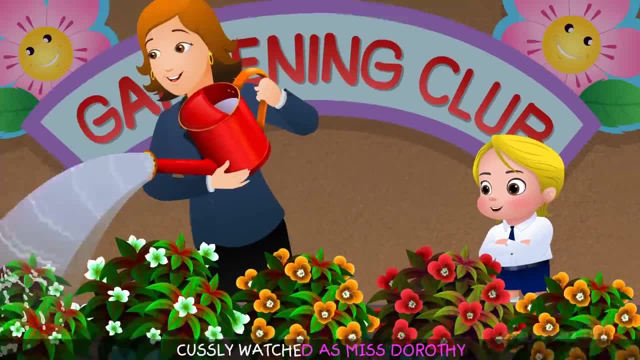 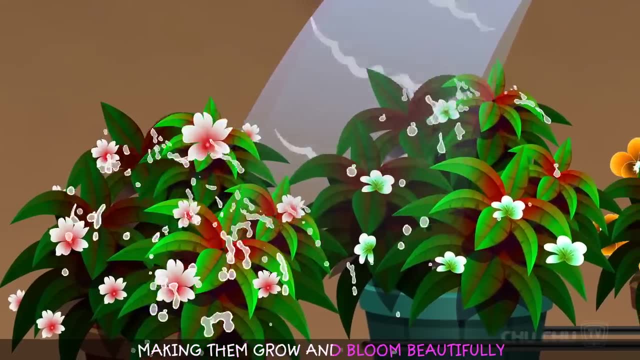 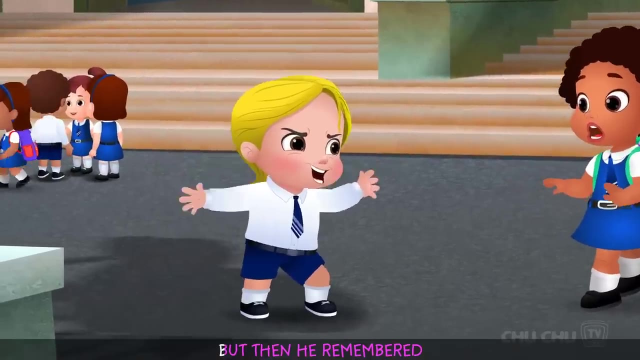 Hehehe, Custly watched as Miss Dorothy used her hands to water the plants, Making them grow and bloom beautifully. One day Custly was about to push a girl, But then he remembered all of the wonderful things Miss Dorothy had done with her hands. 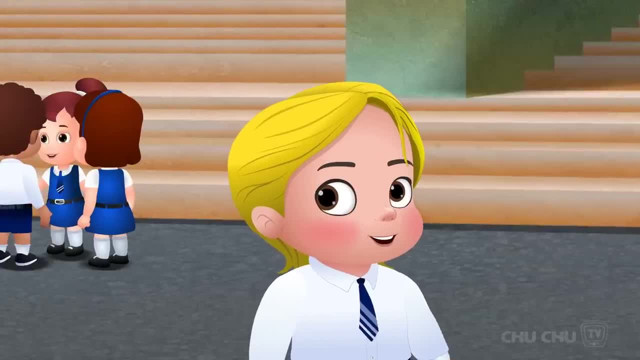 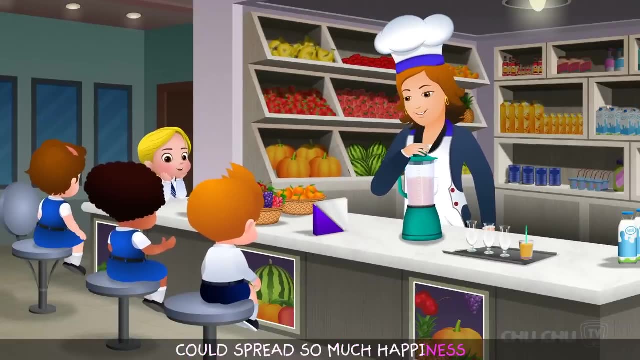 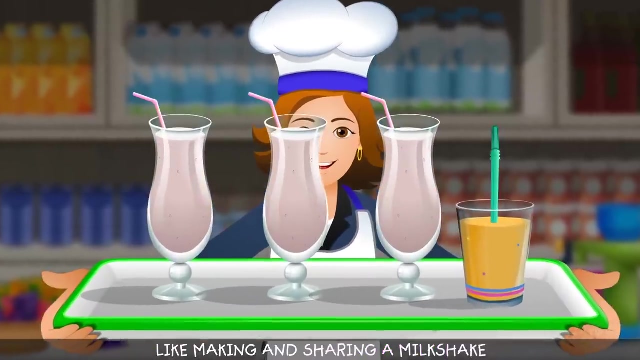 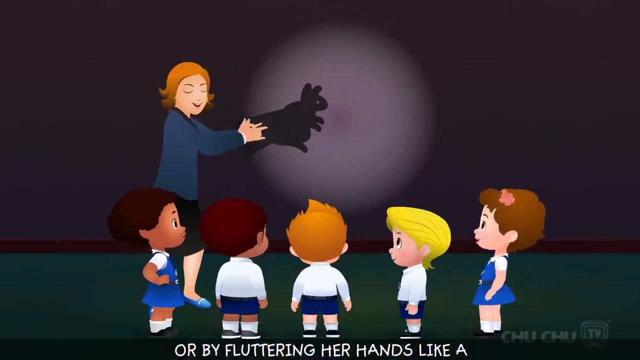 And he stopped himself Custly noticed how Miss Dorothy could spread so much happiness by doing little things with her hands, Like making and sharing a milkshake Or cutting cookies into fun shapes, Or by fluttering her hands like a butterfly's wings. 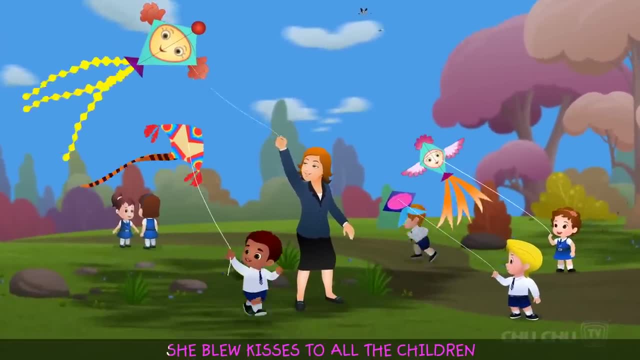 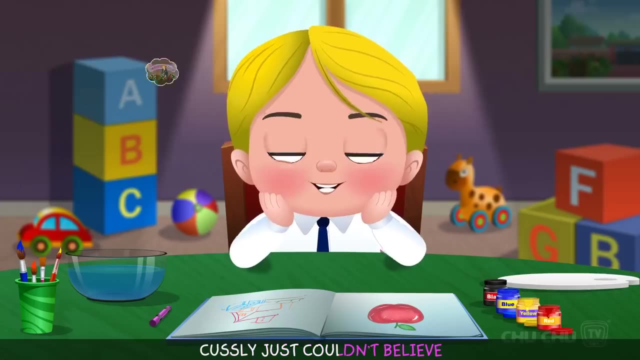 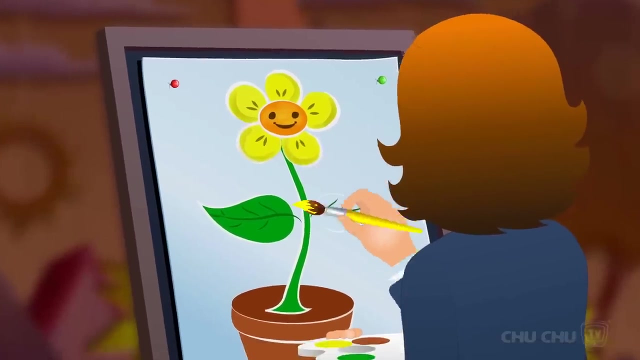 She blew kites in the sky. She blew kisses to all the children. Mwah Custly just couldn't believe how much happiness Miss Dorothy had. Miss Dorothy could spread with her hands One day. Miss Dorothy called Custly over. 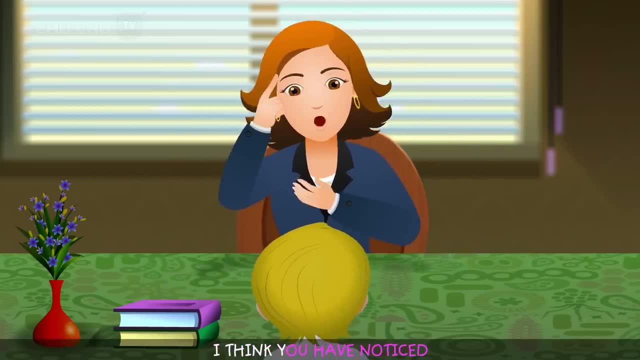 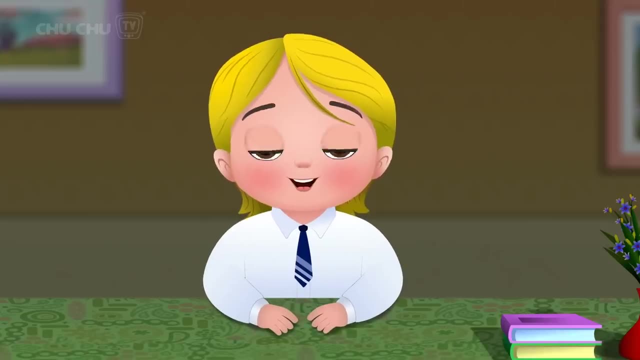 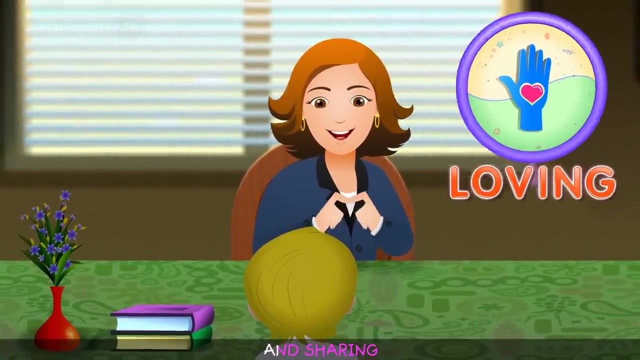 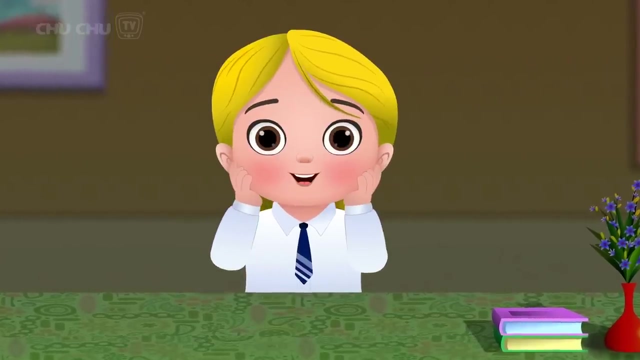 Custly. I think you have noticed just how many wonderful things we can do with our hands, And that our hands are for helping And loving And caring And sharing And caring And not for hurting others. If you use your hands to do nice things, everyone will love you. 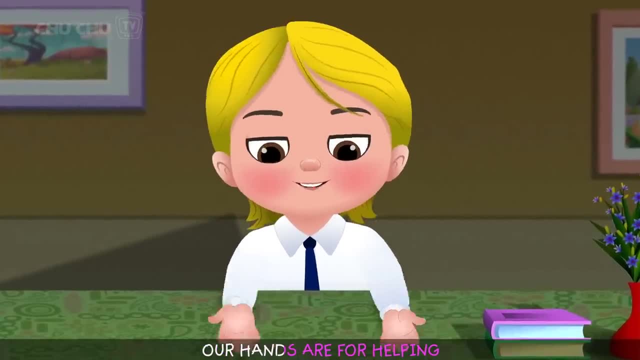 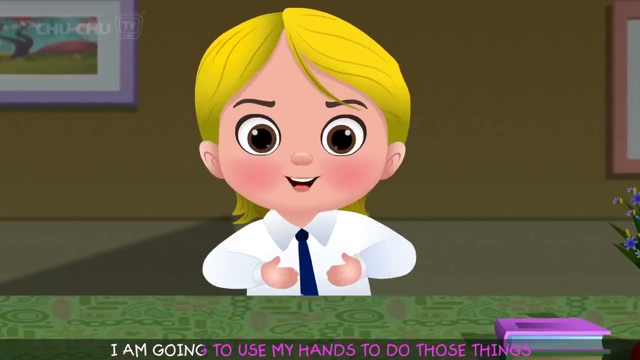 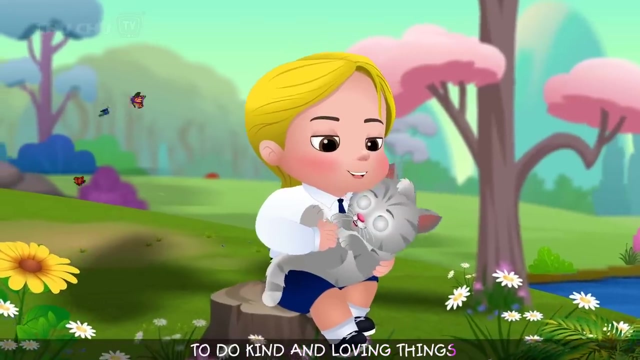 You are right, Miss Dorothy. Our hands are for helping And loving And sharing And caring, And from now on I'm going to use my hands to do those things. Custly used his hands to do kind things. He used his hands to do kind and loving things. 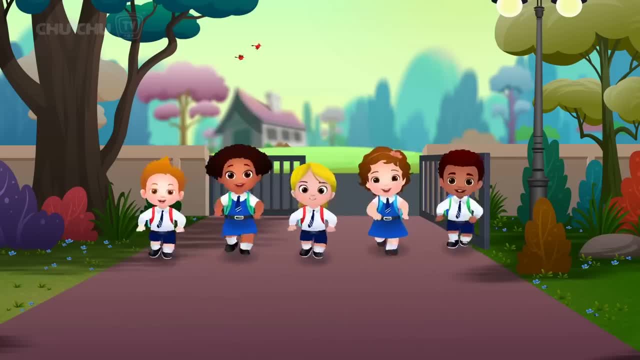 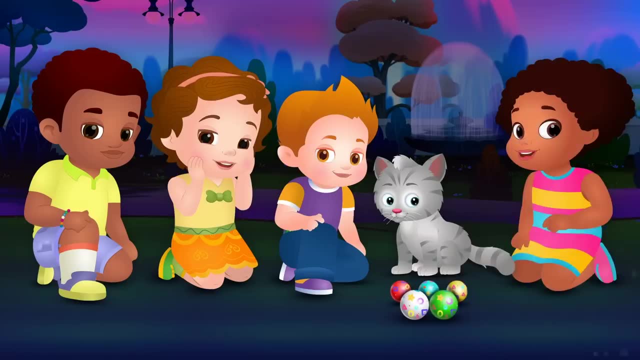 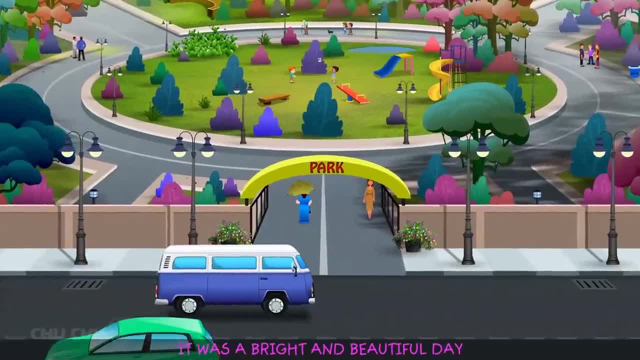 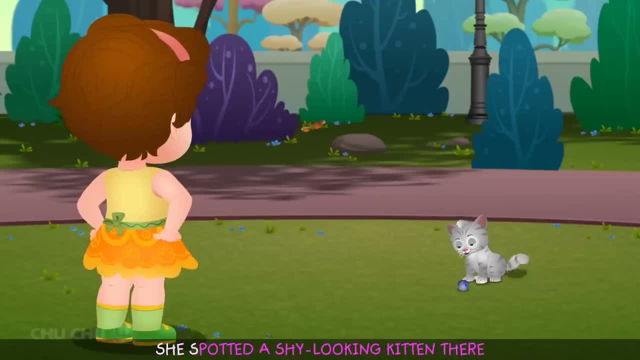 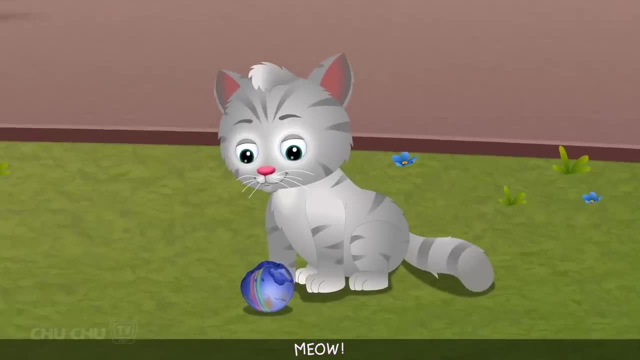 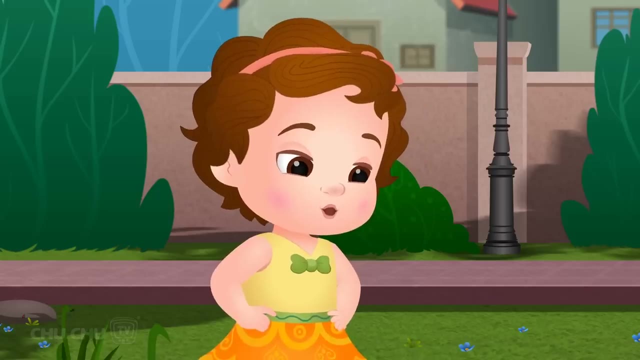 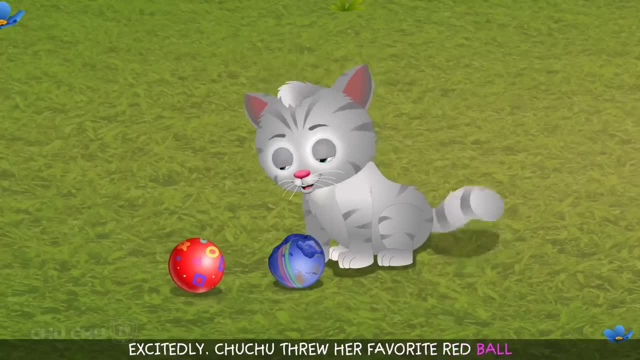 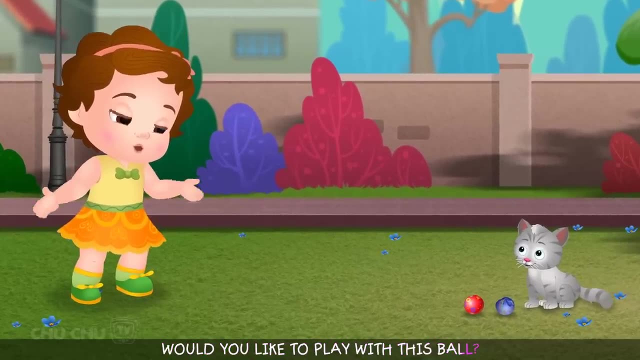 Hooray, Hooray, Hooray, Hooray, Hooray, Hooray, Hooray. Little kitty, would you like to play with this ball? It's nice and bouncy. The kitten was delighted. 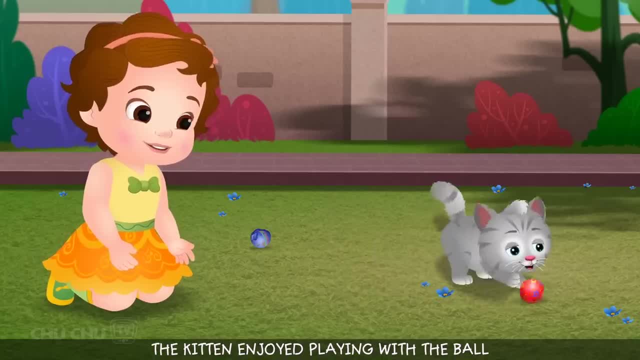 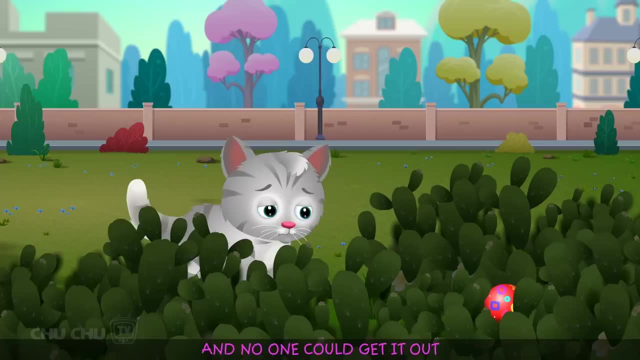 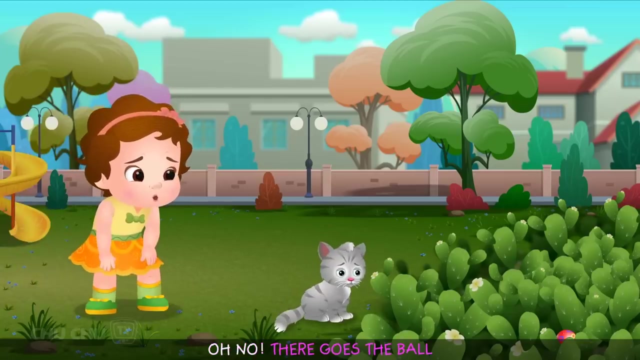 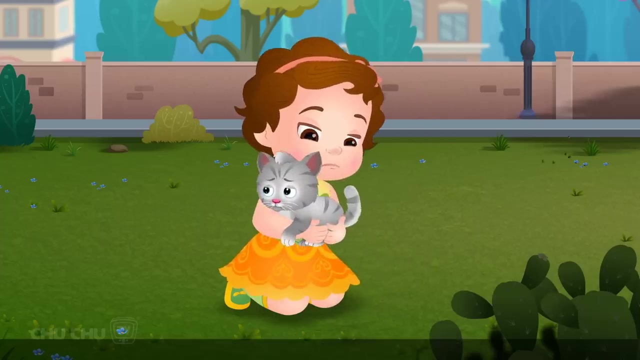 The kitten enjoyed playing with the ball, But then the ball rolled into a thorny bush And no one could get it out. Oh no, There goes the ball. We were having so much fun playing with it. Just then Chacha came by. 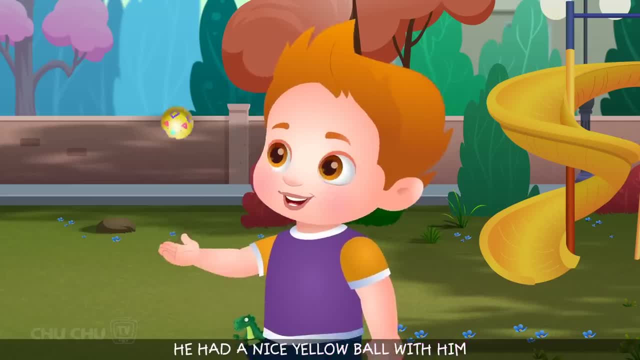 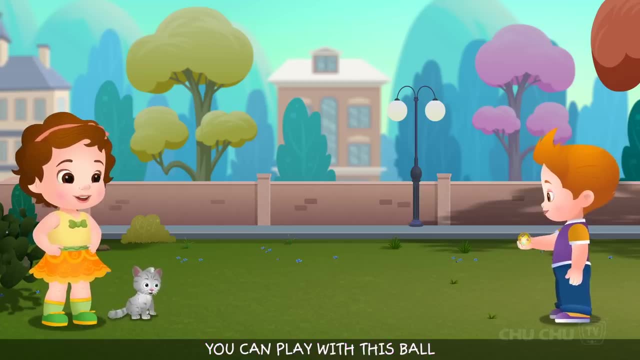 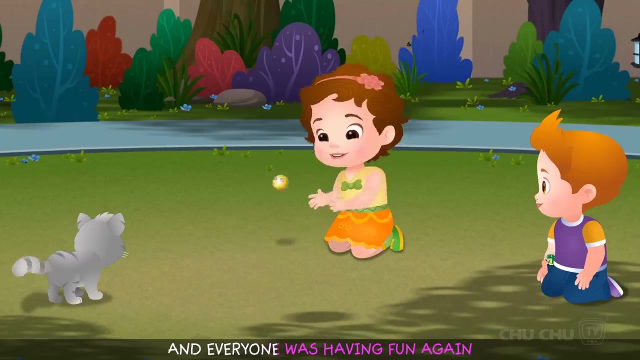 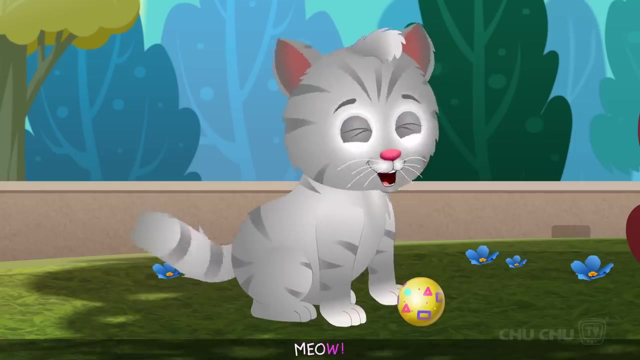 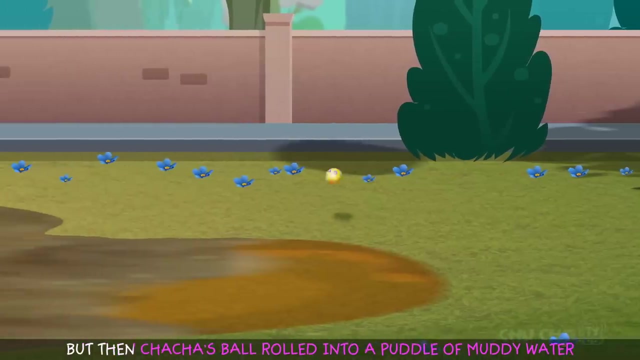 He had a nice yellow ball with him. Here, little kitten, you can play with this ball. Chacha shared his ball, Passing it to the kitten, And everyone was having fun again. But then Chacha's ball rolled into a puddle of muddy water. 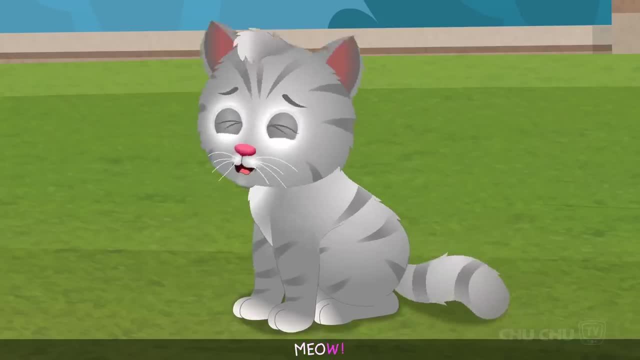 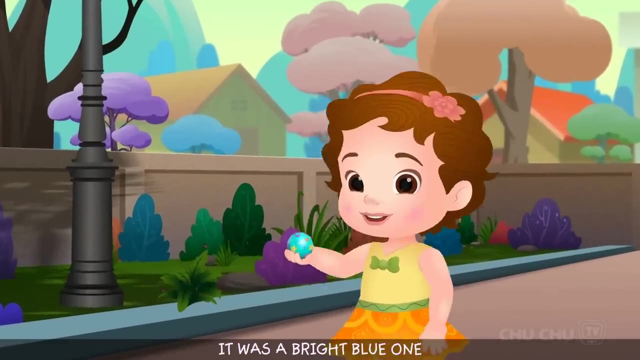 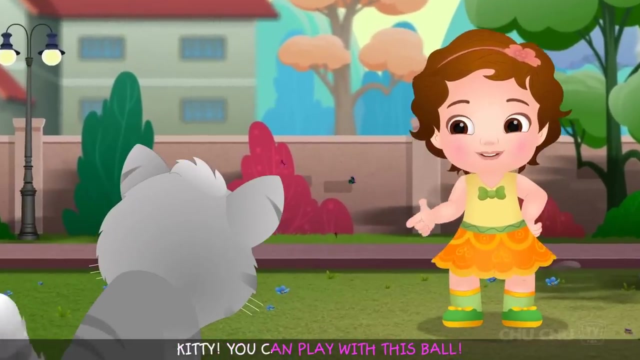 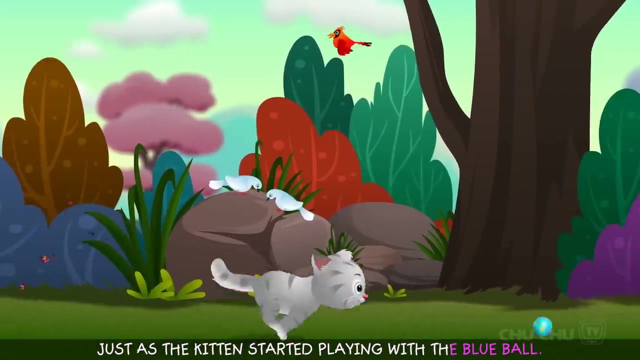 Uh oh. So Chuchu brought another ball. It was a bright blue one. Chuchu gave it to the kitten to play with it. Kitty, you can play with this ball- Just as the kitten started playing with the blue ball. 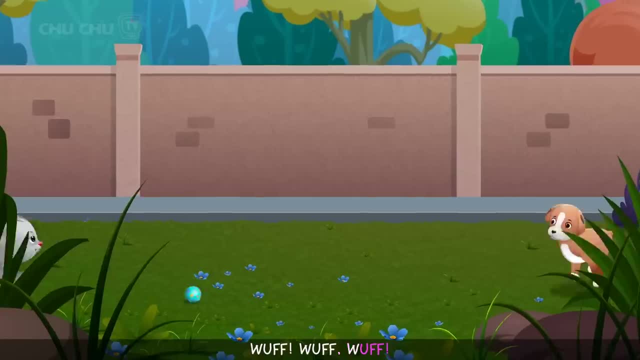 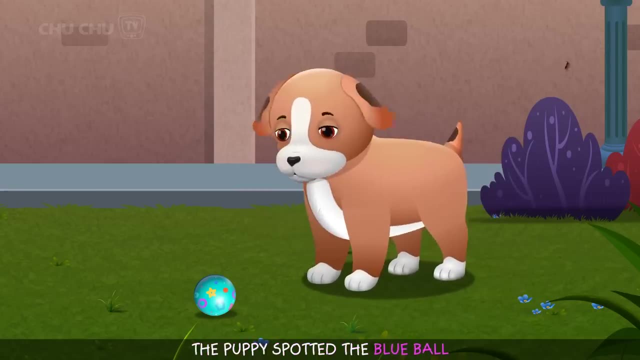 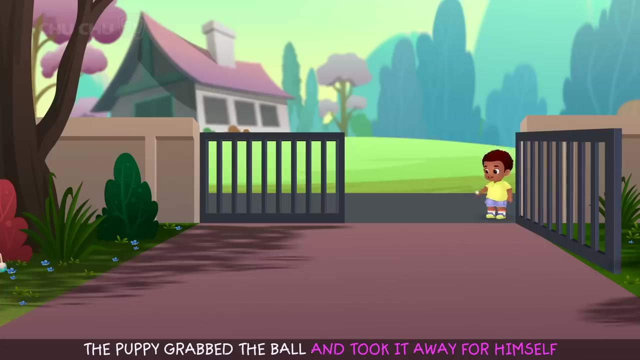 a frisky little puppy ran into the garden. Chuchu, you can play with this ball. Chuchu, you can play with this ball. The puppy spotted the blue ball And, to everyone's surprise, the puppy grabbed the ball and took it away for himself. 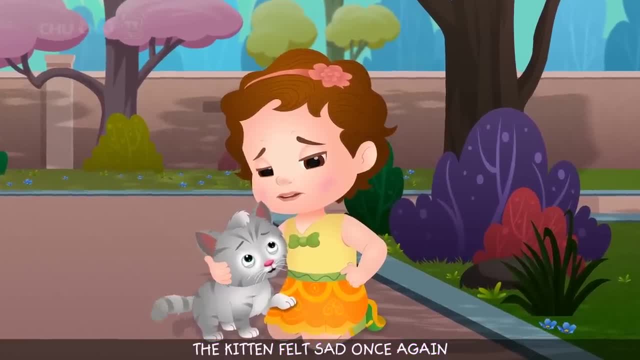 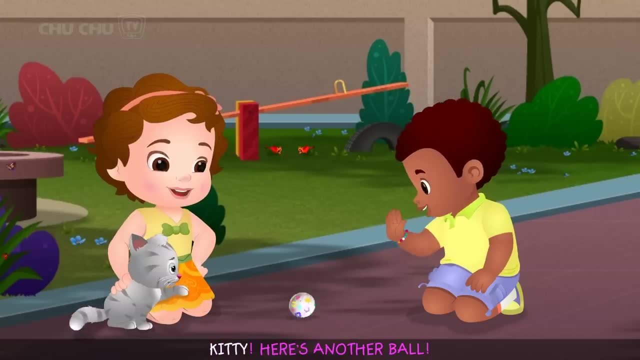 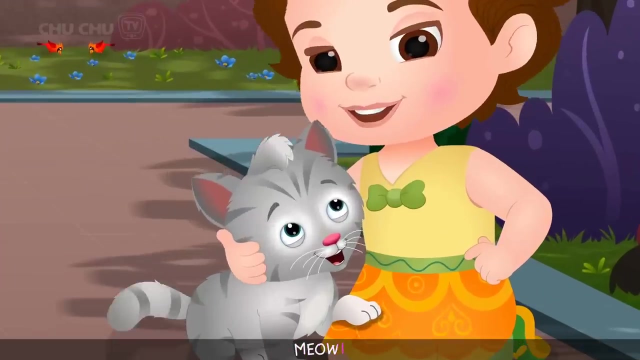 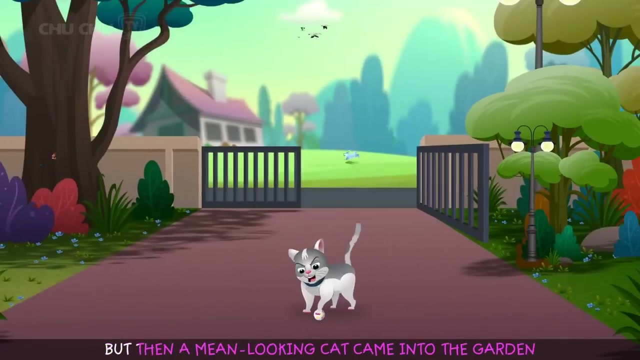 The kitten felt sad once again. Then Chica came into the garden. He had a shiny white ball with him. Kitty, here's another ball You can play with this one. Chica's ball made the kitten happy once again. But then a mean-looking cat came into the garden. 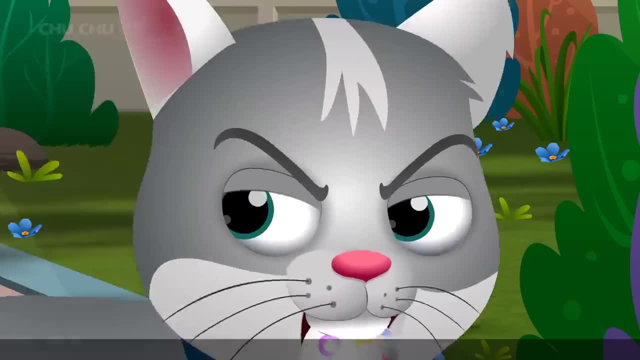 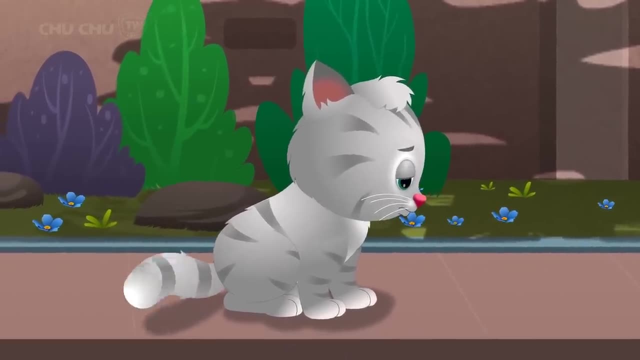 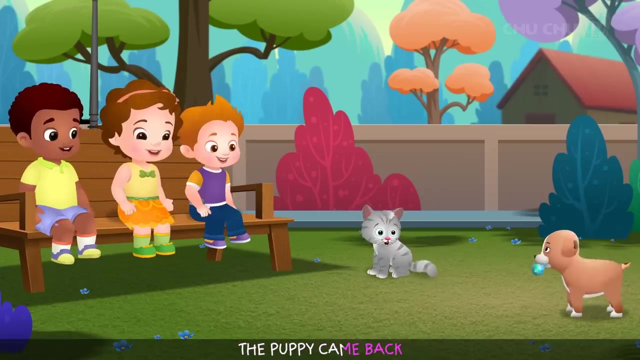 The cat took the white ball away And the kitten was sad again. But then, to everyone's surprise, the puppy came back and returned the ball to the kitten. Then, to everyone's surprise, the puppy came back and returned the ball to the kitten. 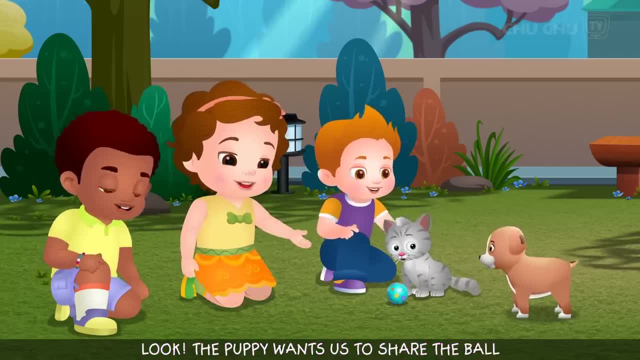 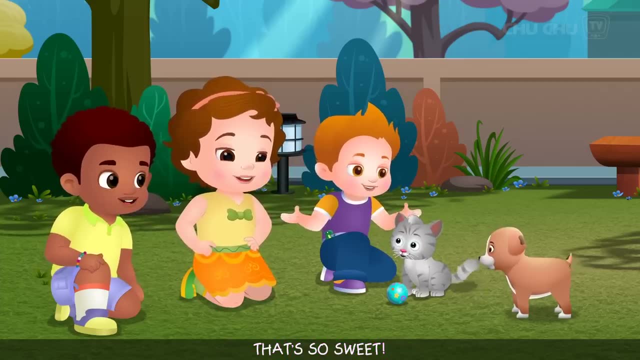 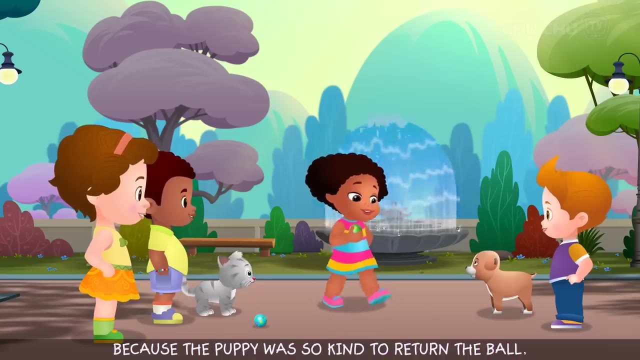 Look, the puppy wants us to share the ball, So we can all be happy. That's so sweet. That's so sweet, Meow, Meow, Meow. Because the puppy was so kind to return the ball, Chiku gave it a small green ball. 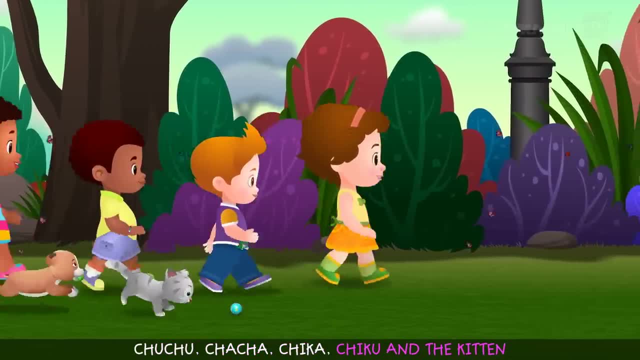 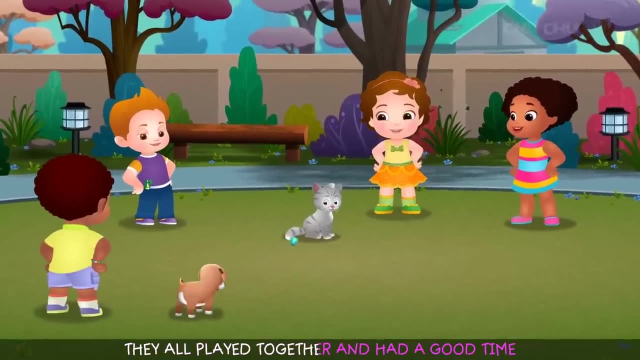 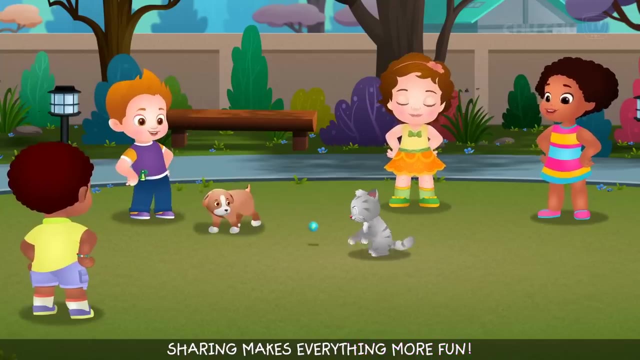 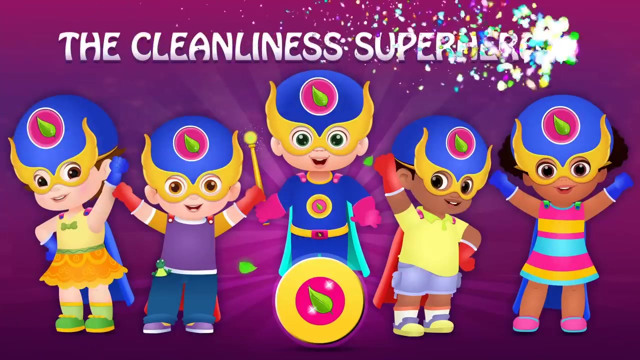 Chuchu Chacha, Chica Chiku and the kitten then invited the puppy to play with them. They all played together and had a good time. Sharing makes everything more fun. Meow, Meow, Let's show it. Chica and Ch relates too. 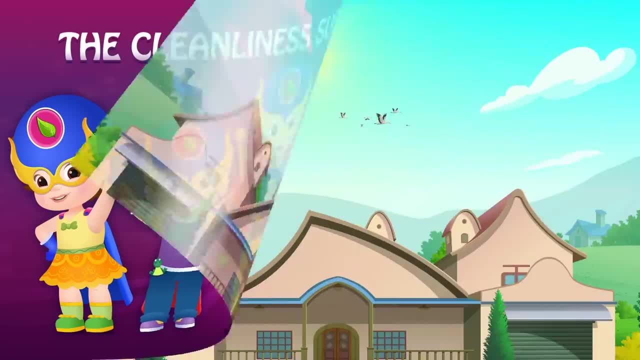 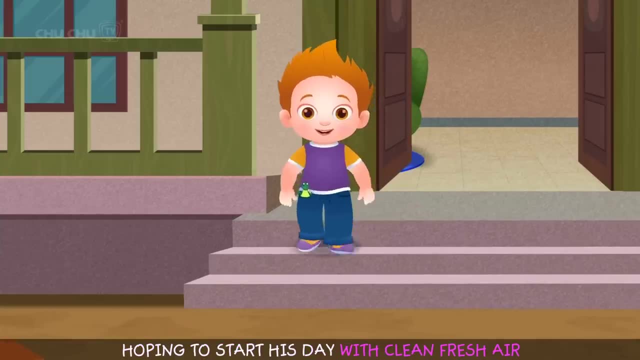 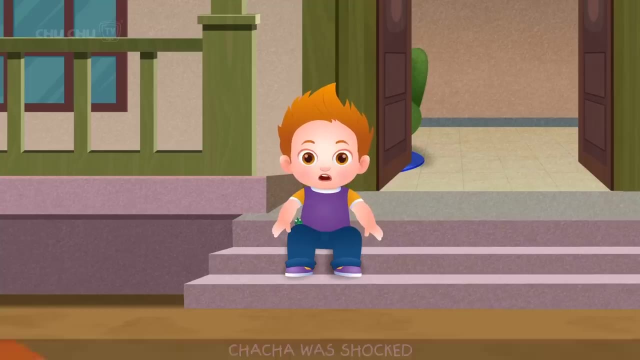 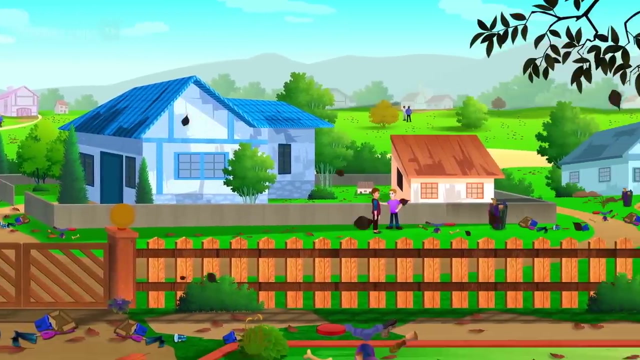 Meow, Meow. It's fun to work together. One morning, Chacha left his house hoping to start his day with clean, fresh air. Huh, Chacha was shocked to see that his neighborhood was so dusty and dirty. There was trash all over. 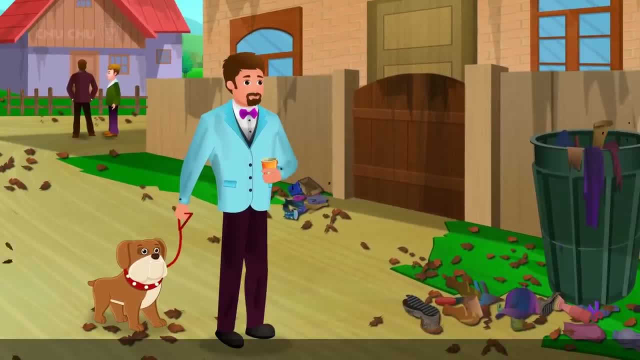 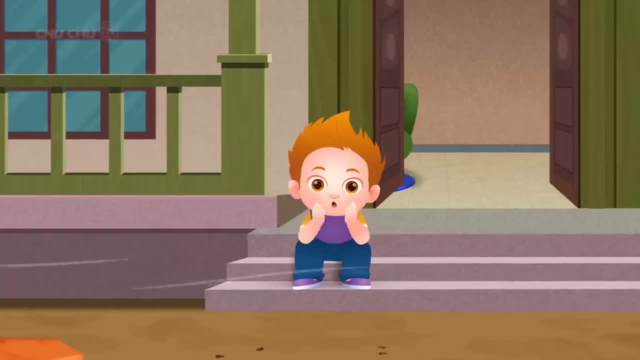 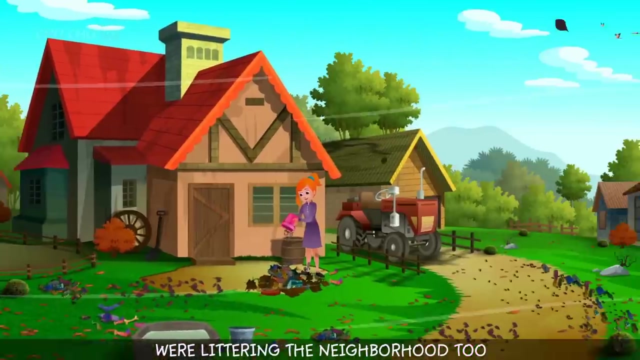 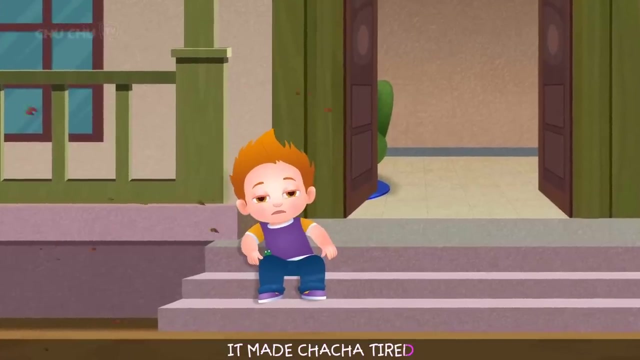 Cha-Cha watched as a man walking a dog through a paper cup on the street, even though there was a bin nearby. Many other people were littering the neighborhood too. The air didn't smell fresh or clean. It made Cha-Cha tired. 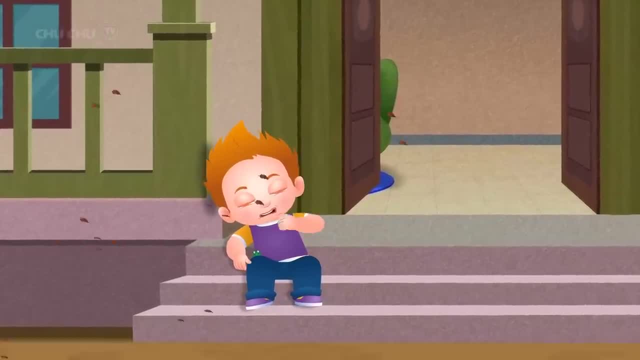 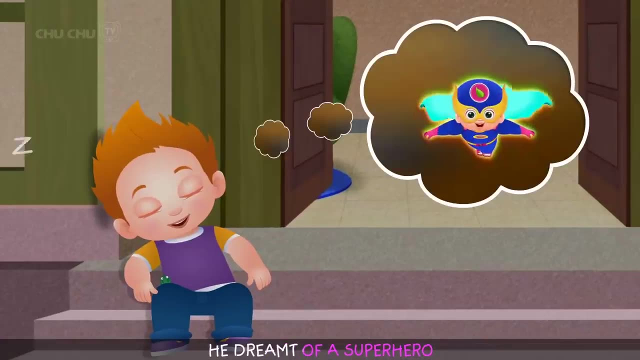 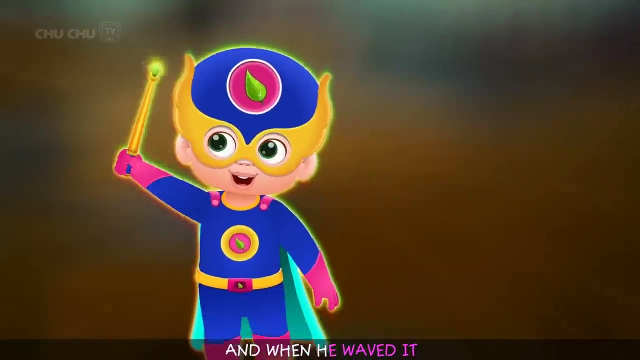 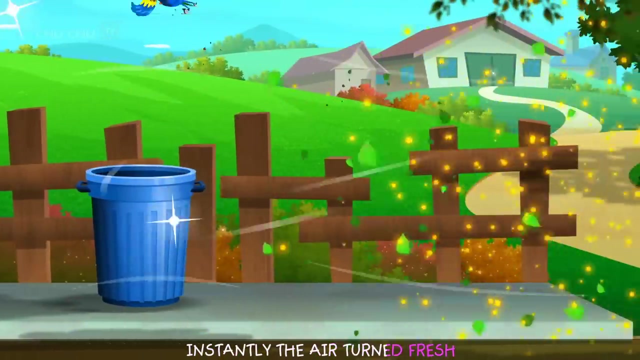 And soon he fell fast asleep. As Cha-Cha slept, he dreamt of a superhero. The superhero had a magical wand And when he waved it he made the neighborhood clean and green. Instantly, the air turned fresh and everyone in the neighborhood felt healthy, active. 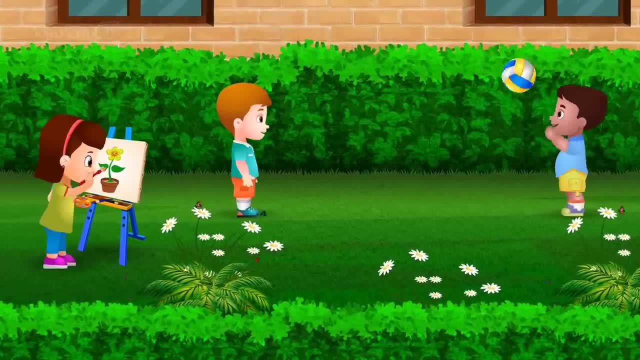 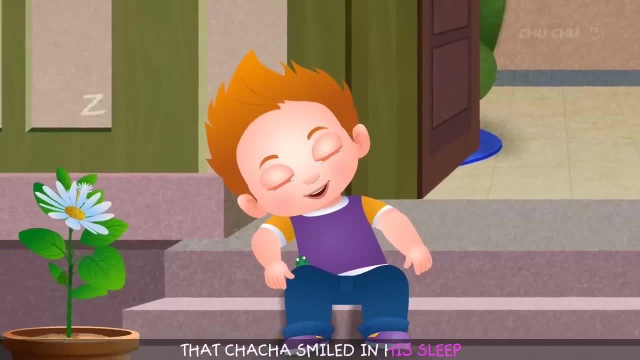 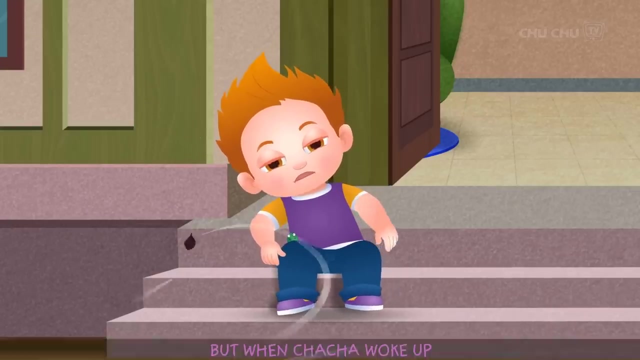 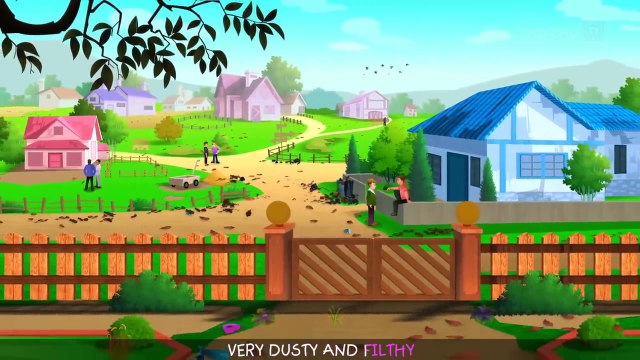 and excited And everyone in the neighborhood felt excited to enjoy themselves. The neighborhood in his dream felt so wonderful that Cha-Cha smiled in his sleep. But when Cha-Cha woke up he was disappointed to see that the neighborhood was still very dusty and filthy. 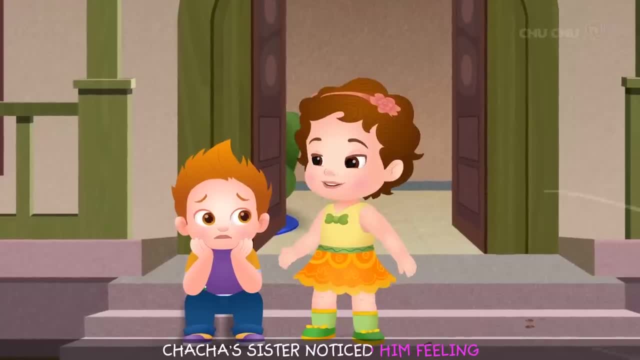 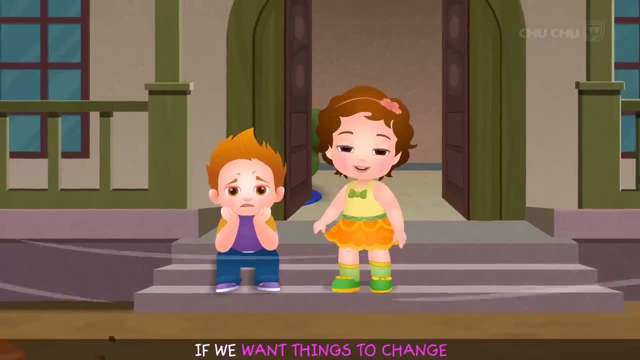 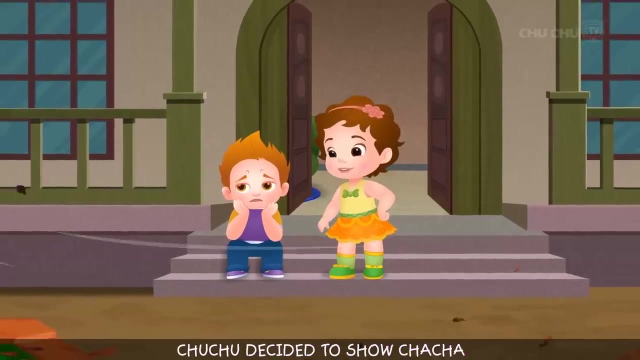 Cha-Cha's sister noticed him feeling disappointed by all the dirt around him. Hmm, If we want things to change, we must first change. Choo-Choo decided to show Cha-Cha and the other children how they themselves could make the neighborhood. 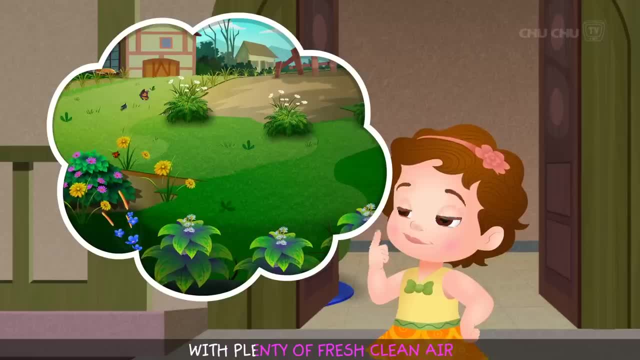 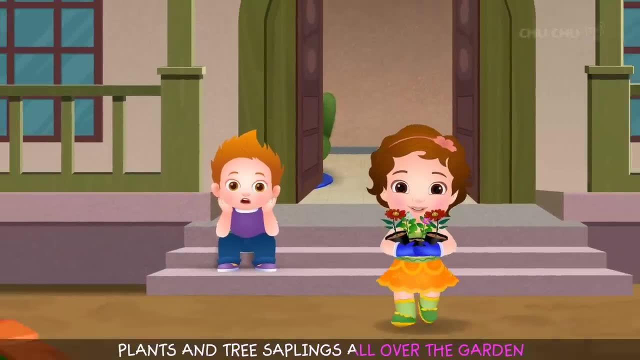 a cleaner and greener place with plenty of fresh, clean air. Choo-Choo decided to play with the neighborhood. Choo-Choo decided to play with the neighborhood. Choo-Choo planted small plants and tree saplings all over the garden. 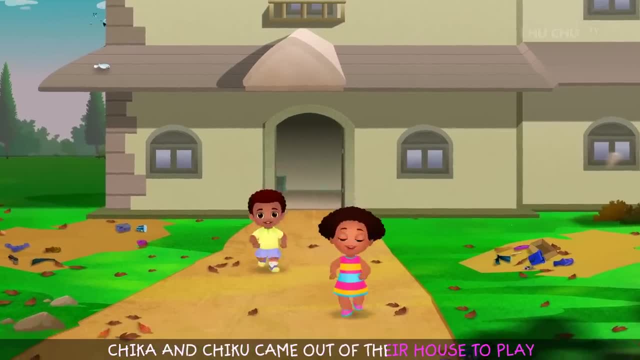 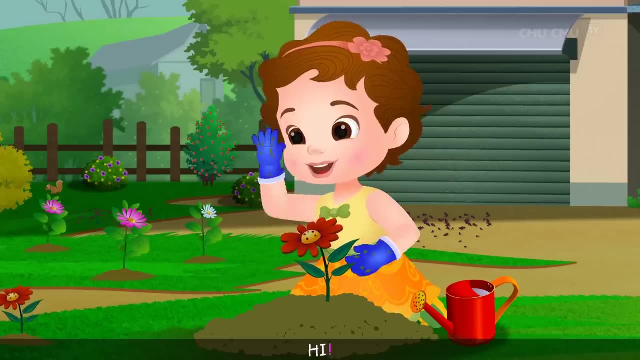 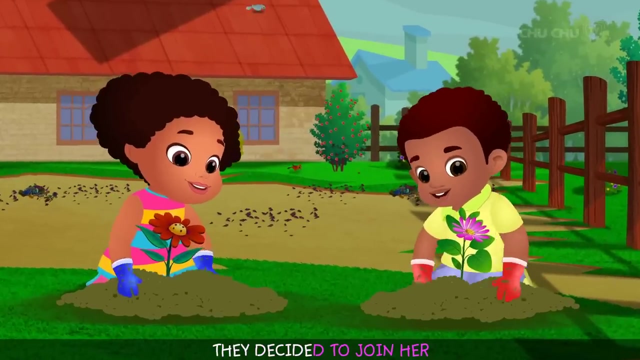 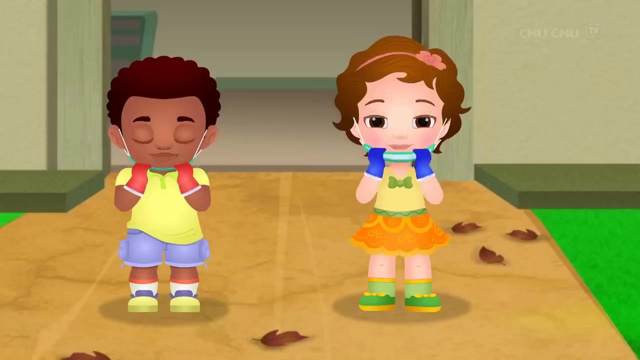 Soon, Chica and Chicoo came out of their house to play Hi Hi. But when they saw Choo-Choo planting the saplings, they decided to join her. Yay, I'm going to play with Choo-Choo. 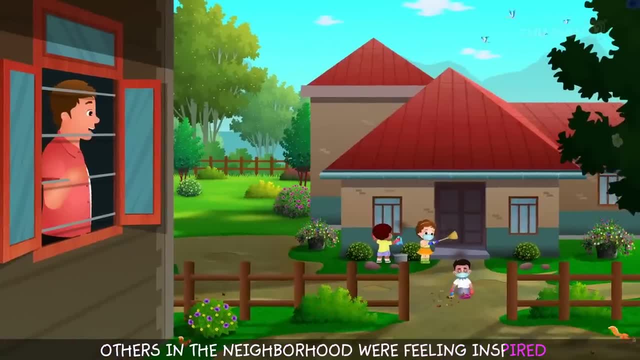 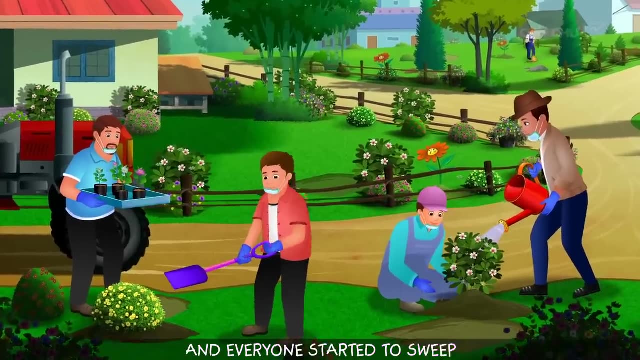 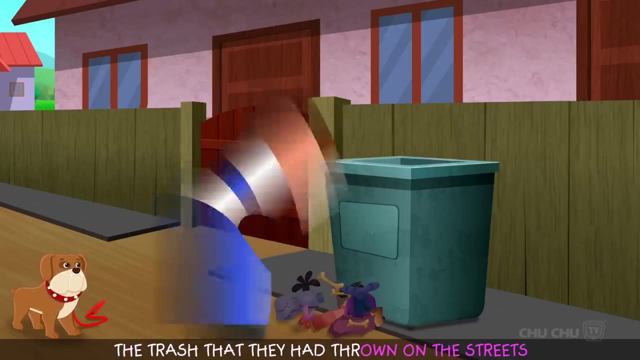 Soon, others in the neighborhood were feeling inspired by Choo-Choo, Chica and Chicoo, And everyone started to sweep and clean up their surroundings. The neighbors even picked up the trash that they had thrown on the streets. In no time, the entire neighborhood. 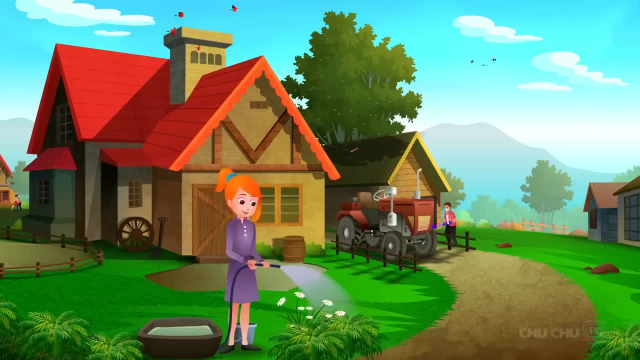 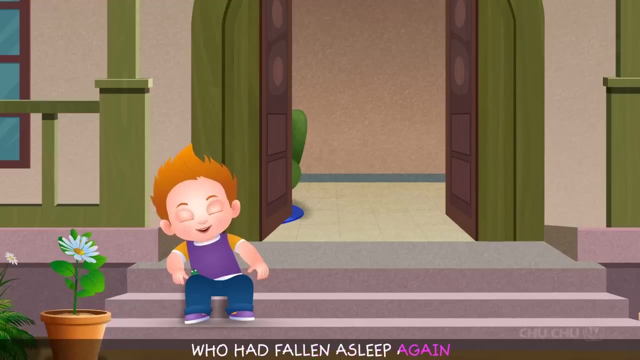 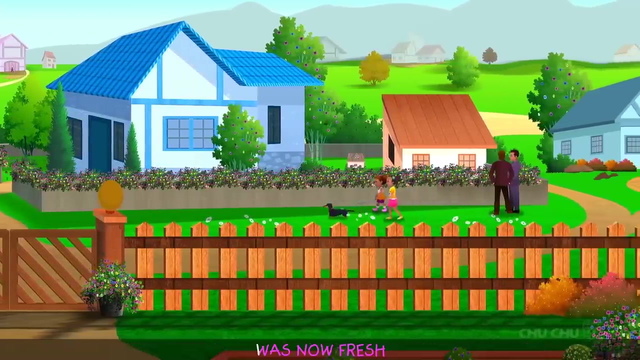 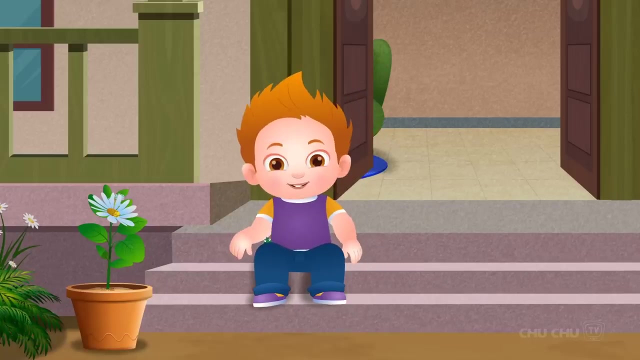 was spicked out. Choo-Choo and spam. cha-cha, who had fallen asleep, again woke up. he looked around and was happy to see that everything around him was now fresh, clean and green. cha-cha decided to plant a sapling, like choo-choo and his friends had he too. 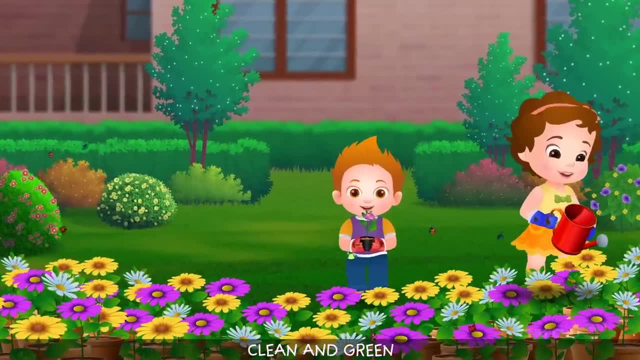 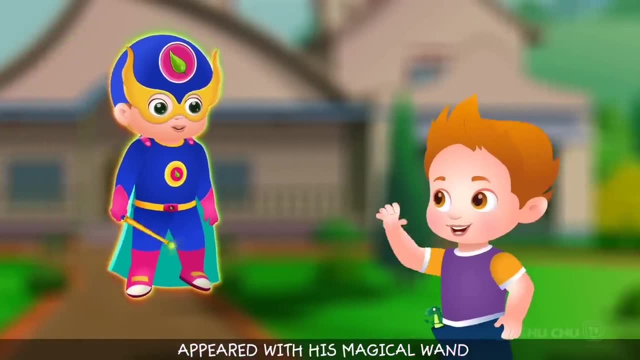 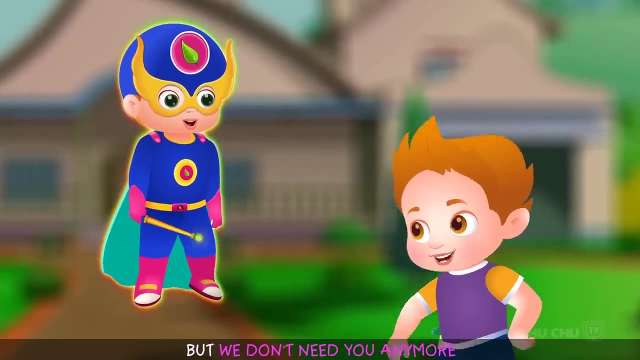 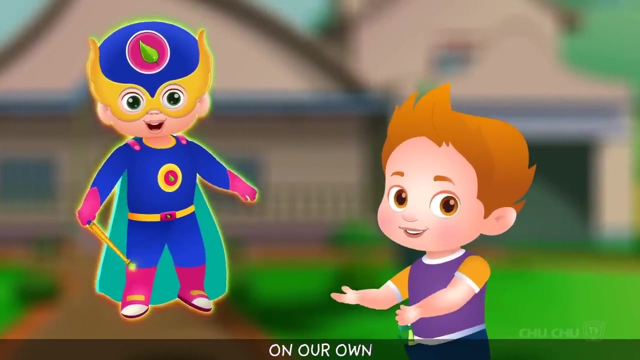 wanted to make the neighborhood clean and green. just then, the superhero cha-cha had dreamt of appeared with his magical wand. hello, Thank You, superhero, but we don't need you anymore. my friends and I have cleaned up the neighborhood on our own. we planted lots of plants and trees, and 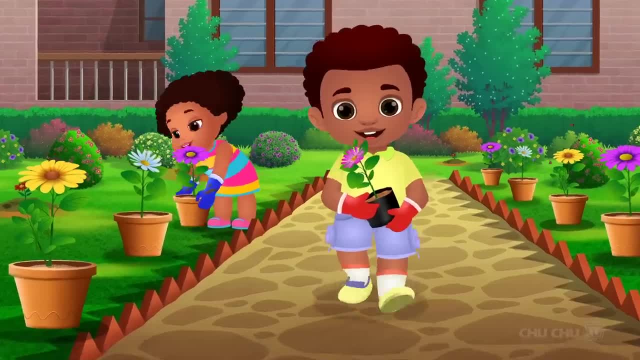 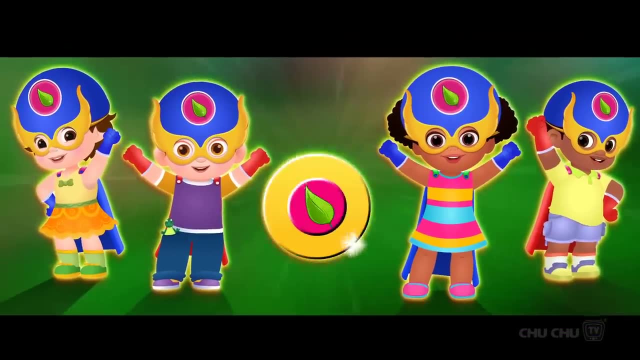 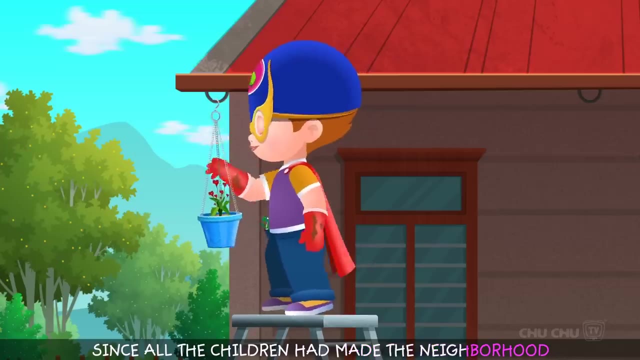 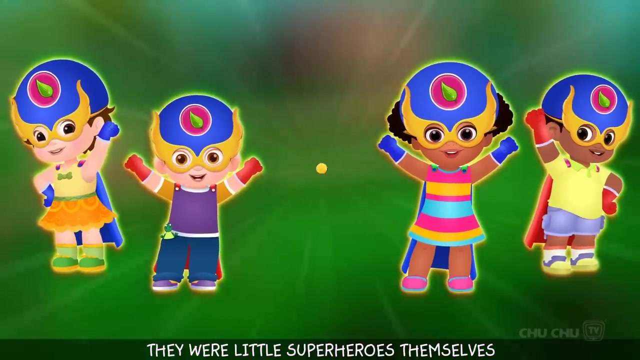 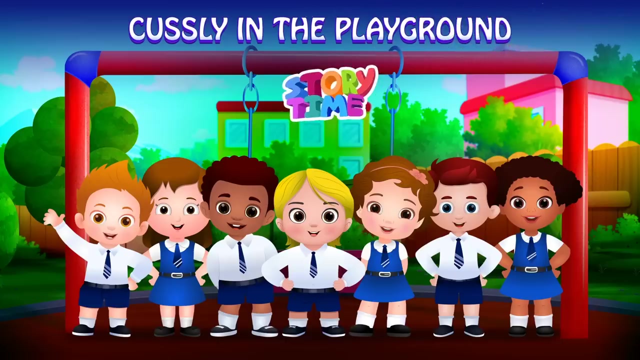 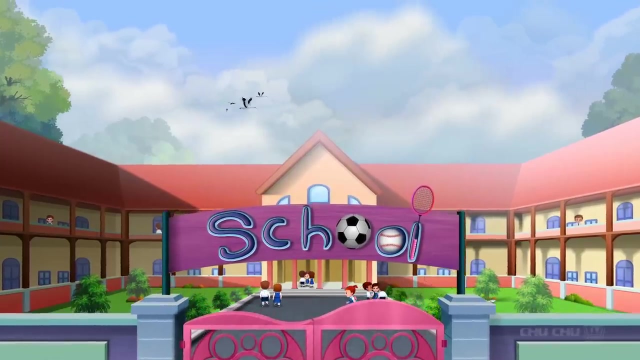 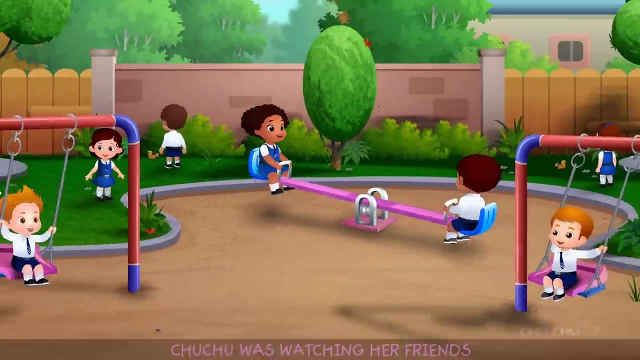 made the air fresh and clean, and now we are little super heroes, or so huh cha-cha was right. since all the children had made the neighborhood clean and green, they were little super heroes themselves. it was recess. choo-choo was watching her friends play on the playground. cha-cha. 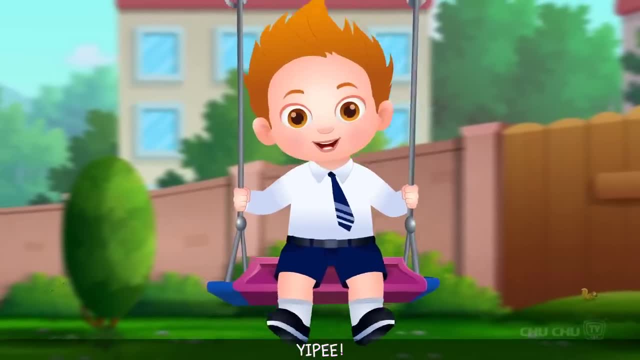 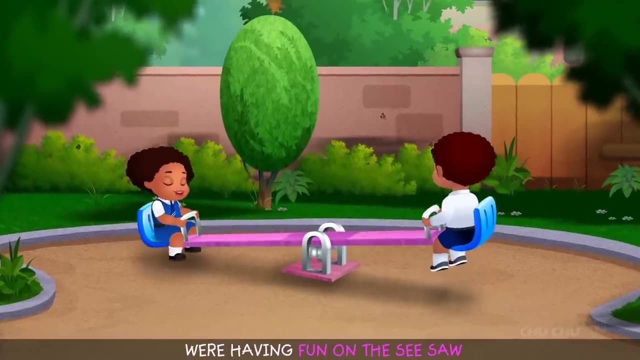 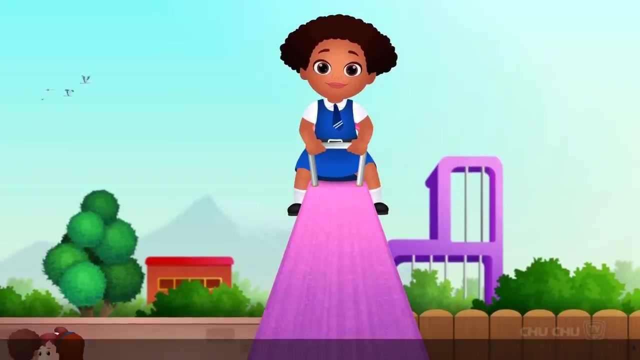 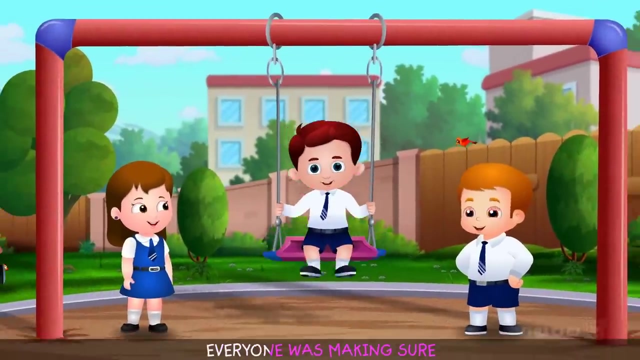 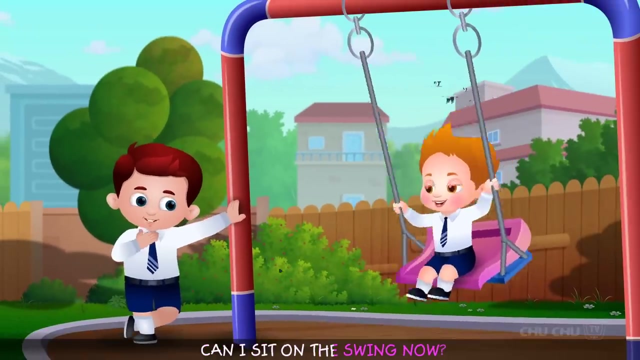 was on the swing. I'm having so much fun. chica and chiku, we're having fun on the seesaw up down. even though everyone was having fun, everyone was making sure that the other children had a turn. cha-cha, can I sit on the swing now? 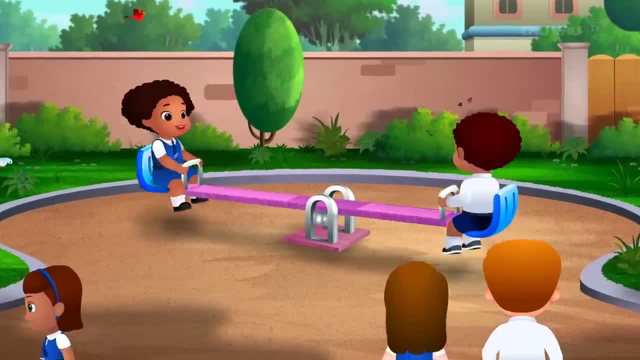 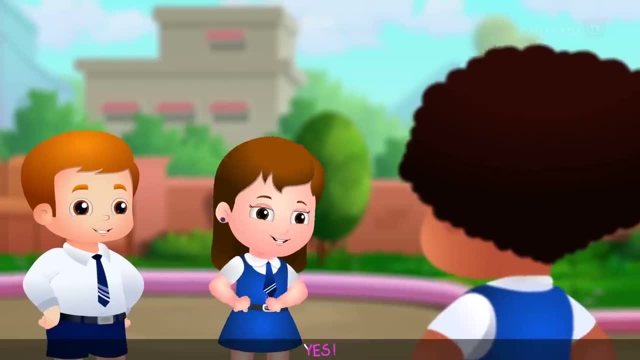 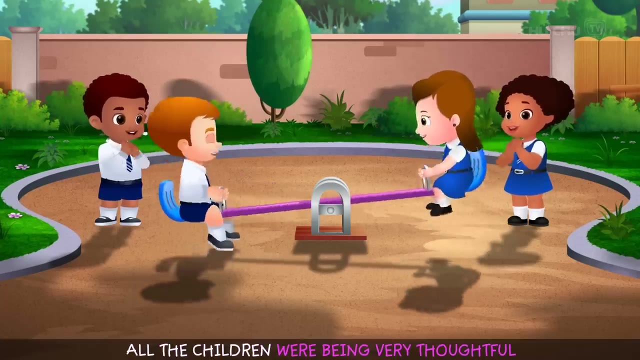 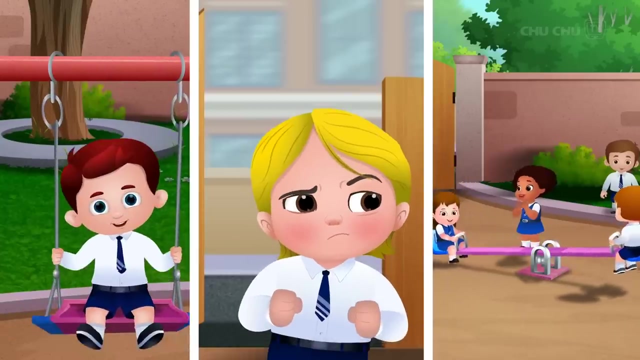 of course. would you like a turn on the seesaw? yes, please come and have a turn. all the children were being very thoughtful, but then, cussly, came into the playground. he stood up and said: I want to play with you, I want to play with you, I want to play with you. 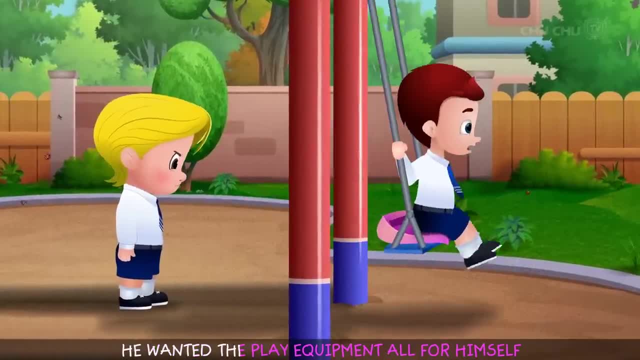 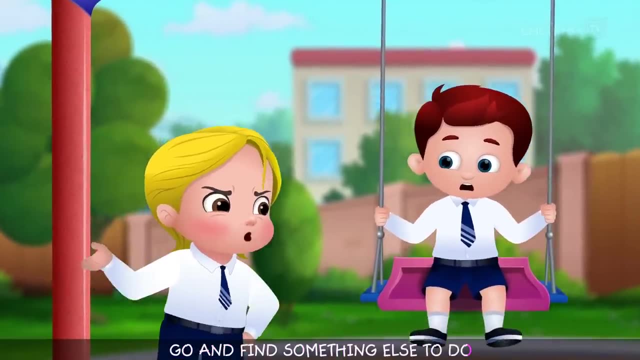 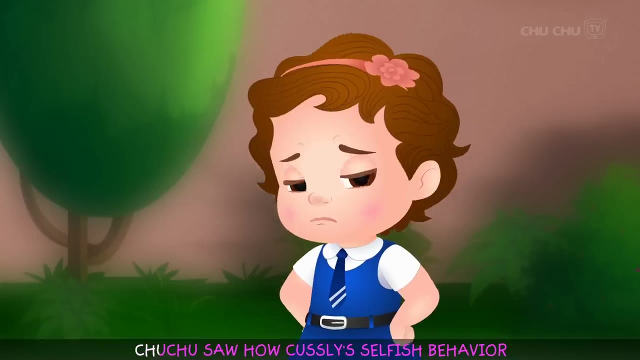 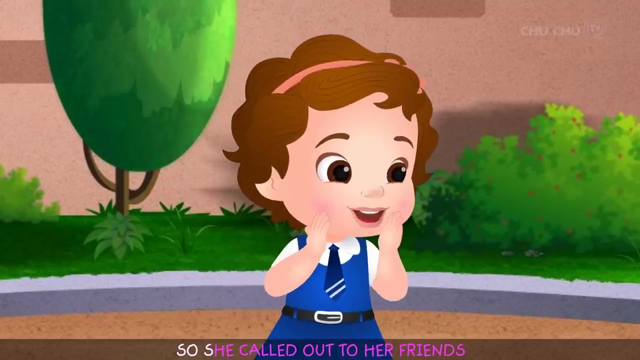 he started pushing the children. he wanted the play equipment all for himself. hey, get up, go and find something else to do. I want a swing, I want the seesaw for myself. choo-choo saw how cussly selfish behavior was ruining everyone's fun, so she called out to her friends: let's play a game. it's a game. 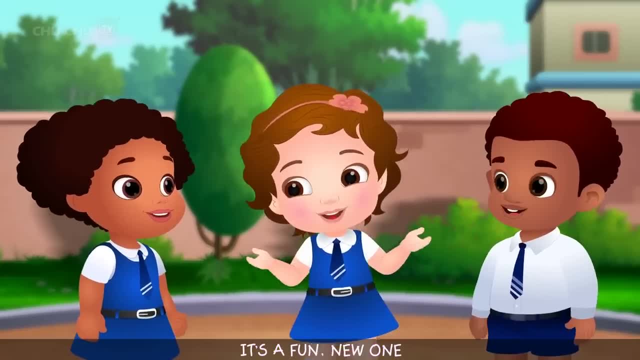 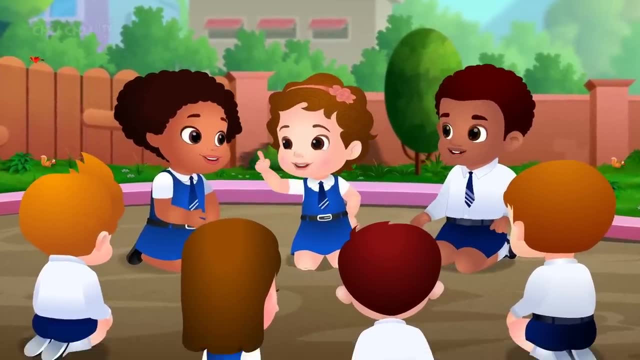 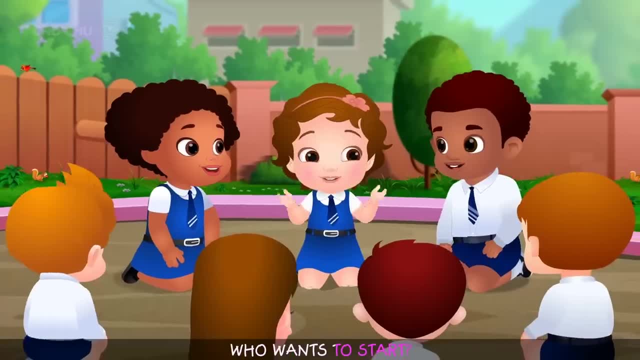 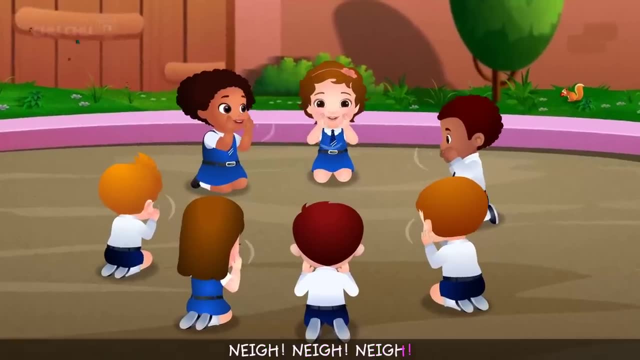 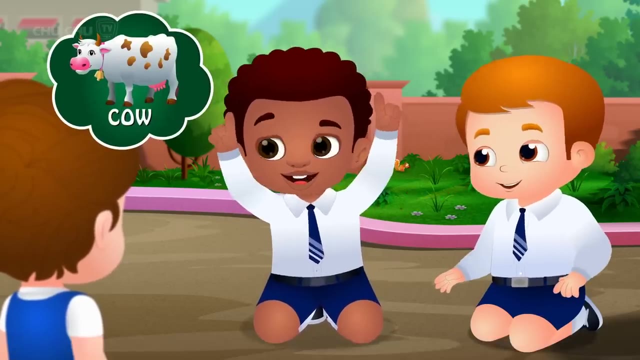 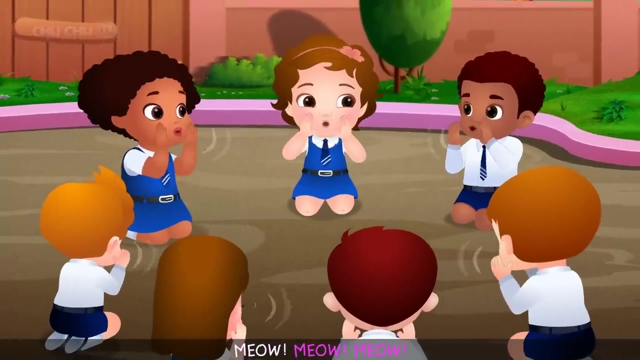 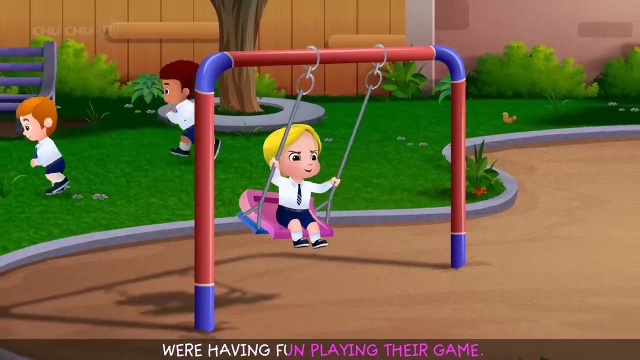 will make the sound that animal makes. who wants to start? I want you. it's my turn now. cow Moo Moo Moo, Cat Meow, Meow, Meow, While Choo Choo and the others were having fun playing their game. 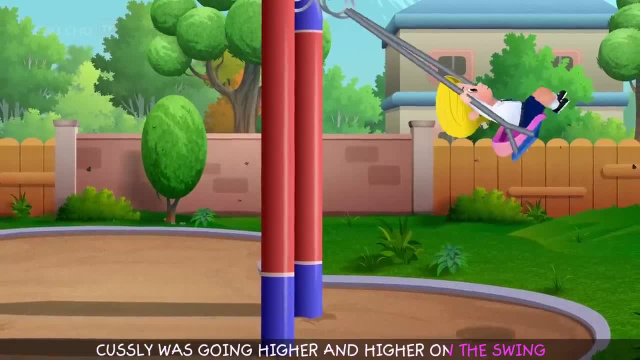 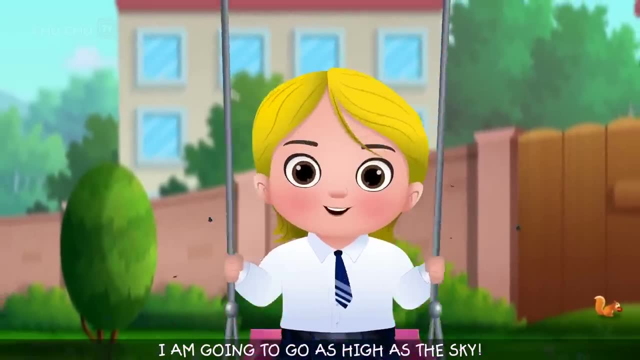 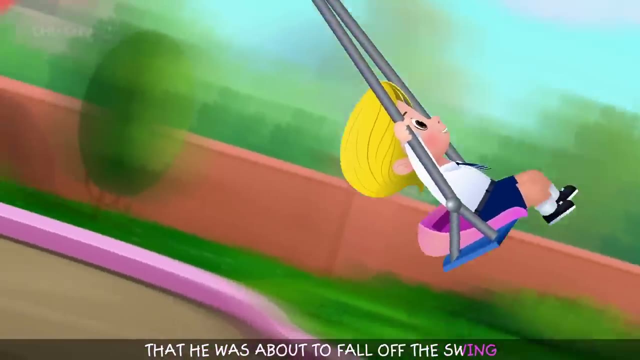 Custly was going higher and higher on the swing. Haha, I'm gonna go as high as the sky. Suddenly, Custly went so high that he was about to fall off the swing. Luckily Choo Choo saw him. Yikes. 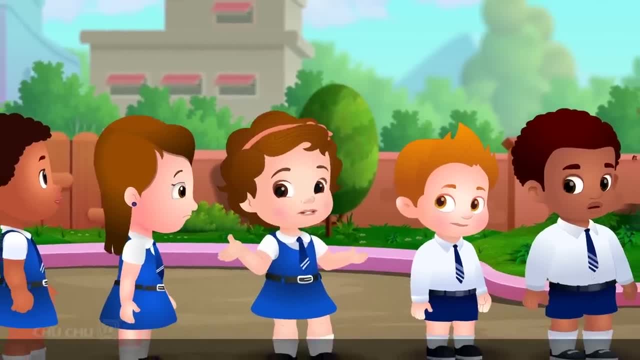 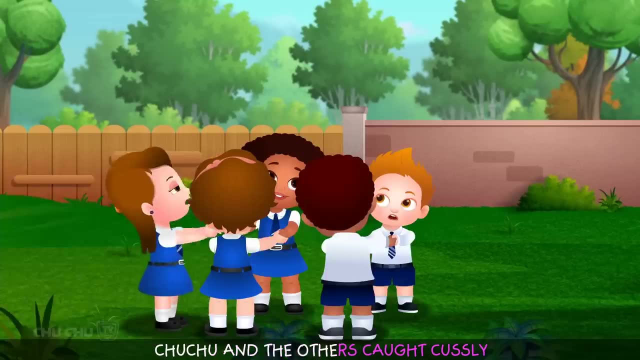 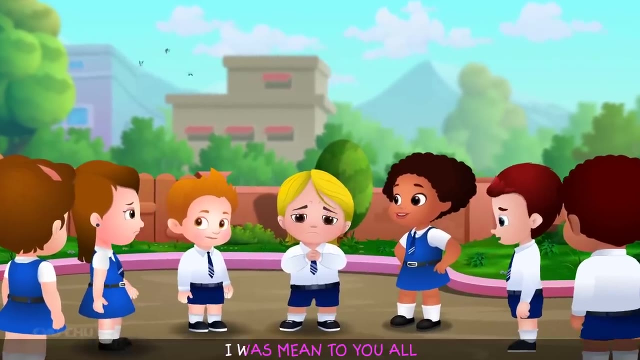 Huh, Friends, Custly is in trouble, Let's catch him before he falls. Choo Choo and the others caught Custly and saved him from really hurting himself. I was mean to you all, but you all still helped me. 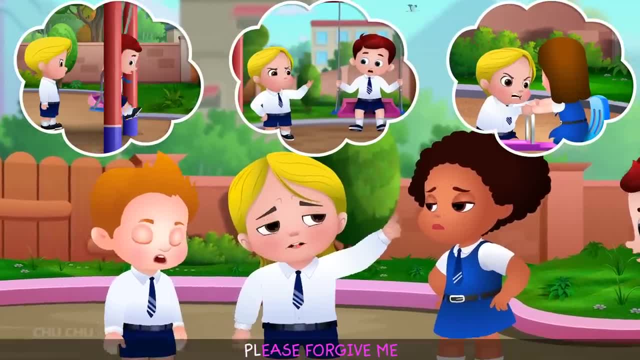 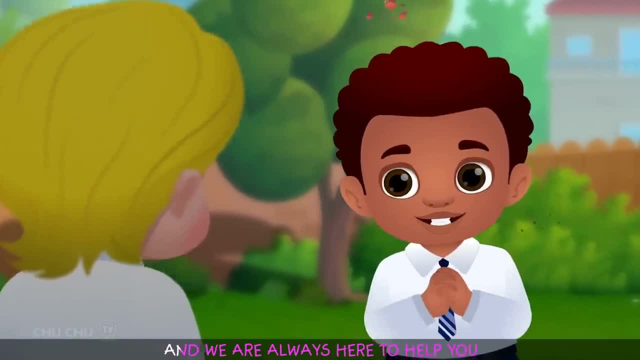 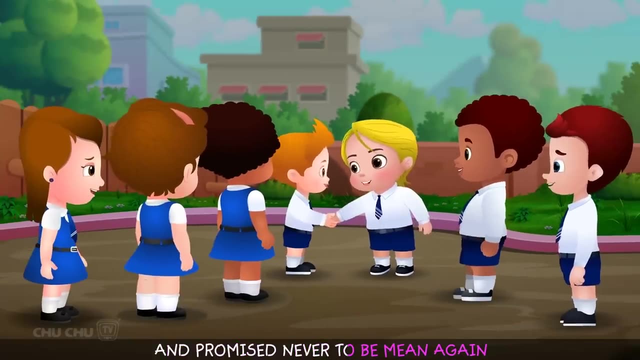 I'm sorry for my bad behavior. Please forgive me. Don't worry, Custly, We are your friends and we are always here to help you. Custly apologized to the children and promised never to be mean again. Everyone forgave him and invited him to join their group. 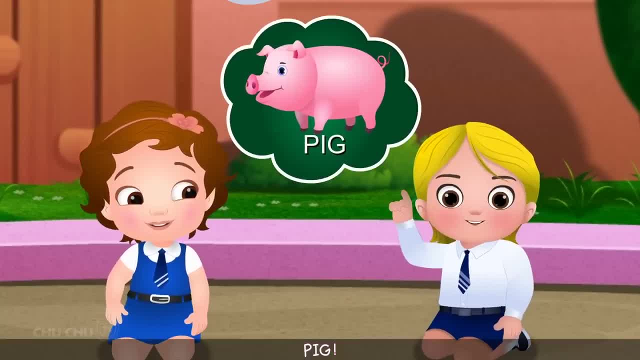 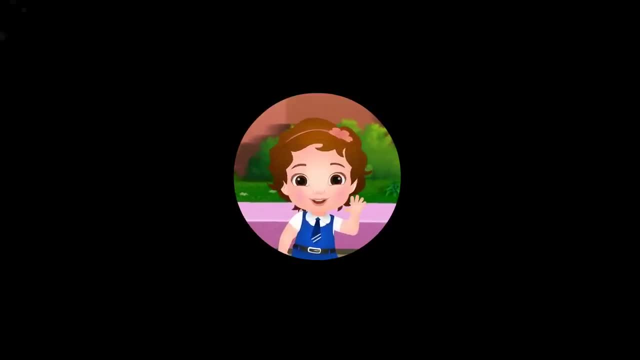 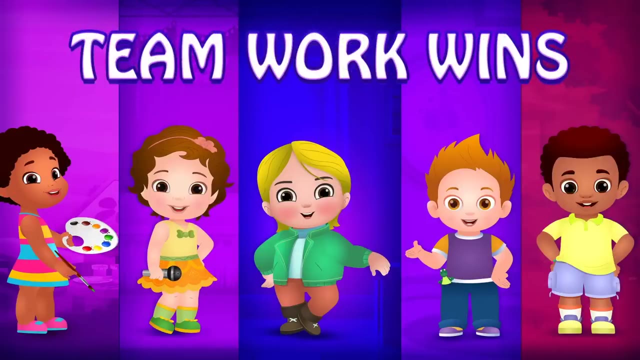 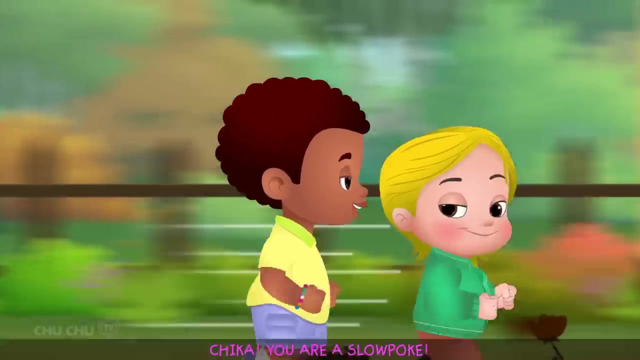 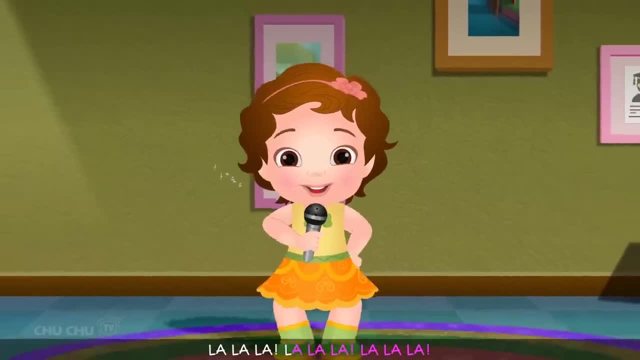 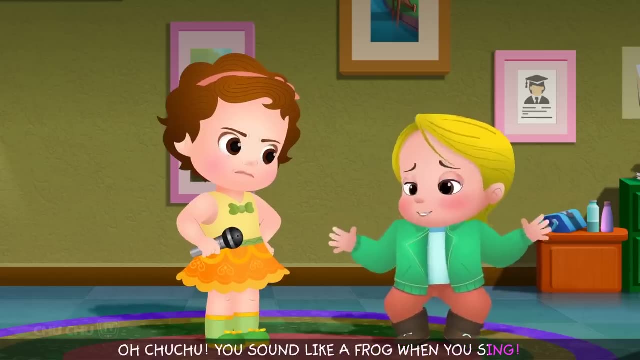 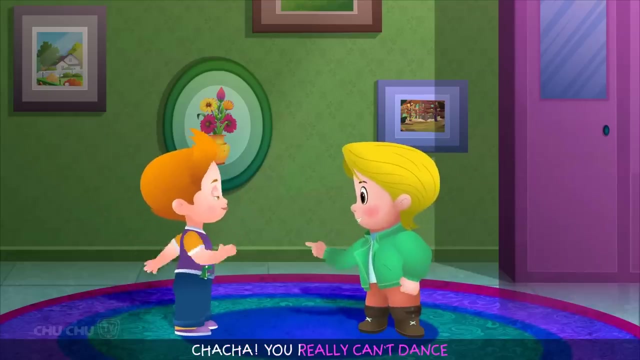 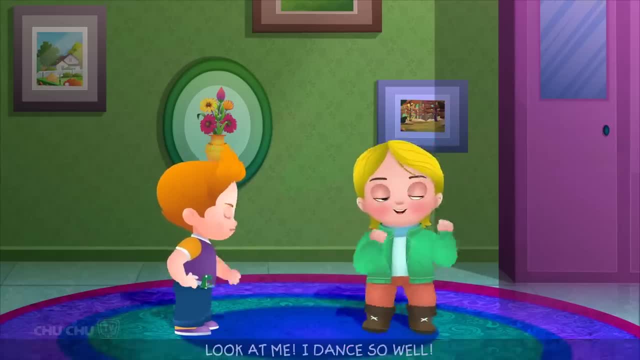 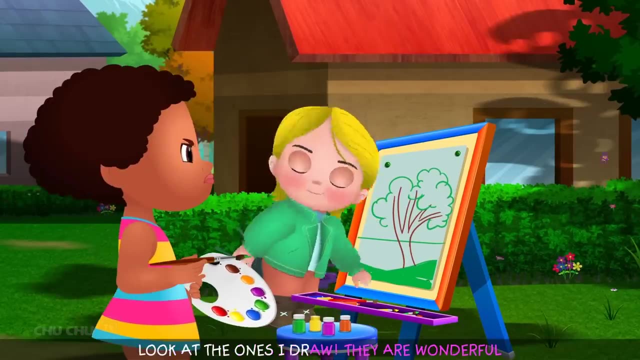 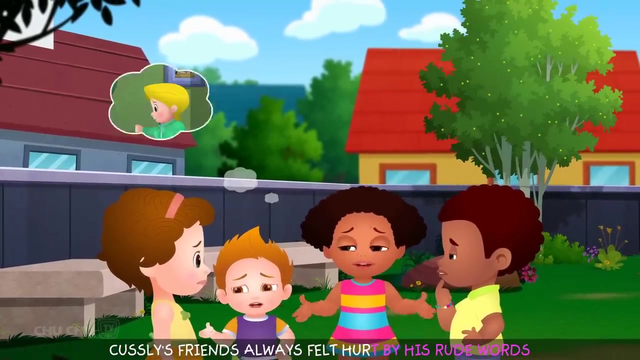 Look at me. I dance so well. Chiku, The pictures you draw look terrible. Look at the ones I draw. They are wonderful. Custly's friends always felt hurt by his rude words. I wish Custly wasn't so rude to us. 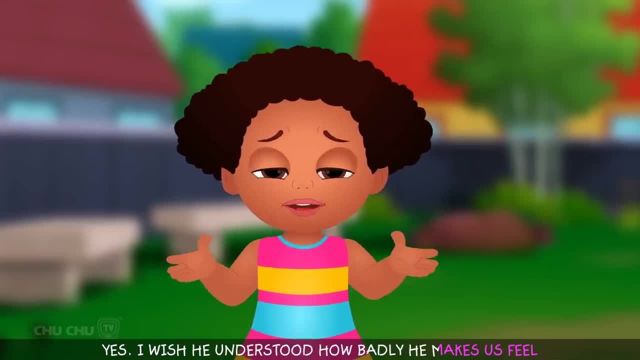 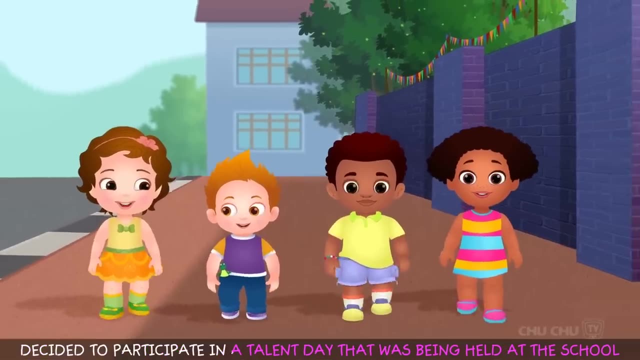 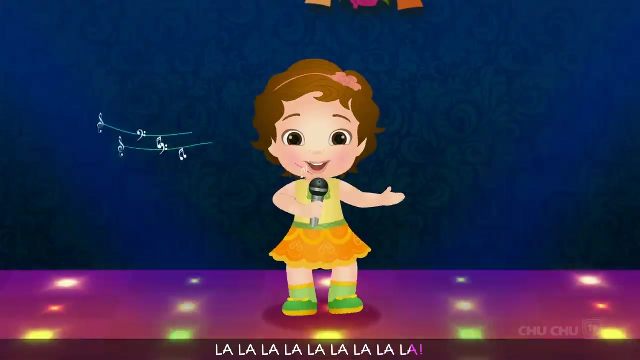 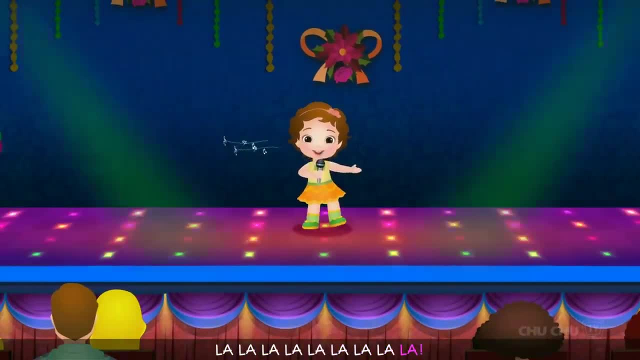 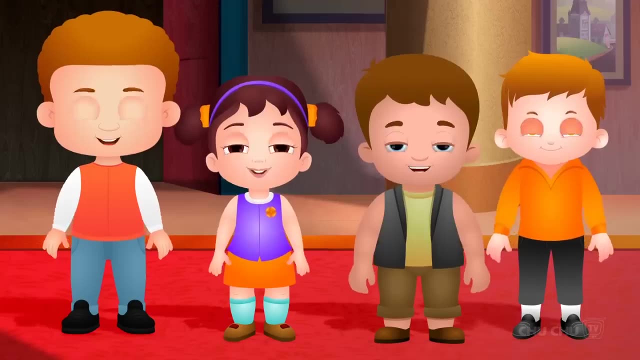 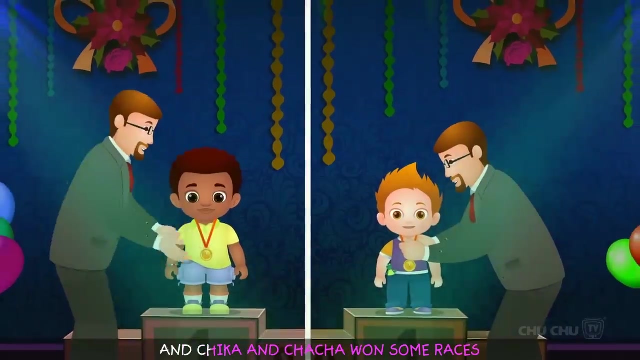 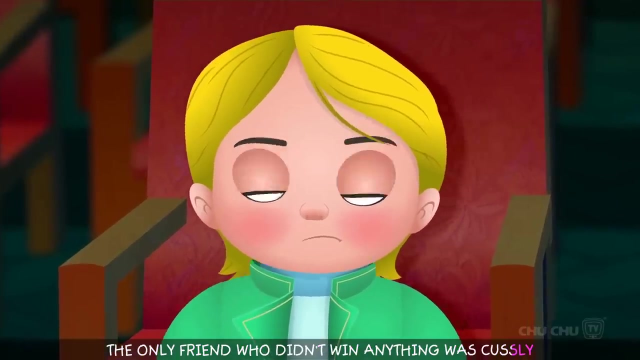 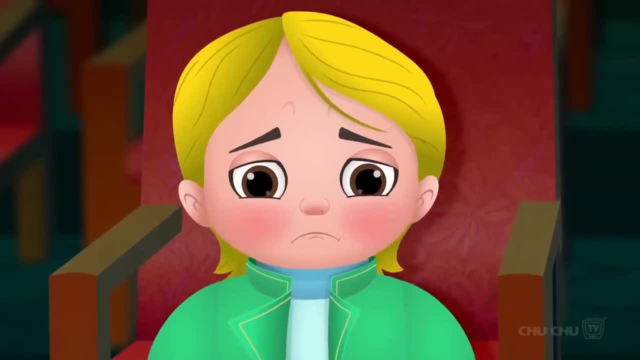 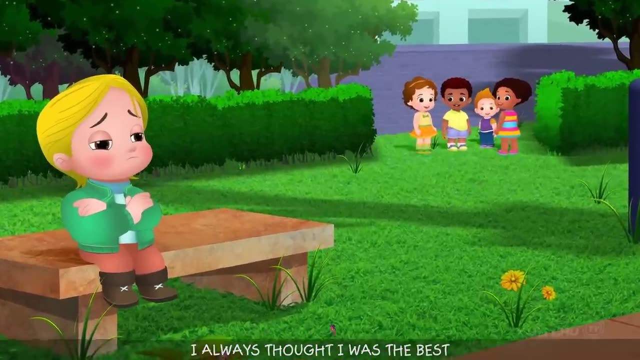 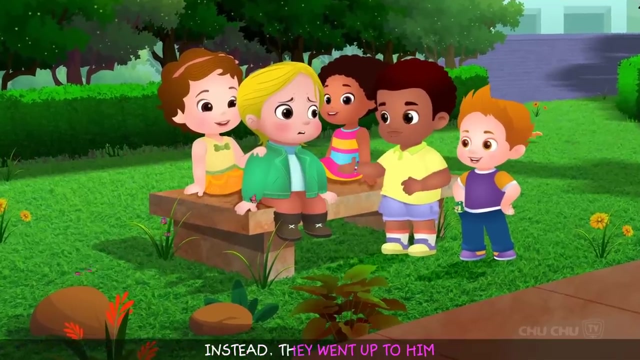 And he felt terrible about it. I'm the only one who hasn't won anything. I always thought I was the best, But Choo Choo and the others didn't make fun of Custly. Instead, they went up to him and tried to make him feel better. 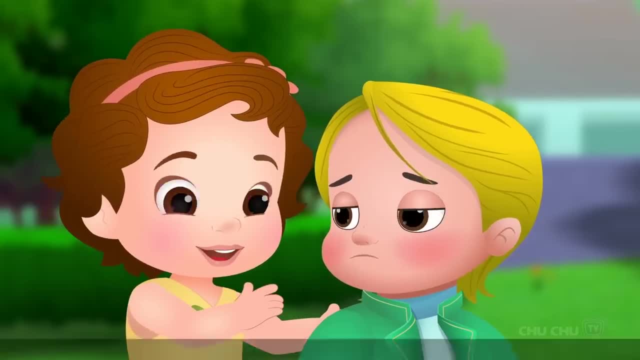 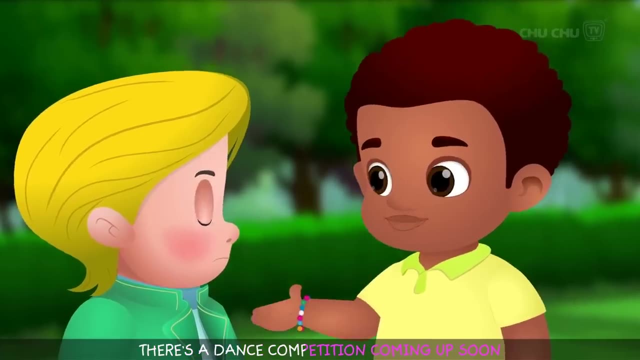 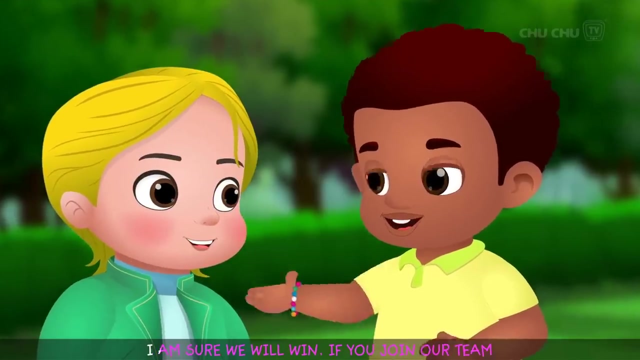 Don't lose hope, Custly. There are many more competitions that you can take part in. There's a dance competition coming up soon. We are participating in it. You're a good dancer. I'm sure we'll win if you join our team. 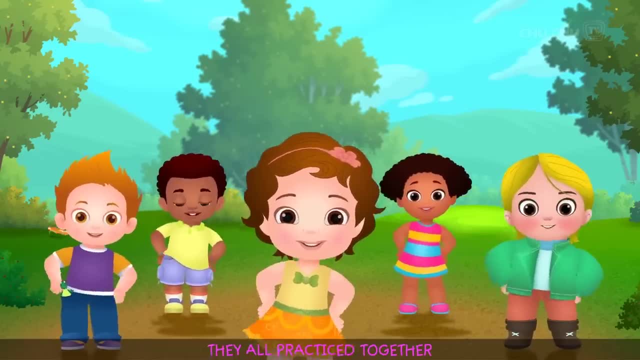 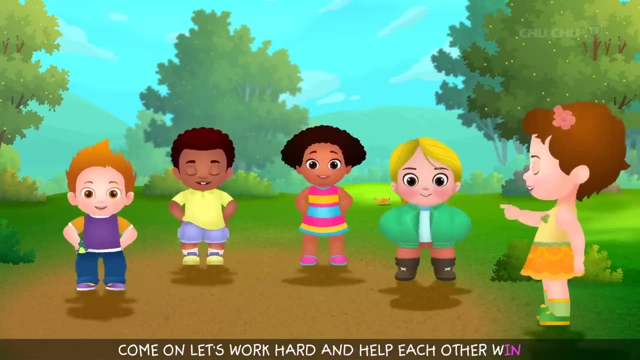 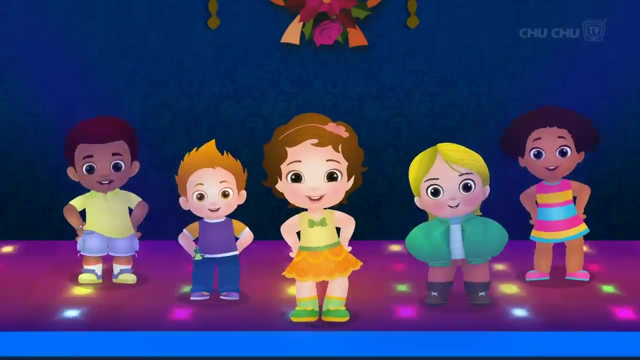 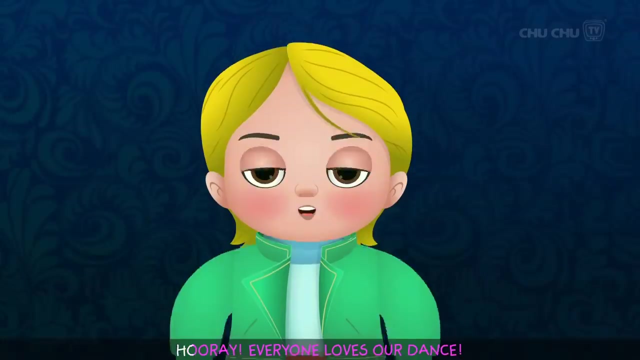 So Custly joined Choo Choo and the others. They all practiced together. Come on, Let's work hard and help each other win. Choo Choo and her friends stole the show during the dance competition. Hooray, Everyone loves our dance. 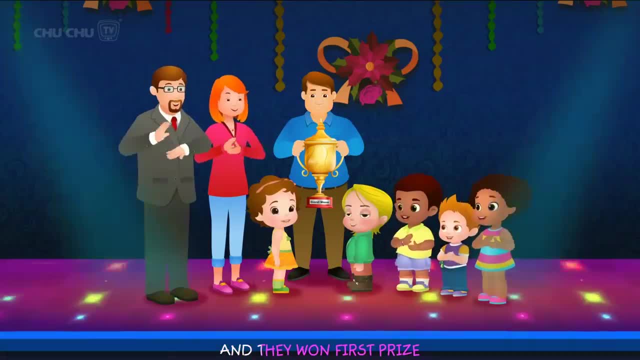 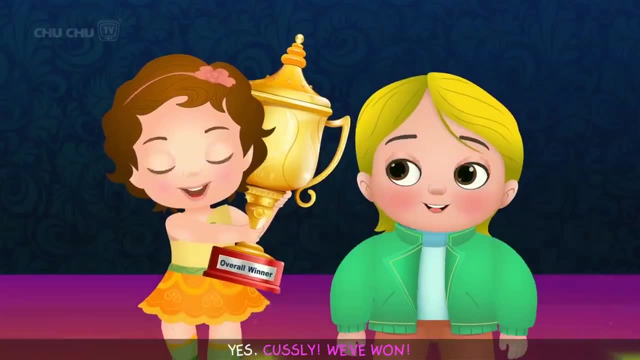 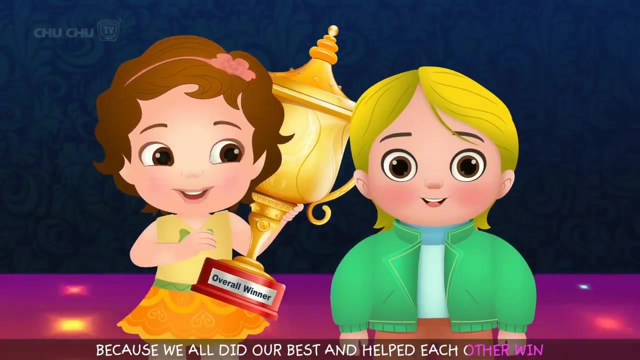 The team's dance was the best And they won first prize. Yay, Our team has won. Yes, Custly, We've won, Because we all did our best And helped each other win. That's what is so special about being a team. 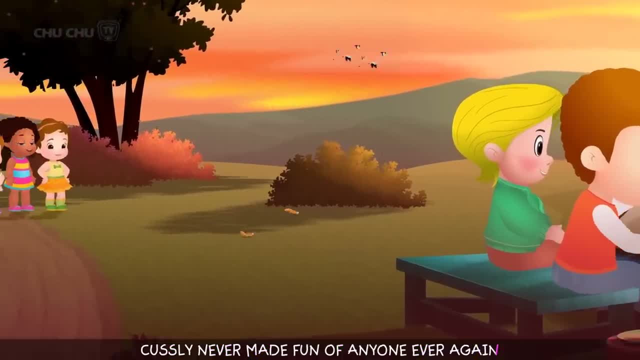 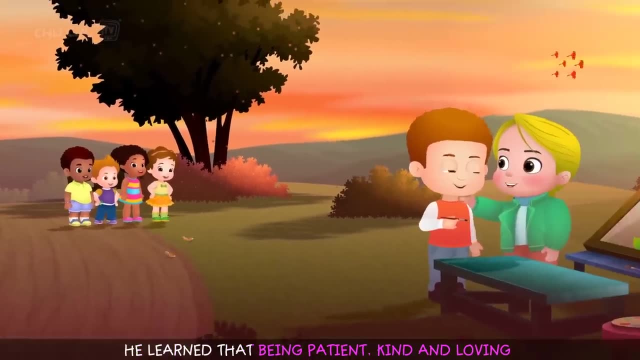 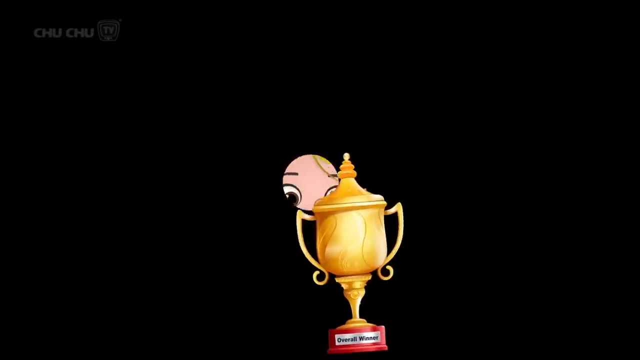 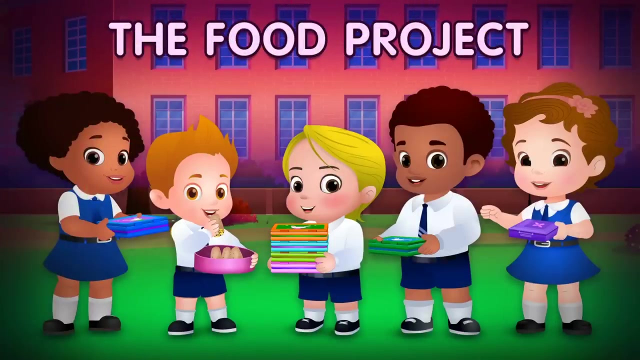 Custly, never made fun of anyone ever again. He tried to be more like Choo Choo by encouraging others. instead, He learned that being patient, kind and loving can bring out the best in others. It was in the lovely school district of Scottsdale. 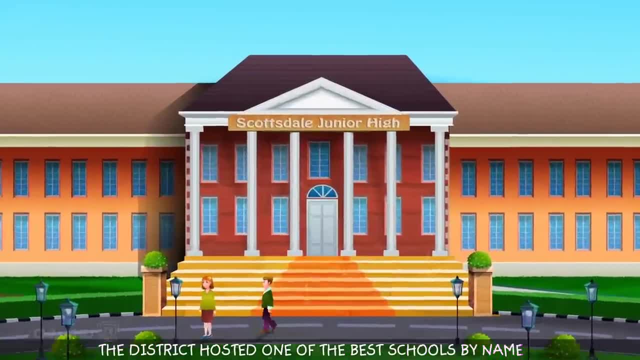 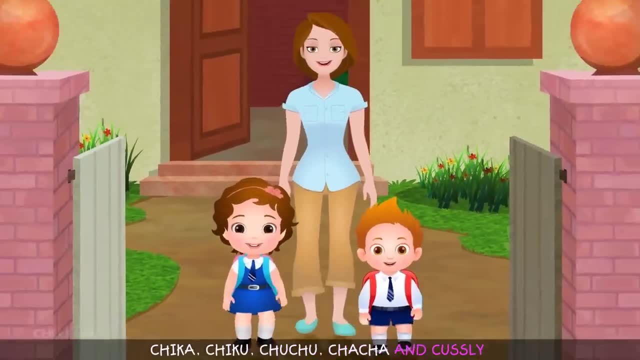 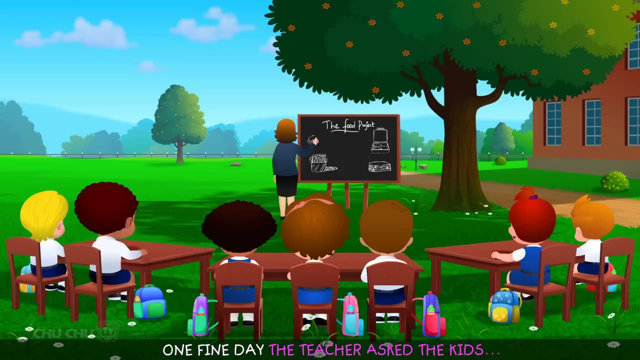 The district hosted one of the best schools by name: Scottsdale Junior High. Chica Chiku Choo Choo Cha Cha and Custly, who were the thickest of friends, went to the school One fine day. the teacher asked the kids 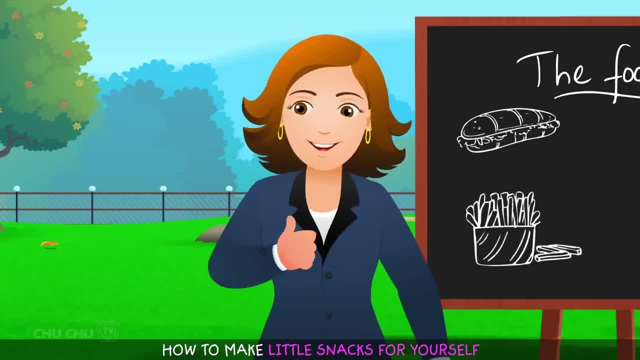 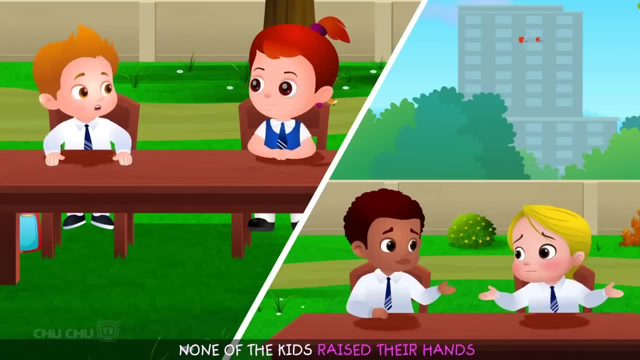 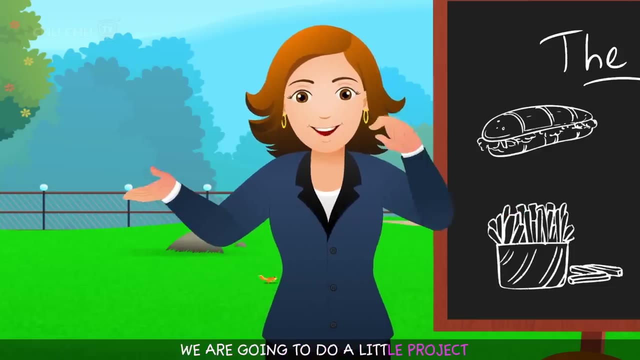 Little ones, those who know how to make little snacks for yourself, please raise your hands. None of the kids raised their hands. Aw, that's okay, We are going to do a little project. We are going to make our snack for tomorrow. 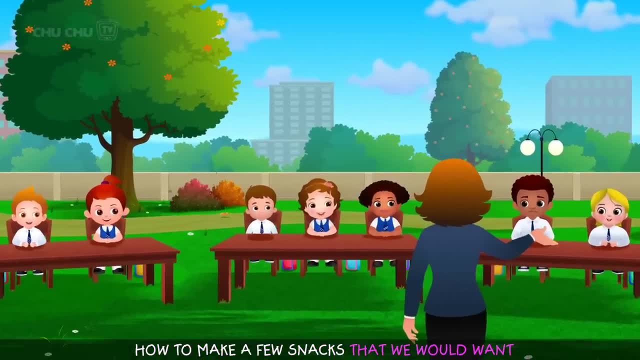 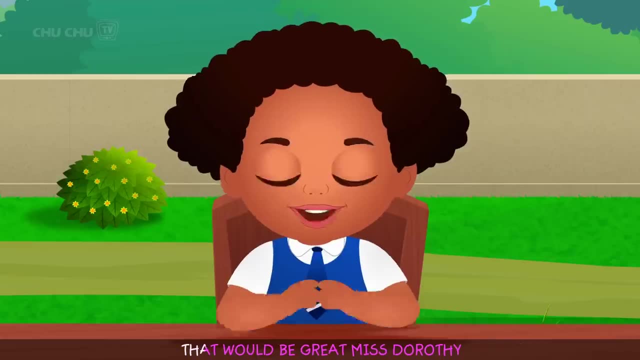 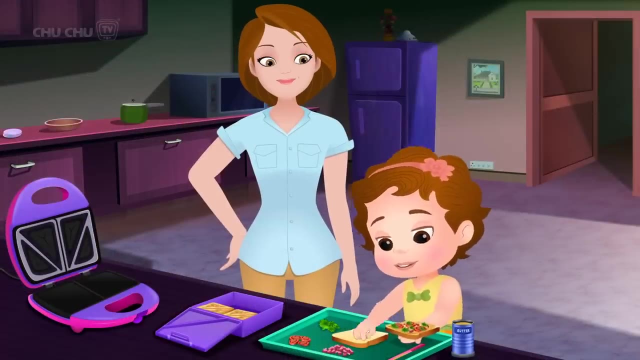 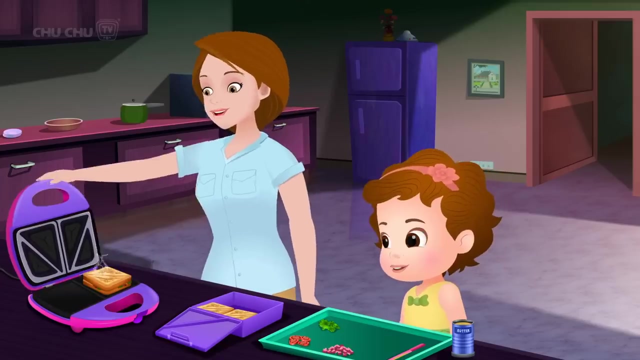 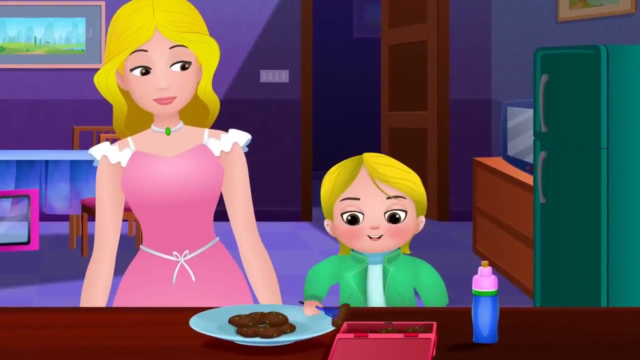 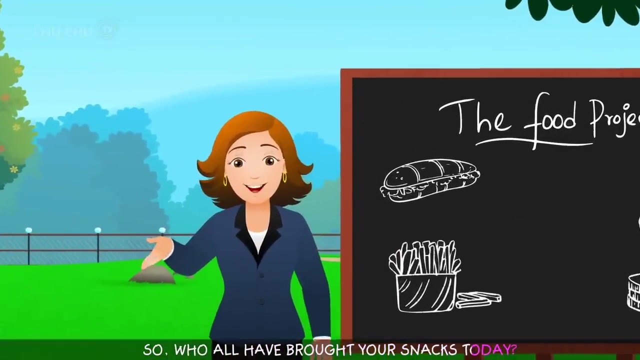 Ask your mom to teach you how to make a few snacks that we would want. I want you, little ones, to make your snacks tomorrow. That would be great, Miss Dorothy Sooo, who all have bought your own snacks for today. Except for Chiku and Chika, the others raised their hands. 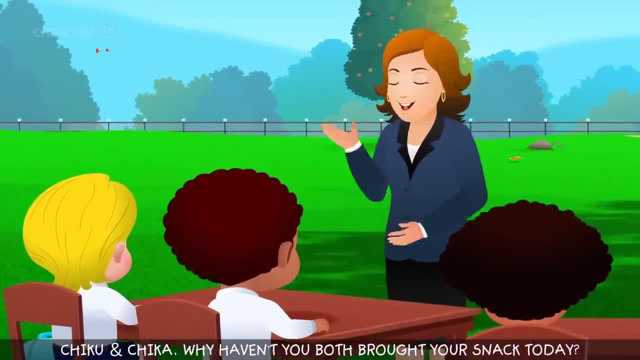 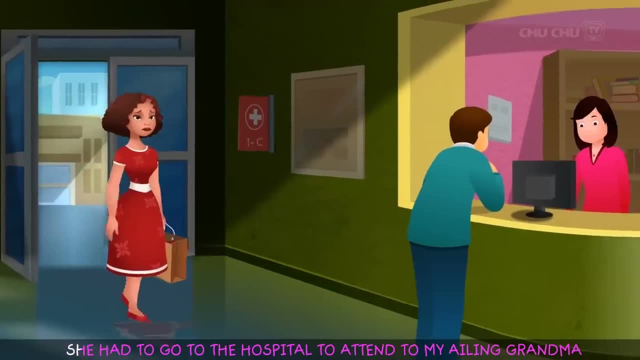 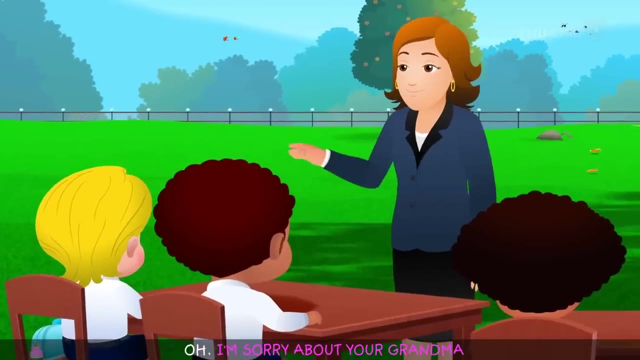 Chiku and Chika, why haven't you both brought your snack today? My mother was not home to make me my snack, Miss Dorothy. She had to go to the hospital to attend to my ailing grandma. Oh, I'm sorry about your grandma. 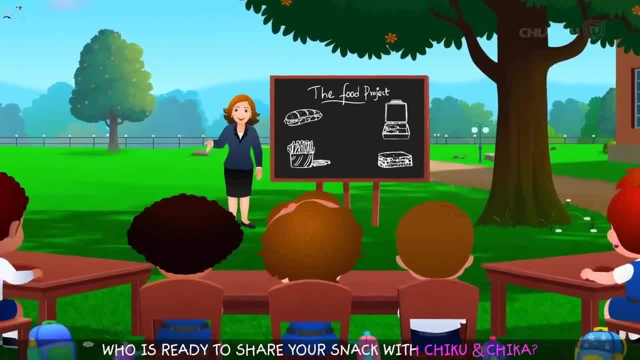 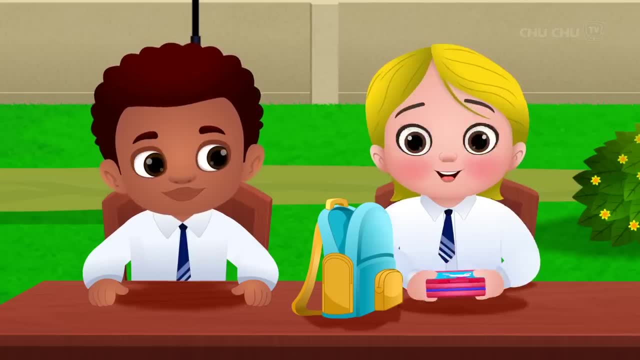 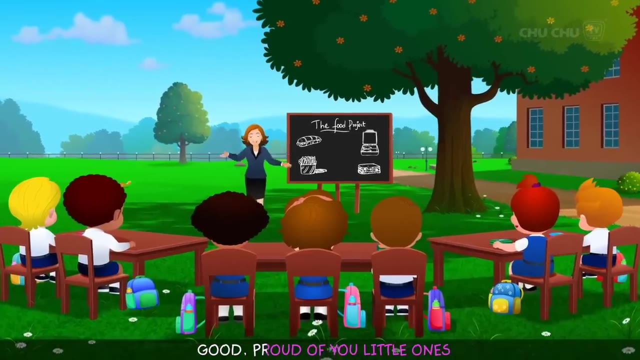 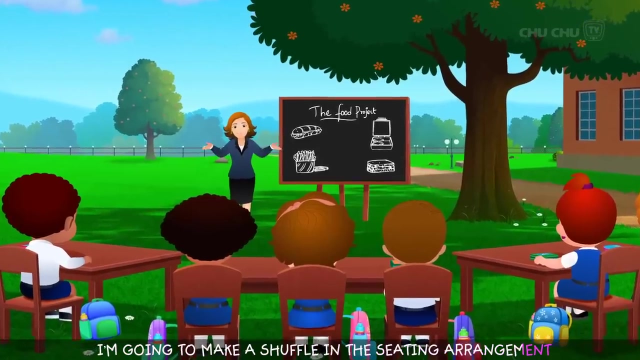 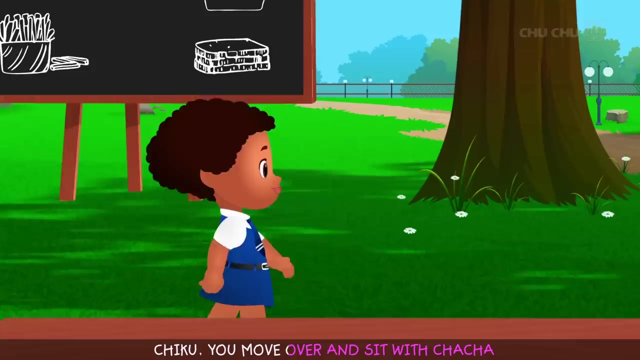 Class. who is ready to share your snack with Chiku and Chika? Good Proud of you, little ones. Listen, I'm going to make a shuffle in the seating arrangement. Sure, Miss Dorothy Chiku, you move over and sit with Cha-Cha. 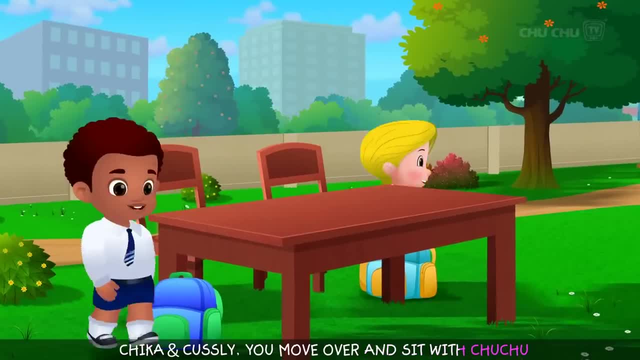 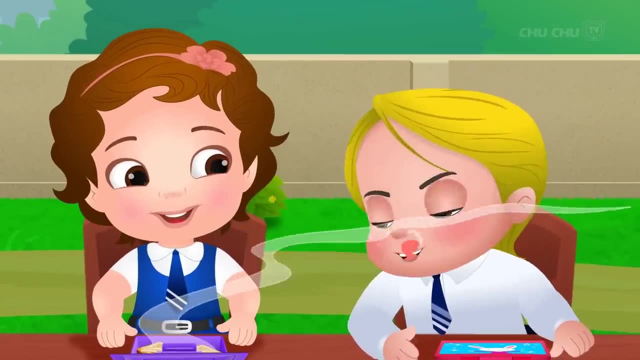 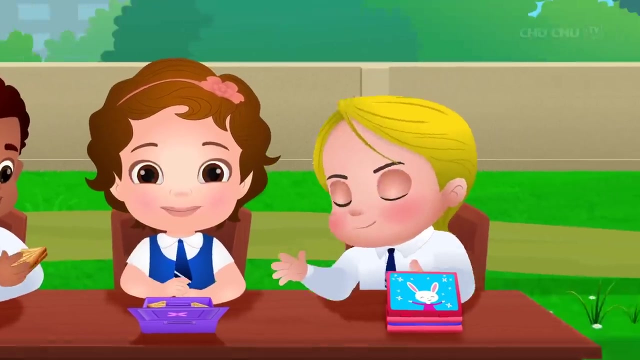 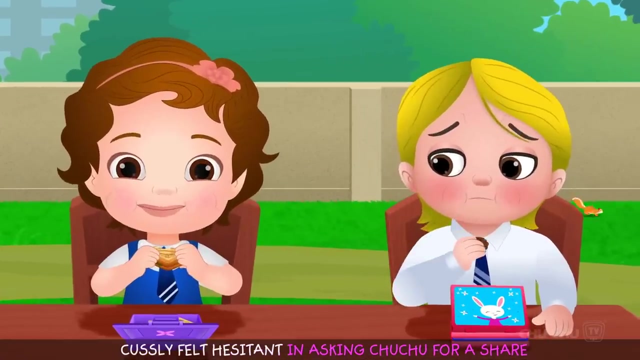 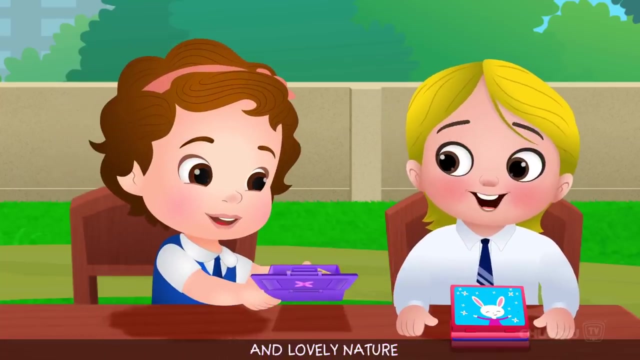 Chika and Custly. you move over and sit with Chika And Chuchu. Since Custly did not offer to share his snack with Chika, Custly felt hesitant in asking Chuchu for a share. Her soft gentle and lovely nature made her offer a share to Custly. 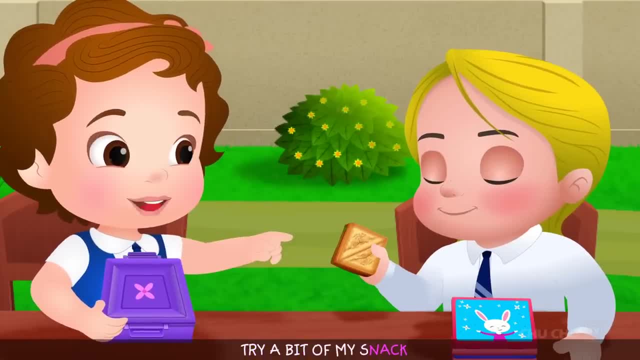 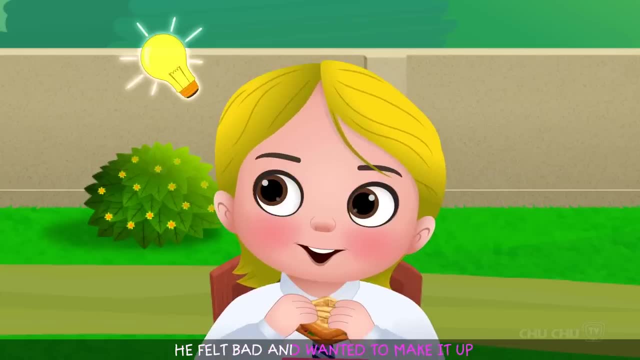 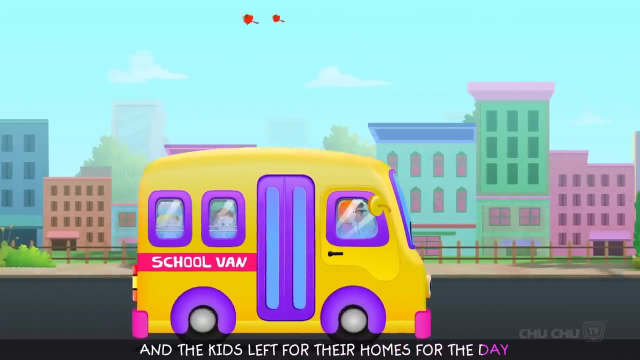 You would love this. Custly, Try a bit of my snack. Custly felt ashamed for what he had done. He felt bad and wanted to make it up. The school bell rang and the kids left for their homes for the day. 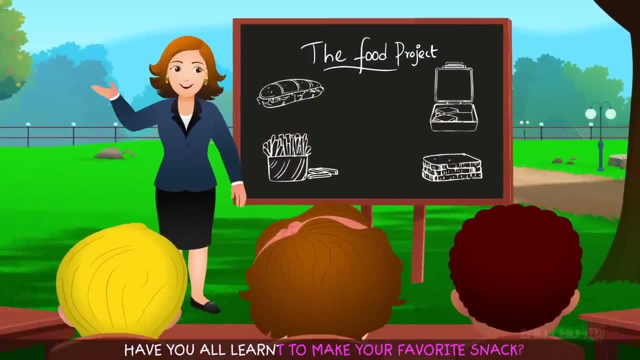 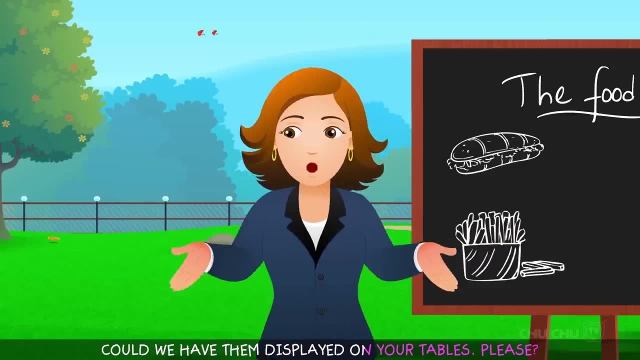 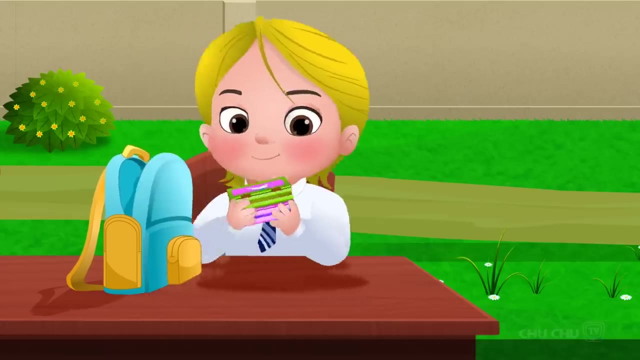 So little ones? have you all learned to make your favorite snack? Yes, Miss Dorothy, Could we have them displayed on your tables, please? All the kids put their preparations on the table. Custly had put four boxes on his table. 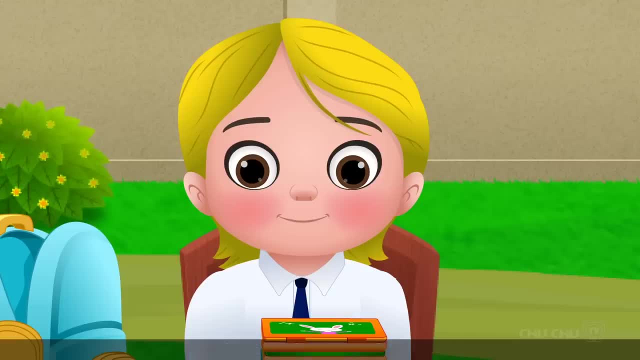 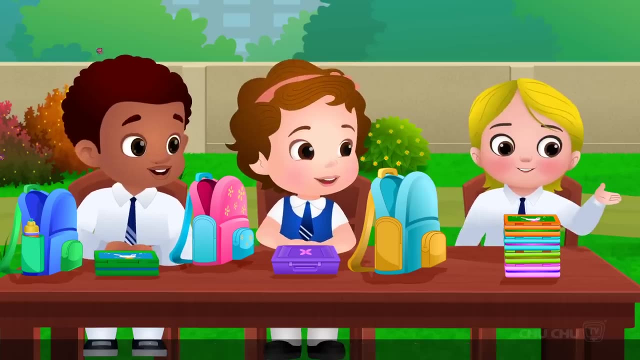 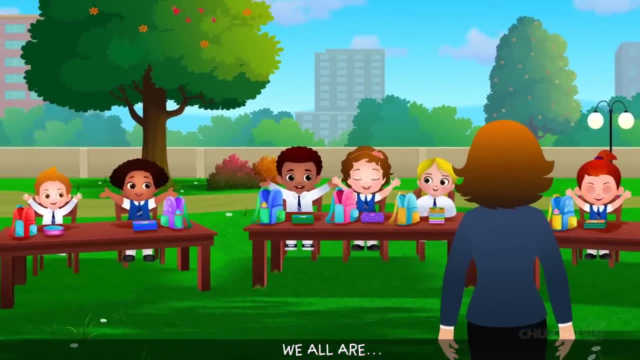 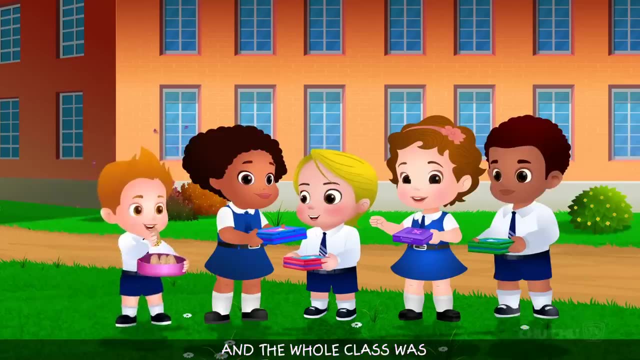 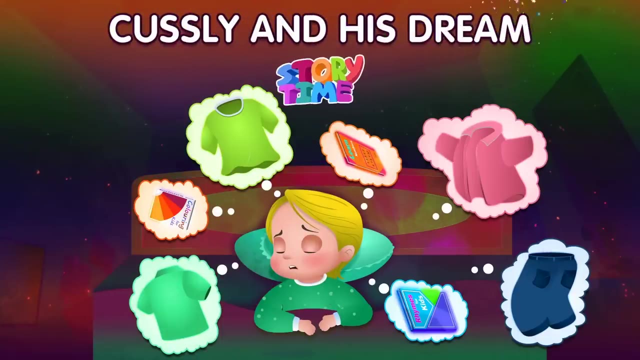 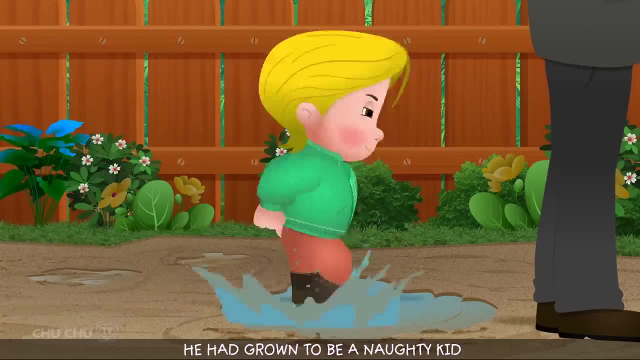 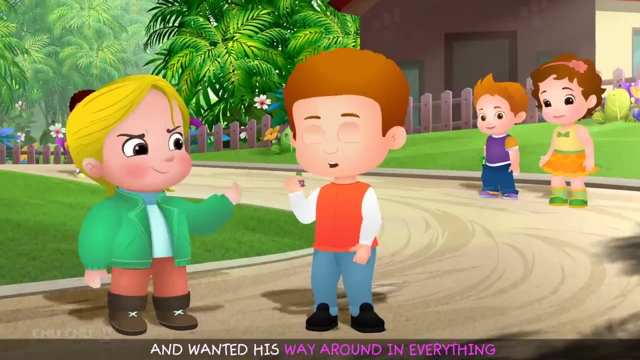 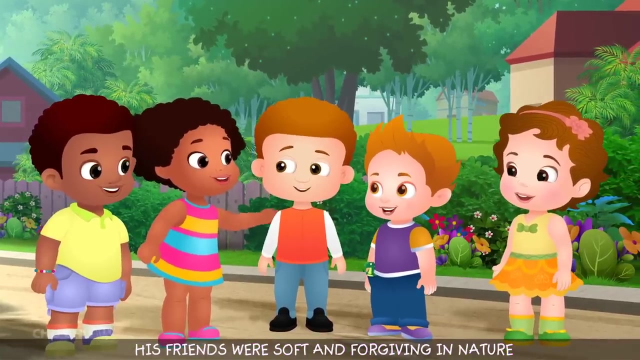 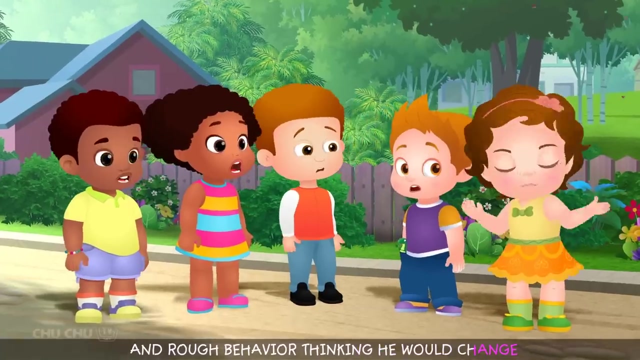 He had grown to be a naughty kid. He pulled out his pants and put them on the table. He pushed his friends down, bullied them and wanted his way around in everything. His friends were soft and forgiving in nature. They just put up with his harsh and rough behavior, thinking he would change. 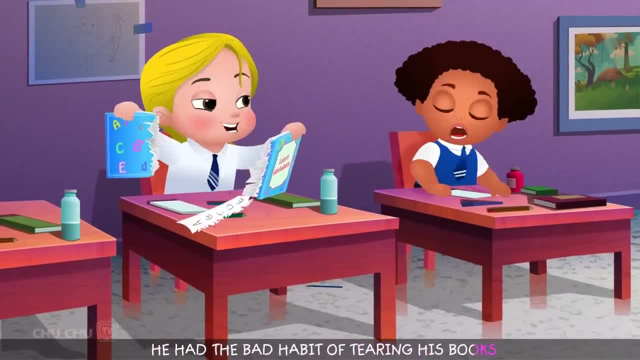 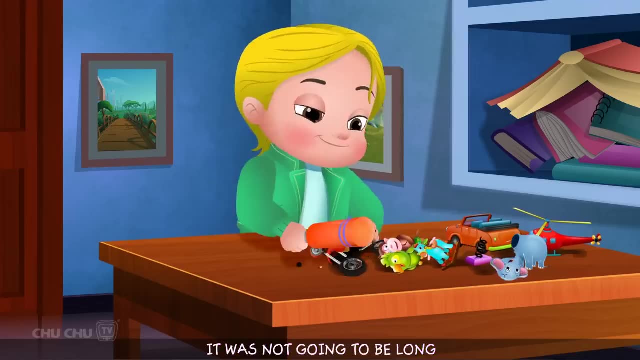 He had the bad habit of tearing his books, throwing his clothes and breaking his toys. He had the bad habit of throwing his clothes and breaking his toys. It was not going to be long before someone taught him a lesson. It was not going to be long before someone taught him a lesson. 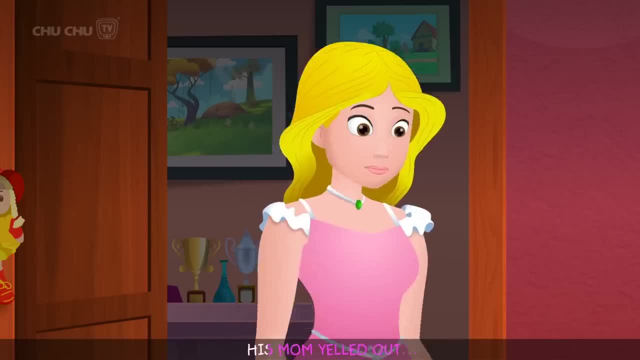 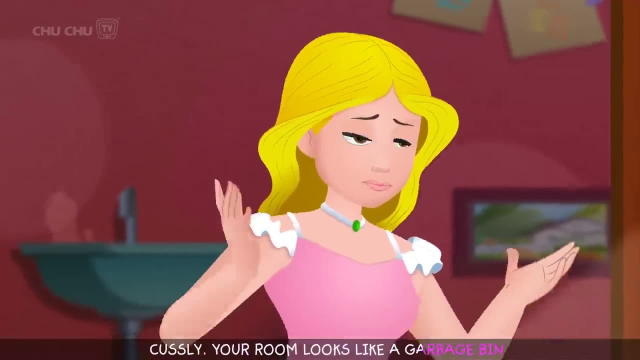 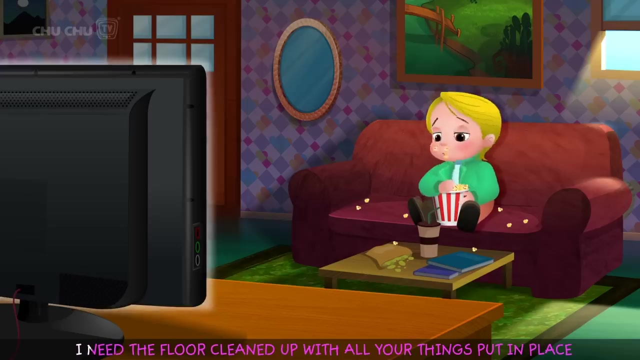 It was a nice sunny day. His mom yelled out. His mom yelled out Custly. Your room looks like a garbage bin. Your clothes, toys and books are all over the floor. I need the floor cleaned up with all of my clothes. 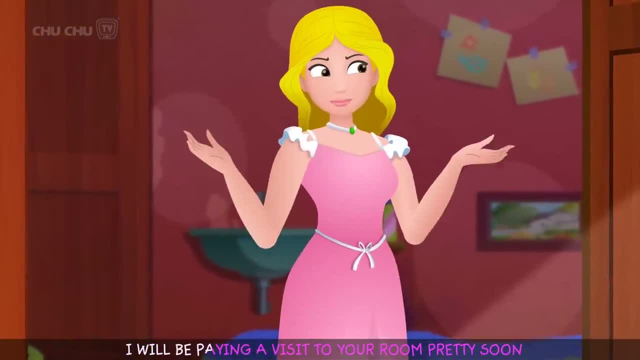 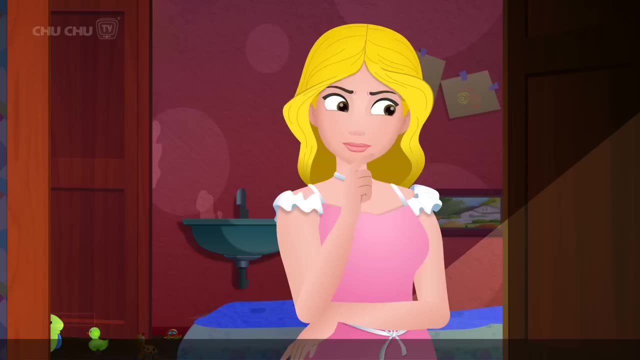 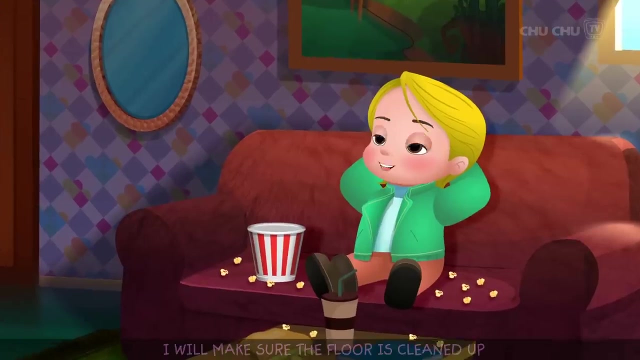 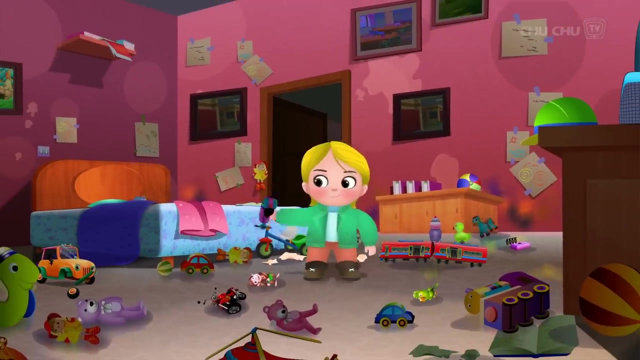 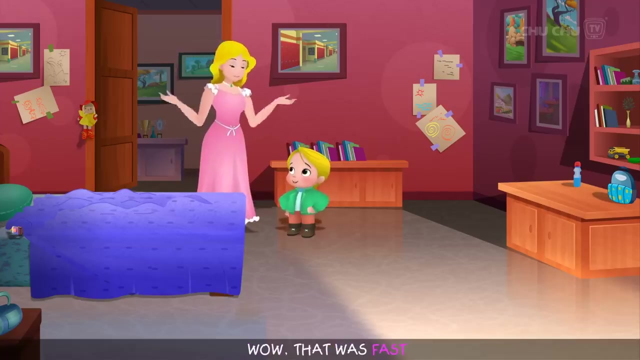 your things put in place. I will be paying a visit to your room pretty soon. you don't want to be grounded, do you? did you hear me? yeah, yeah, loud and clear. I'll make sure the floor is cleaned up. Wow, that was fast. this does not look. 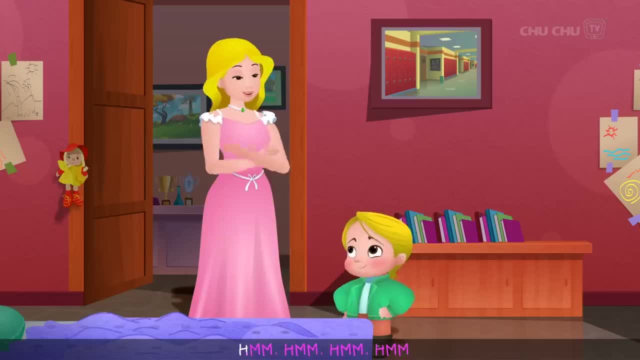 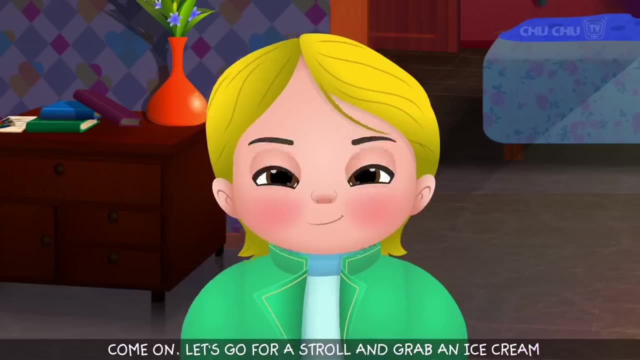 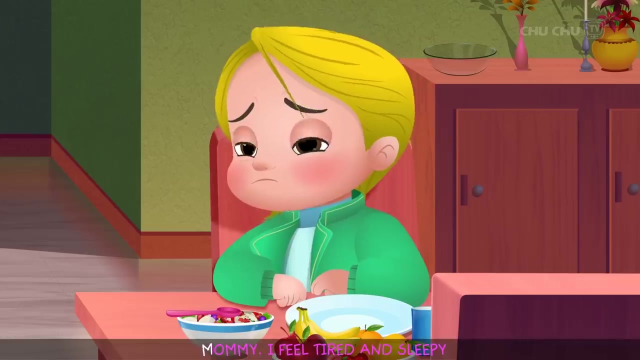 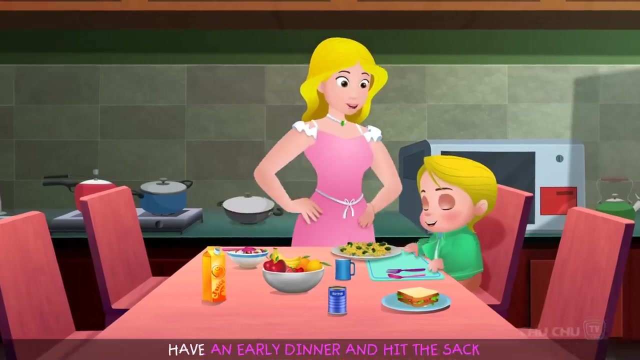 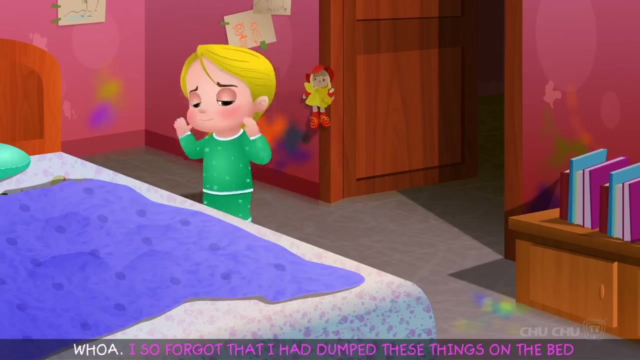 like your room. good job, come on, let's go for a stroll and grab an ice cream. it's a treat for your hard work. mommy, I feel tired and sleepy. dinner is ready. have an early dinner and hit the sack. yeah, okay, whoa, I so forgot that I had dumped these. 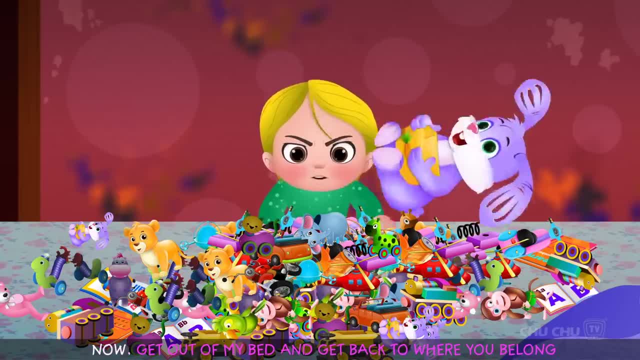 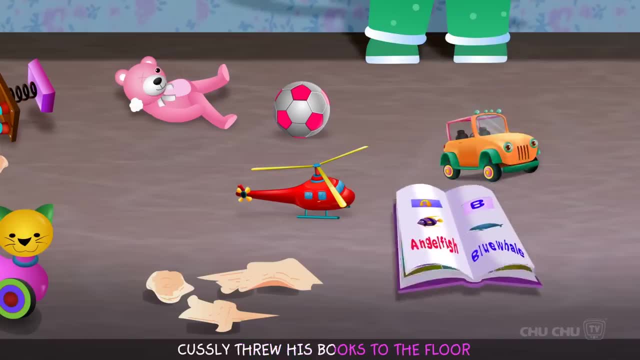 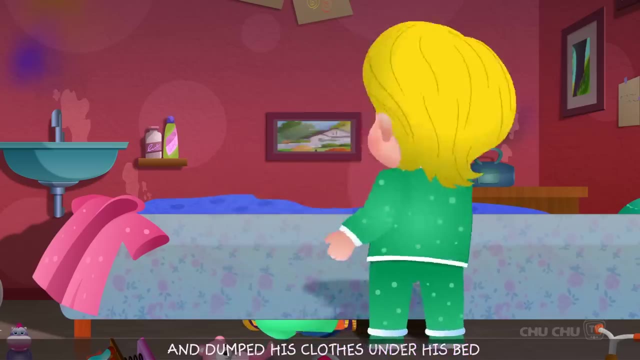 things on the bed. now get out of my bed and get back to where you belong. you cusley threw his books to the floor, he tossed his toys around and dumped his clothes under his bed. now that my bed is cozy, let me put off the light and go to 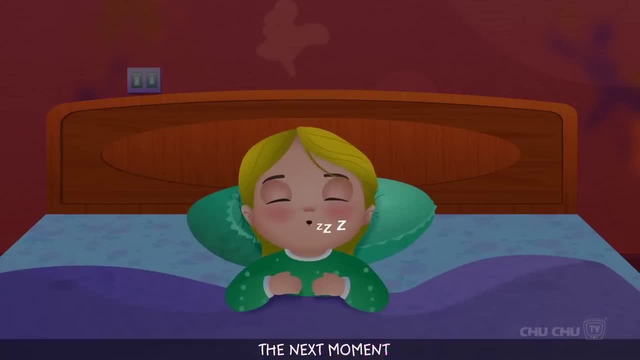 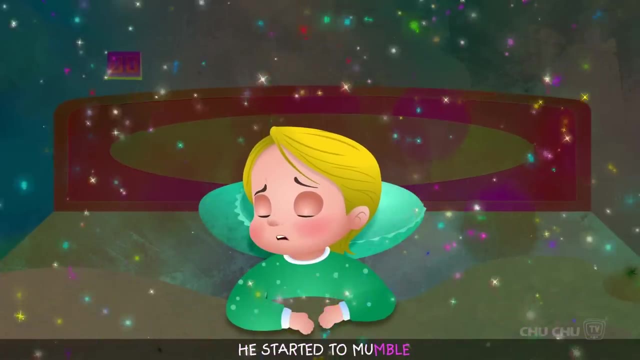 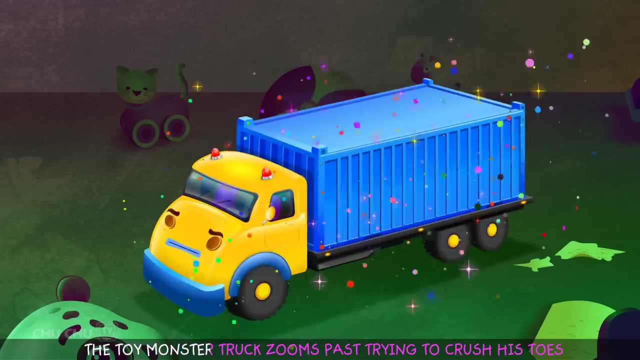 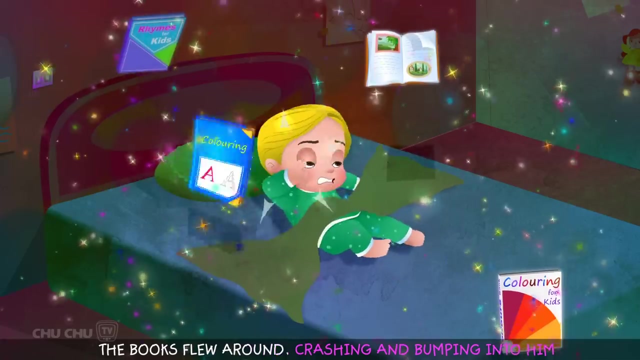 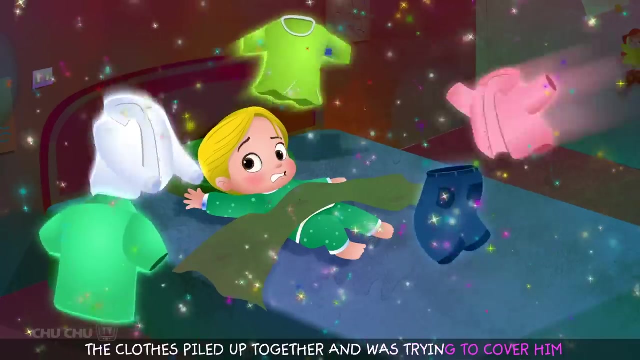 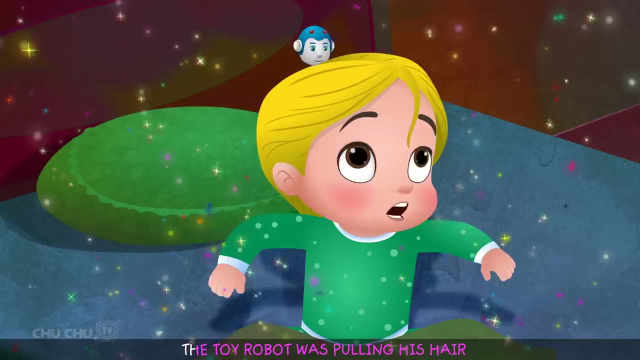 sleep. the next moment cusley was deep in sleep and was snoring away to glory. he started to mumble, he started to toss and turn in his sleep the toy monster truck trying to crush his toes. the books flew around, crashing and bumping into him. the clothing piled up together and was trying to cover him. the toy robot was. 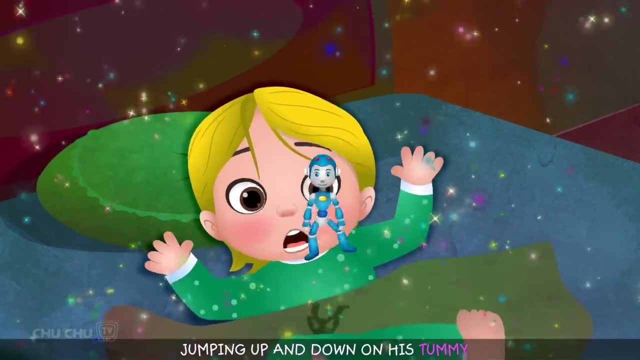 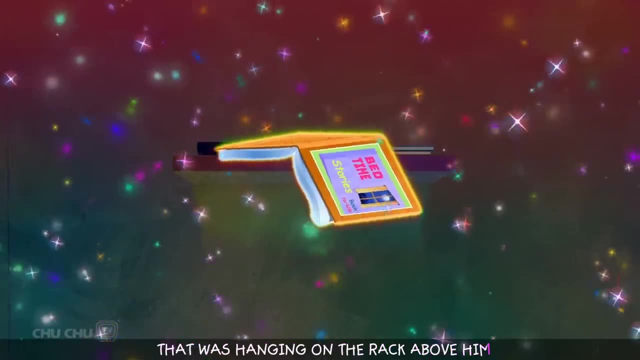 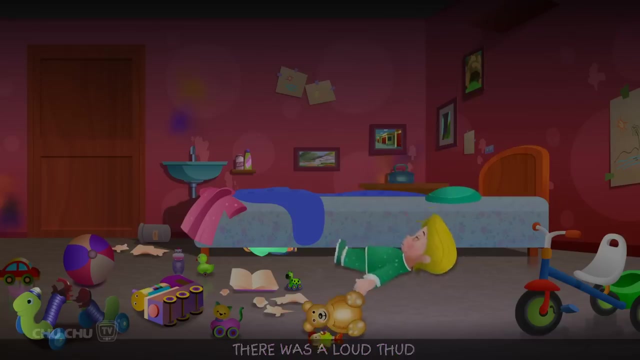 pulling his hair, jumping up and down on his tummy. Finally, the giant storybook that was hanging on the rack above him crashed onto his head with a bang. There was a loud thud. Custly had rolled off the bed and was on the floor. 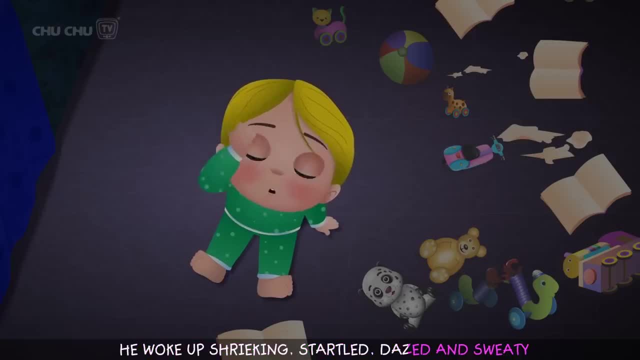 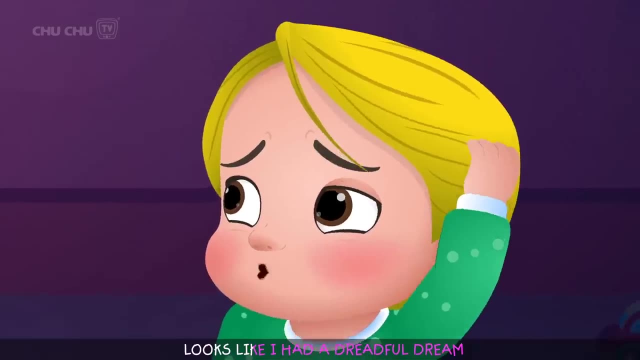 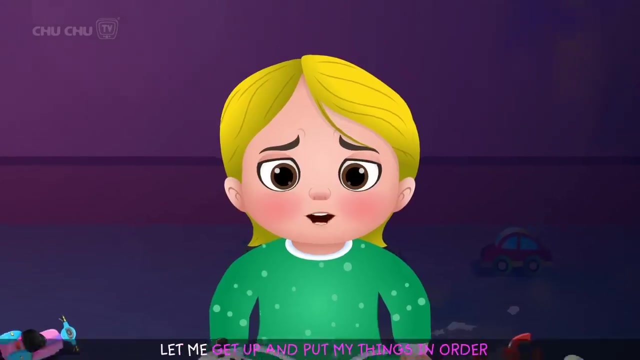 He woke up shrieking, startled, dazed and sweaty. Whoa, What was that? Looks like I had a dreadful dream. It was more of a nightmare. Let me get up and put my things in order. Let me put them where they belong. 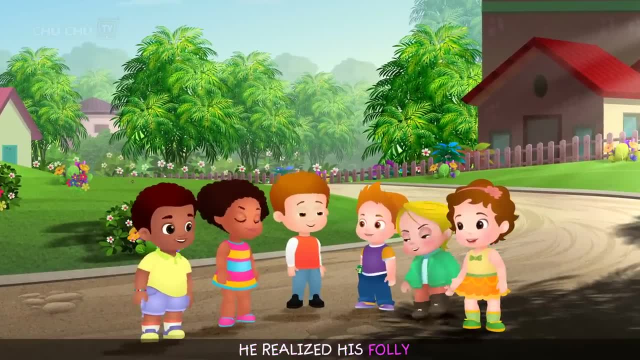 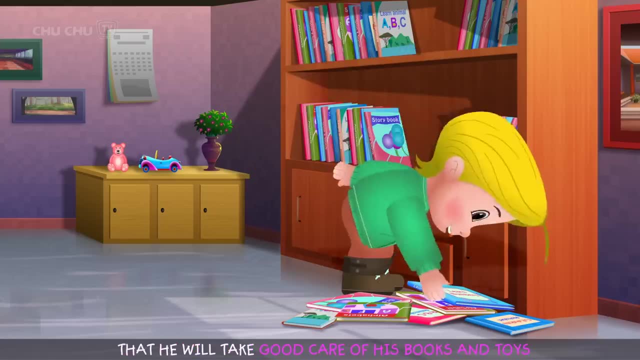 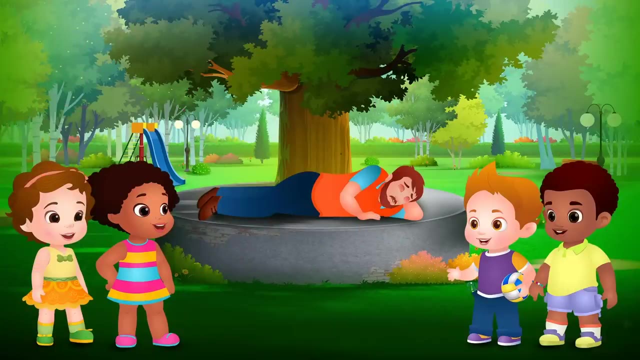 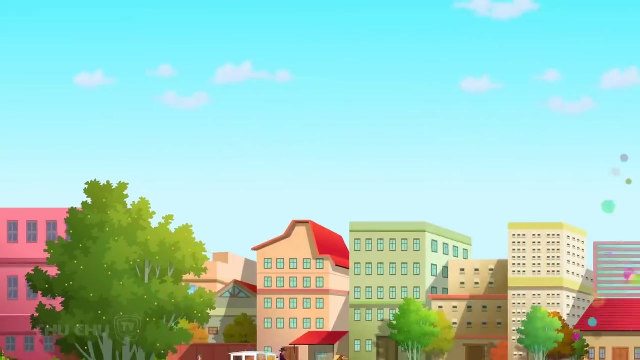 From that day onwards he realized his folly and decided to be gentle to one and all. He promised that he will take good care of himself. He promised that he will take good care of his books and toys. This was in a quiet suburb in the city of Scottsdale. 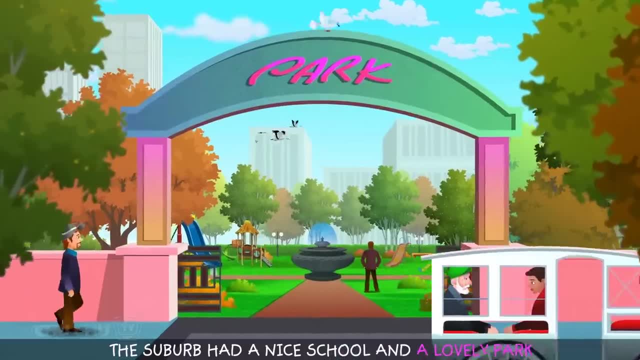 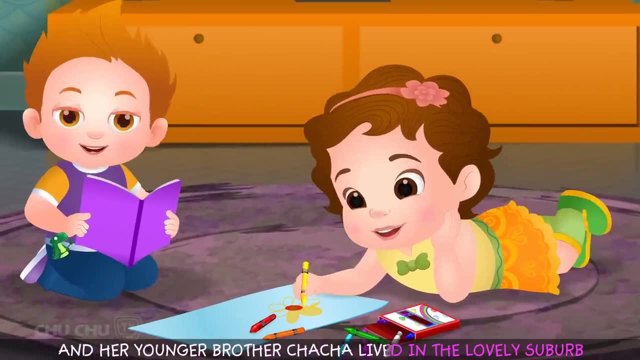 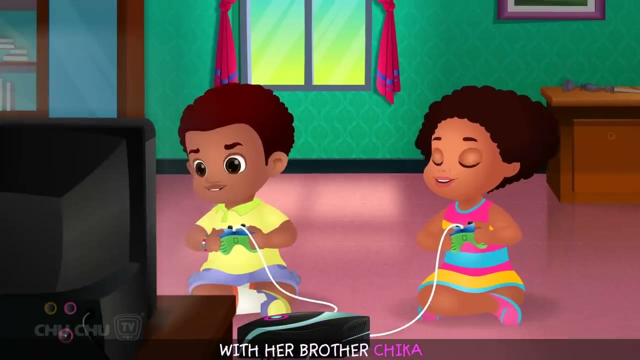 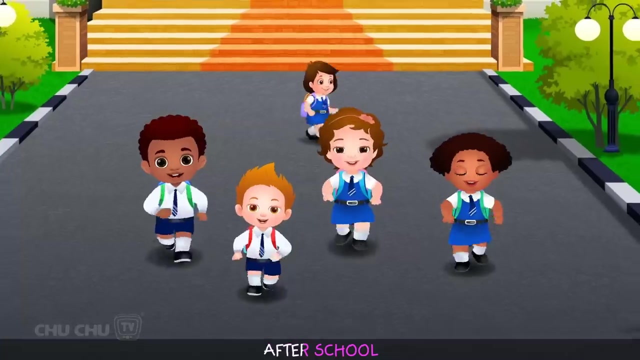 The suburb had a nice school and a lovely park. A little girl named Choo Choo and her younger brother Cha Cha lived in the lovely, quiet suburb. Next door lived a little girl, Chiku, with her brother Chica. They all went to the same school and were very close friends. 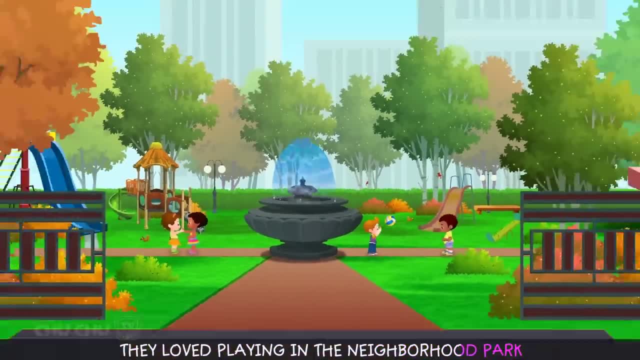 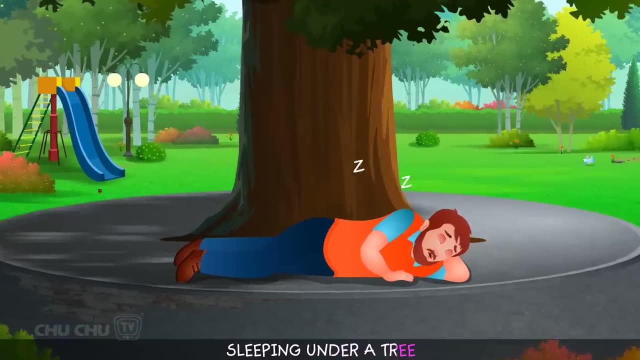 After school they loved playing in the neighborhood park. One day, while playing, they had noticed a man sleeping under a tree. This man seems to be sleeping whenever we want him to sleep. This man seems to be sleeping whenever we want him to sleep. 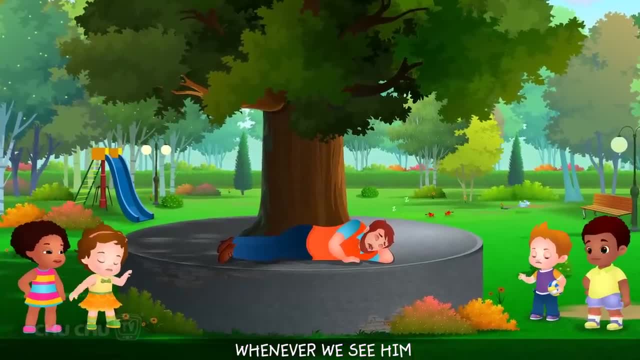 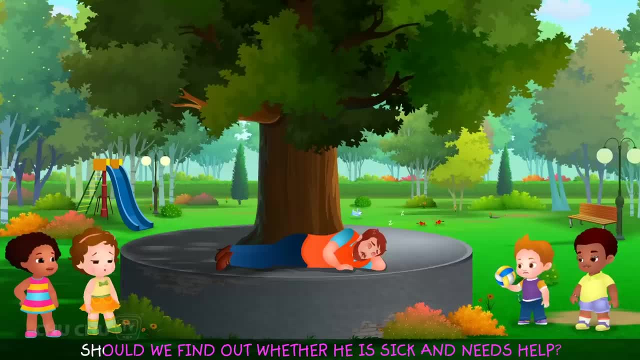 It's really cool to see him sleep with a baby. It's really cool to see him sleep with a baby. It was so cool when he sleep with a baby, But again, when we see him, it's free. Oh yeah, I noticed that too. 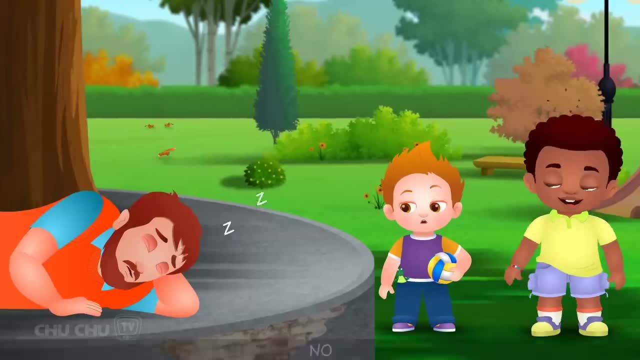 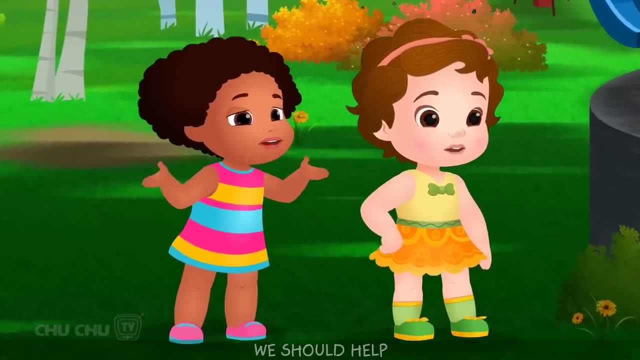 Should we find out whether he is sick and needs help? No, let's not go near strangers and talk to them, But we should help, But we should help. Once we go home, let's tell mom and try to help him. 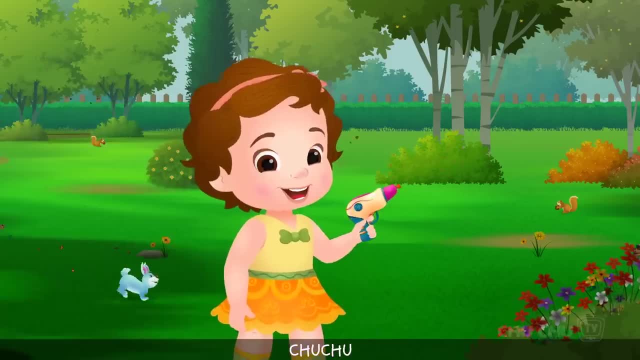 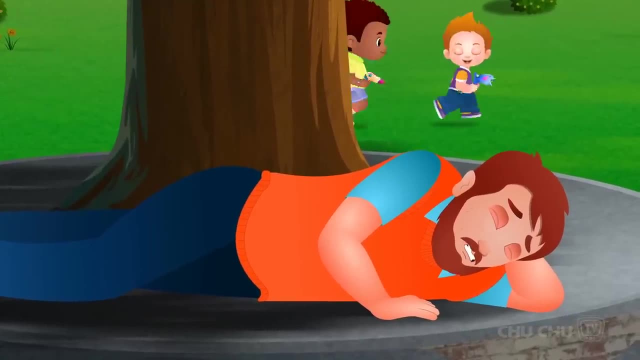 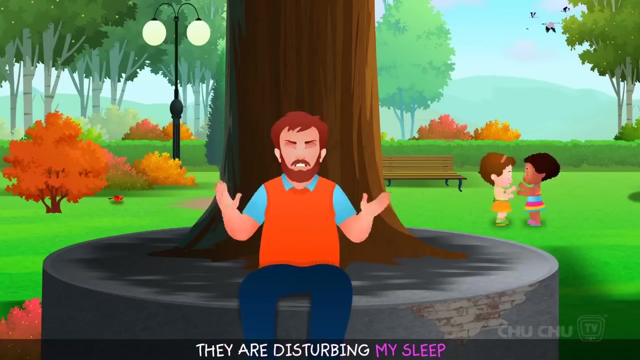 You are right, Let's do that. Choo-Choo, Cha-Cha, Cha-Cha, Chiku and Chika started to play. I need to get rid of these kids. They are disturbing my sleep. Need to make sure they never come back. 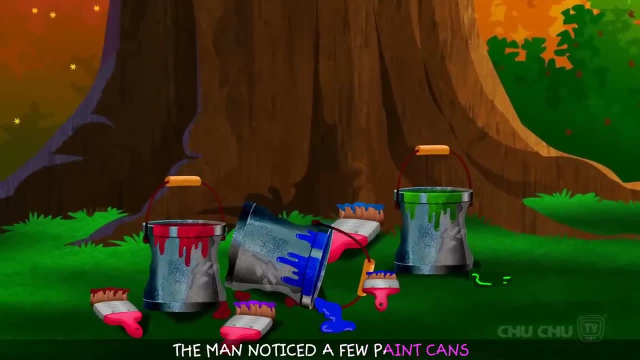 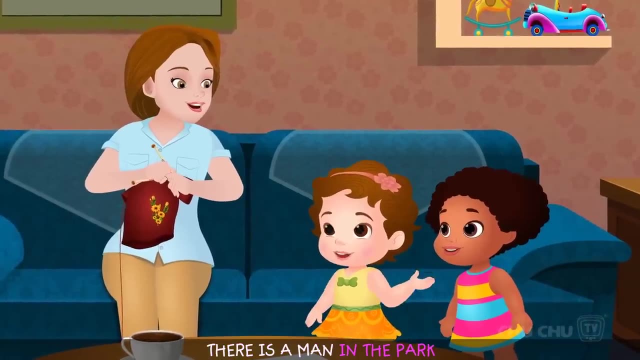 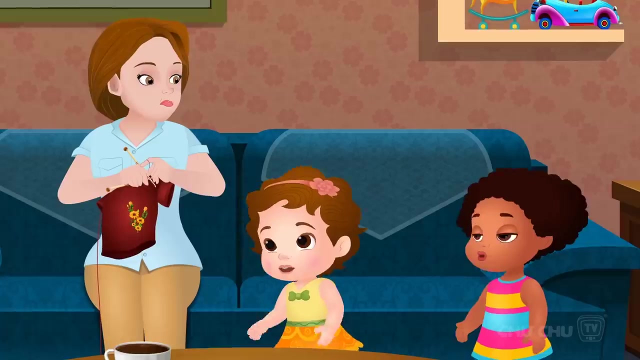 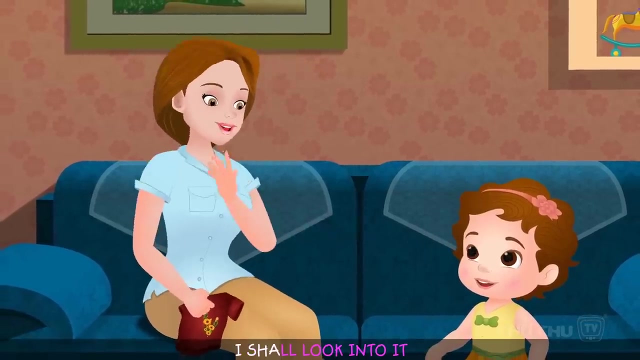 Looking around, the man noticed a few paint cans. Mommy, there is a man in the park who is always sleeping. We fear that he is sick. We wanted to tell you and get him help. Good job, I shall look into it. 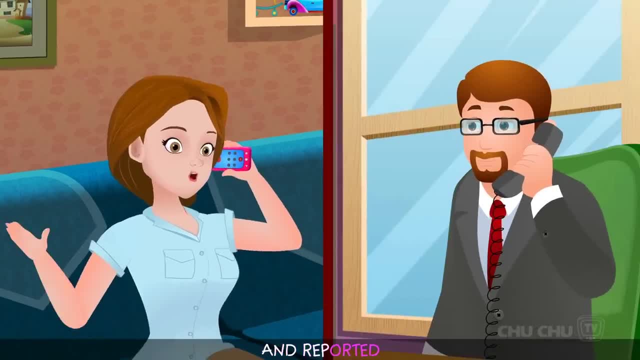 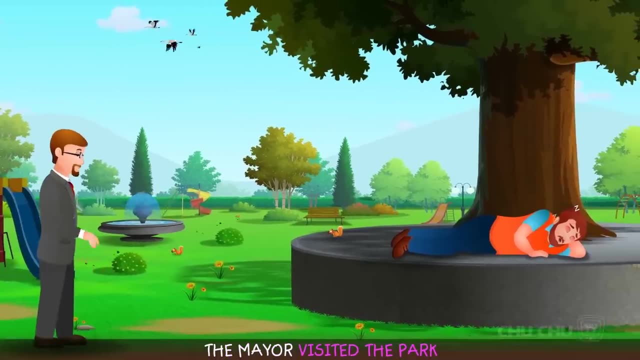 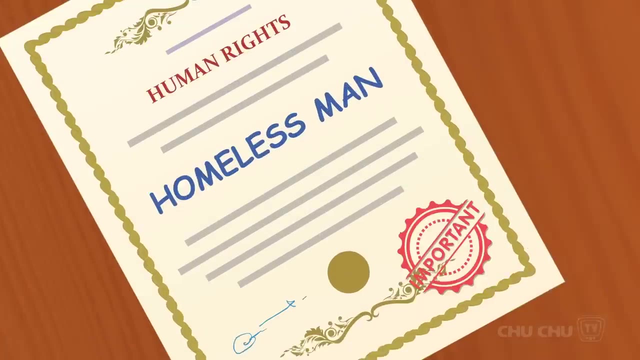 Chuchu's mom called the mayor's office and reported. The mayor's office assured to have a look. The mayor visited the park and he put a community notice: Homeless man. The mayor left the park and the man started to paint the monster. 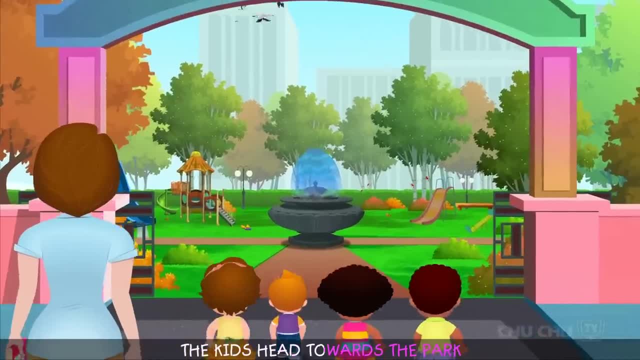 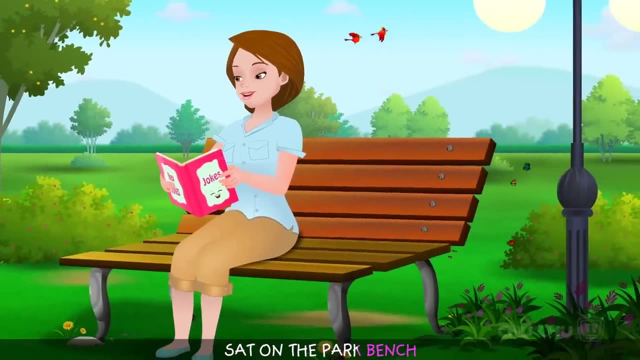 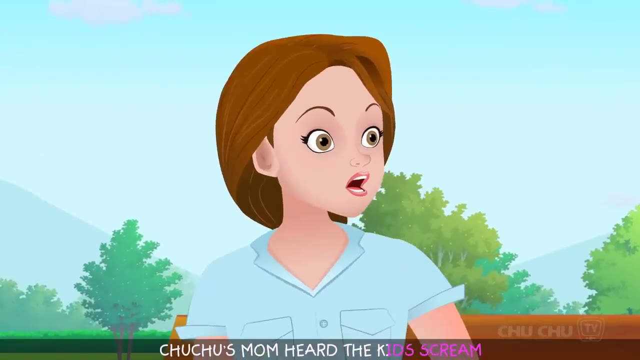 The weekend had started, The kids head towards the park wanting to play. Chuchu's mom, with a book in her hand, sat on the park bench. Mommy, Mommy, All of a sudden Chuchu's mom heard the kids scream. 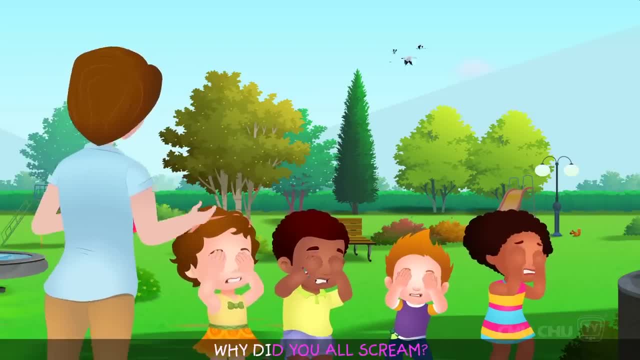 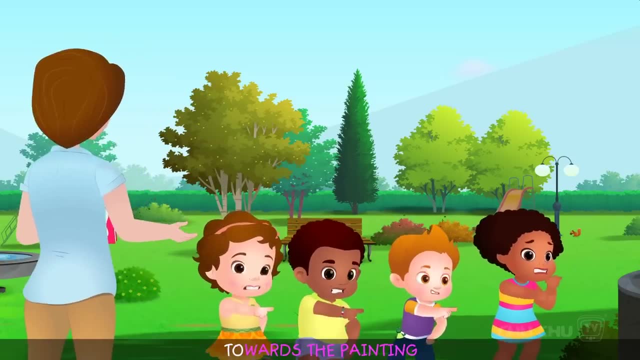 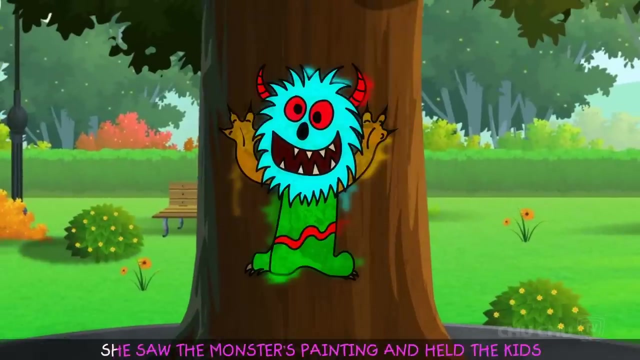 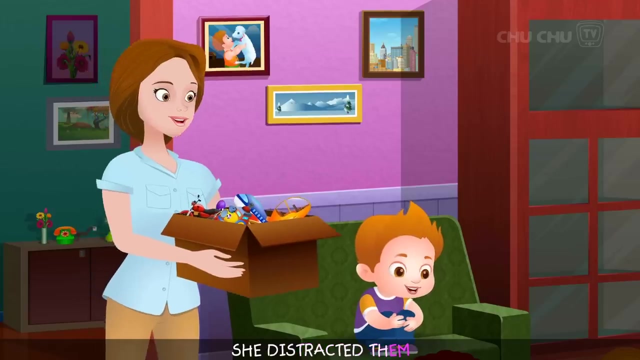 Whoa, What's wrong? Why did you all scream? Why are you trembling? The kids pointed their fingers towards the painting. She saw the monster's painting and held the kids. She distracted them by giving them some toys and a little candy. 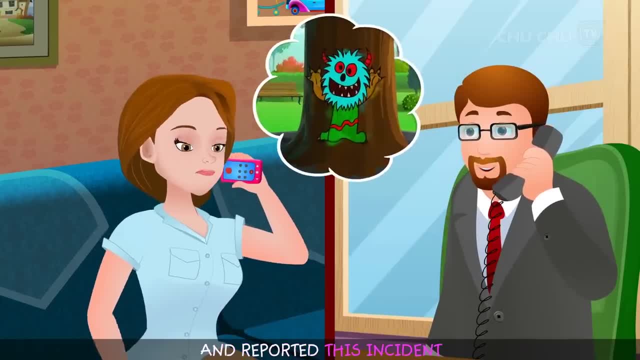 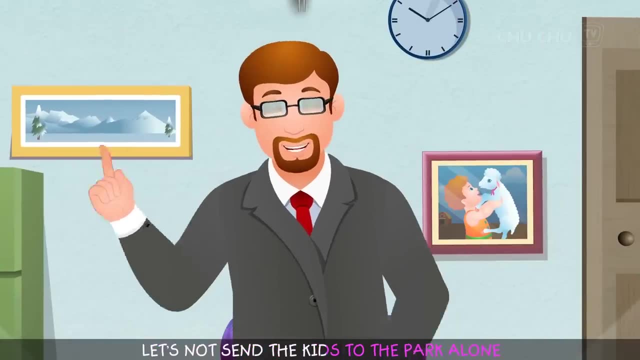 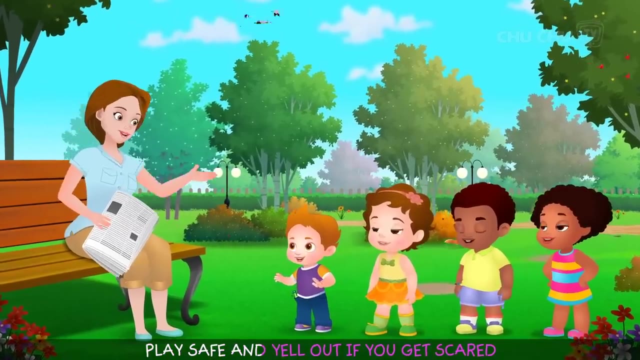 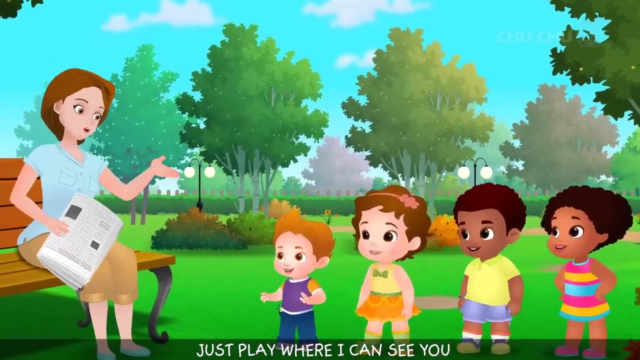 She called the mayor's office and reported this incident. Folks, till we figure this out, let's not send the kids to the park alone. Play safe and yell out. if you get scared, I'm right here, Just play where I can see you. 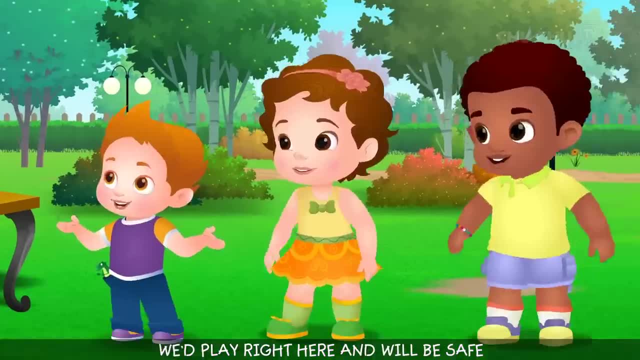 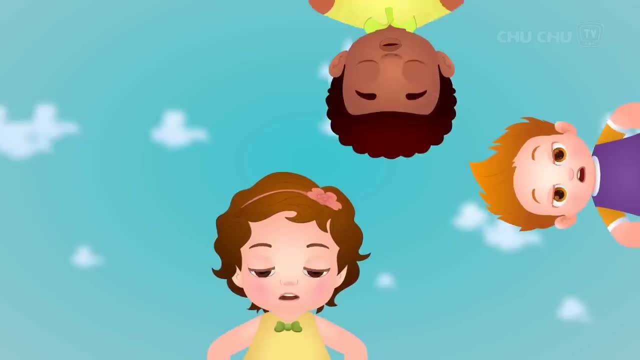 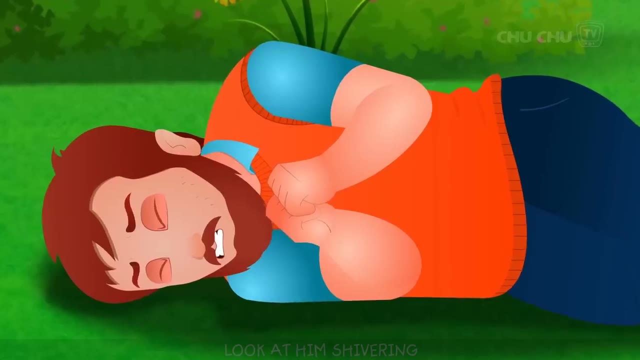 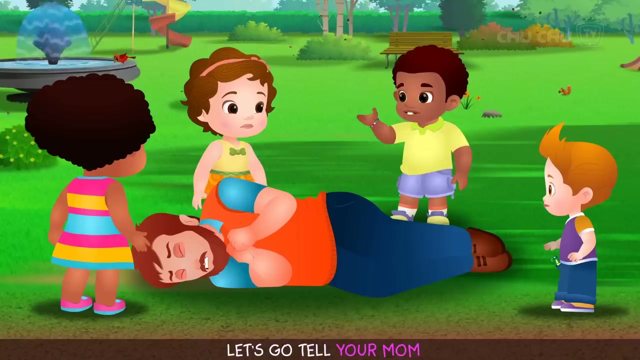 We play right here and we'll be safe. As they were playing, they see the man shivering. Cha-cha, Looks like the man is really sick. Look at him shivering. You were right. Let's go tell your mom. 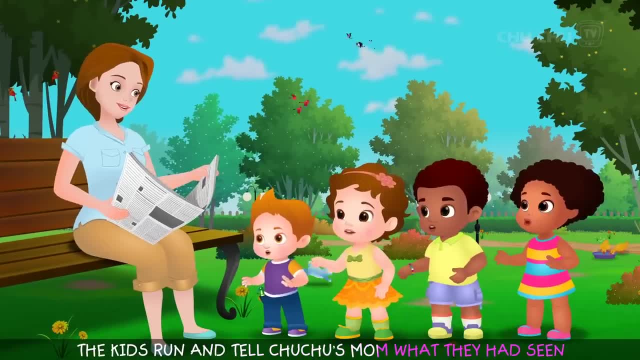 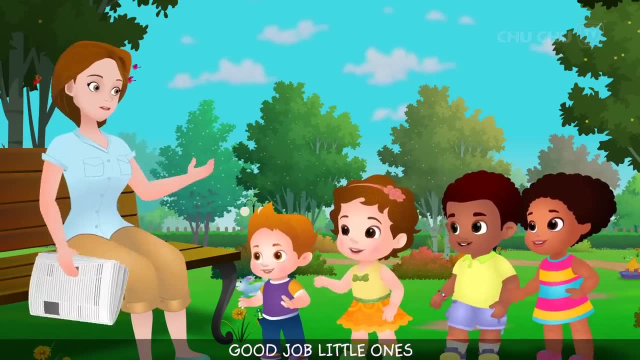 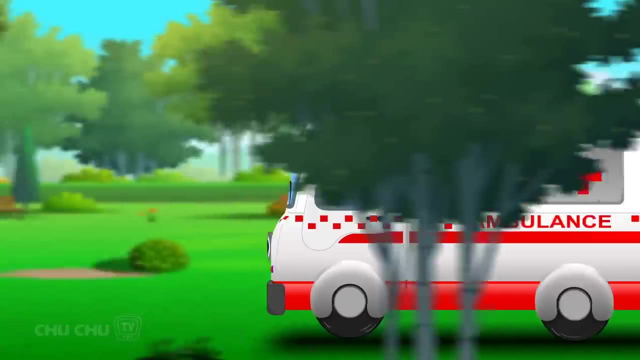 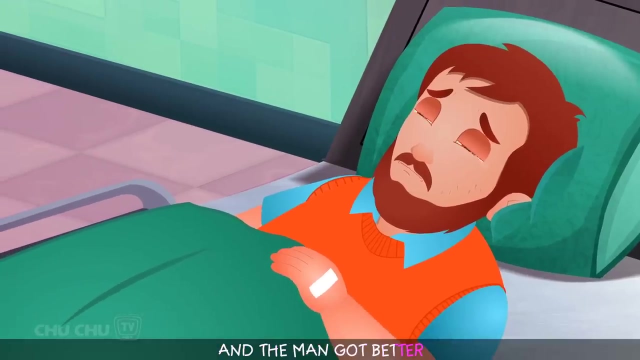 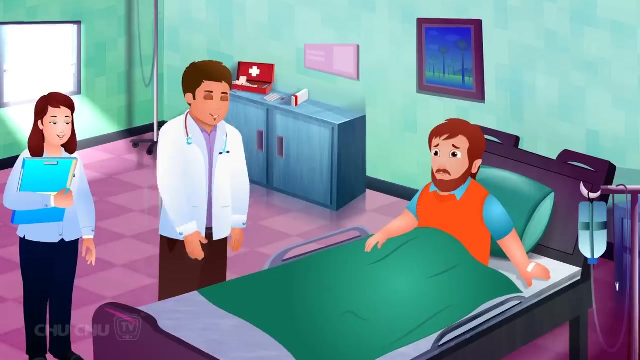 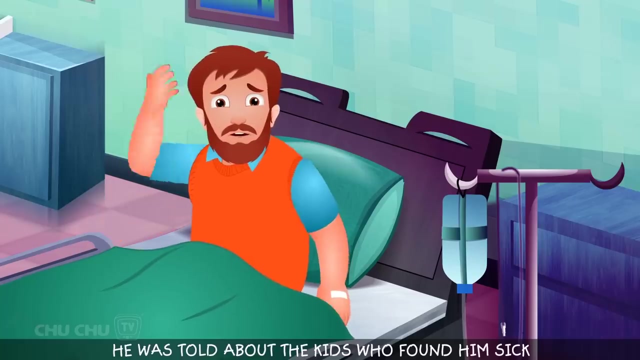 The kids run and tell Chuchu's mom what they had seen. Good job, little ones. Let me call for an ambulance to take him to the hospital. And the man got better Who brought me to the hospital. He was told about the kids who found him sick. 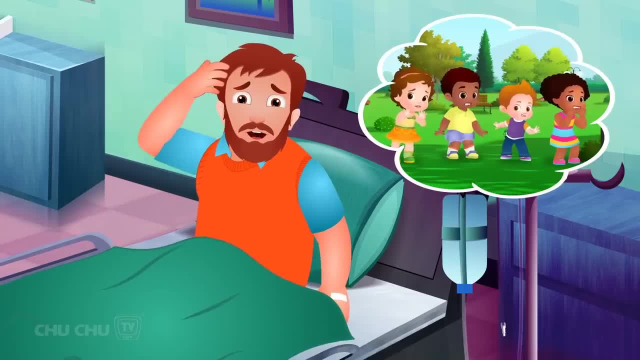 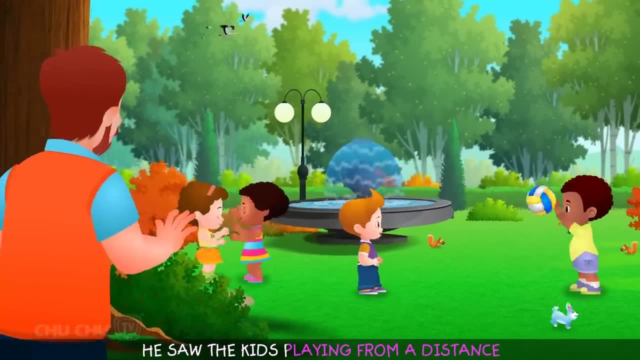 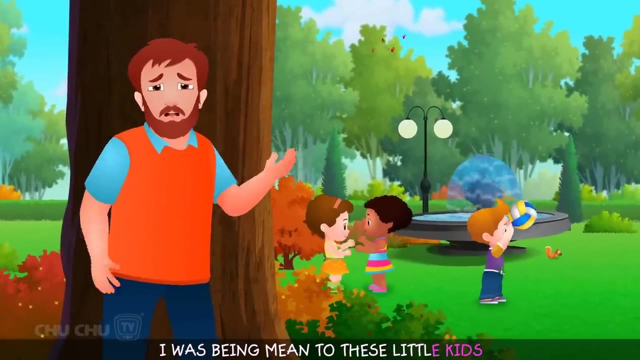 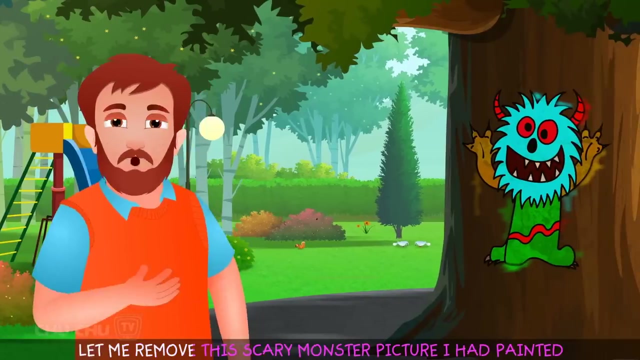 The man felt bad of his misdeed. Discharged from the hospital, the man went to the park. He saw the kids playing from a distance. I was being mean to these little kids. It's time to make it right. Let me remove the scary monster picture I had painted. 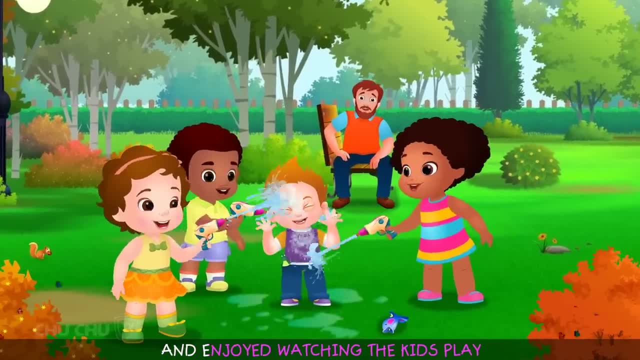 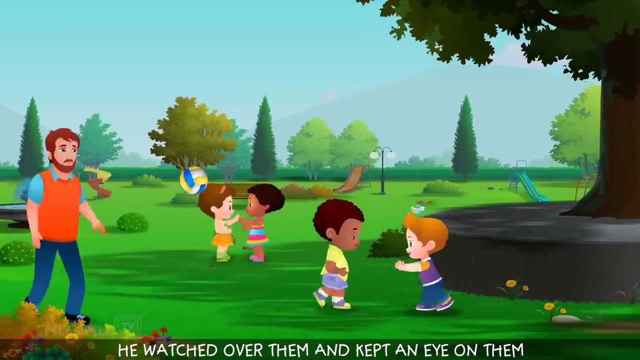 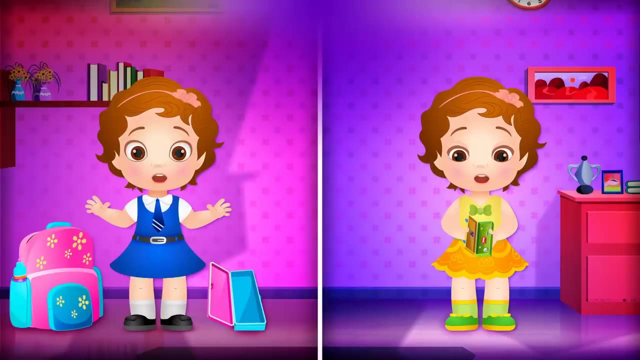 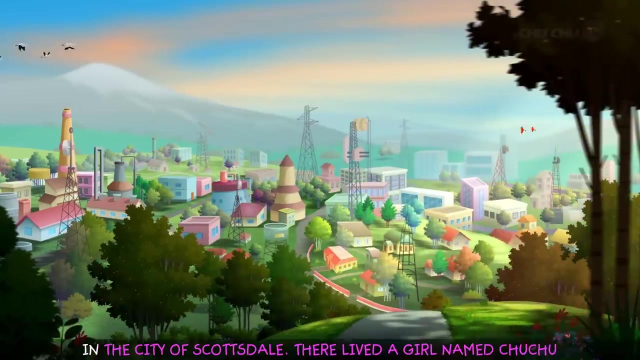 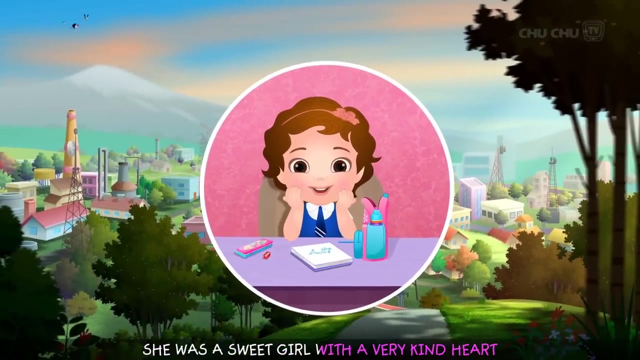 From that day onward he sat and enjoyed watching the kids playing. He watched over them and kept an eye on them ever after. In the city of Scottsdale there lived a girl named Chuchu. She was a sweet girl with a very kind heart. 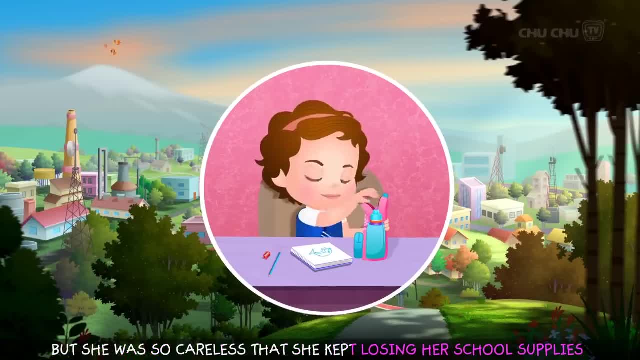 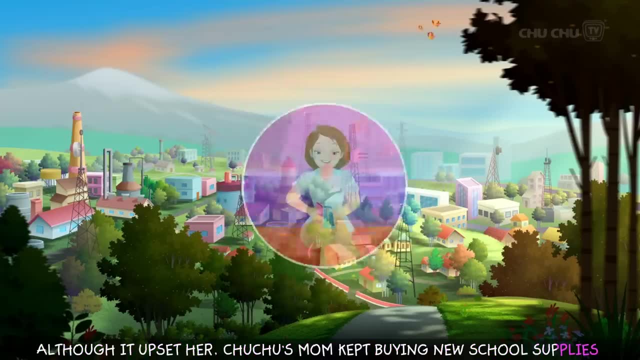 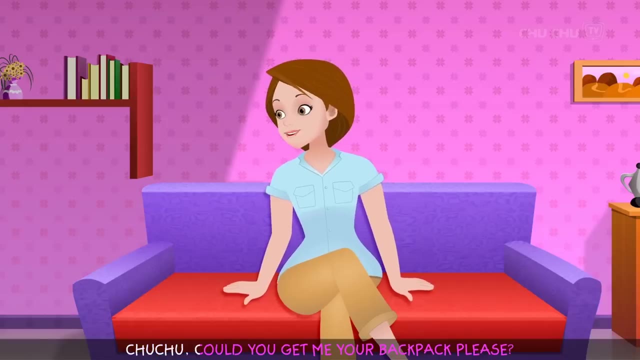 But she was so careless that she kept losing her school supplies, Although it upset her. Chuchu's mom kept buying new school supplies. Then one Monday morning her mommy yelled out: Chuchu, could you get me your backpack please? 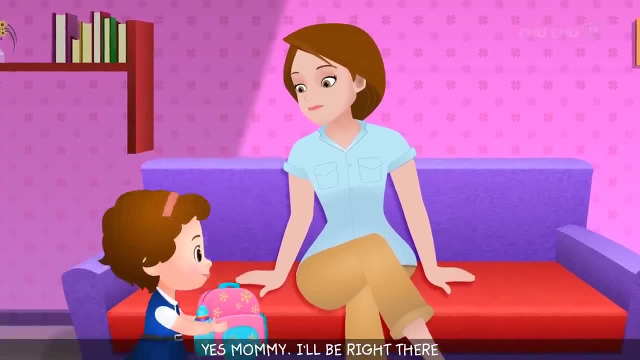 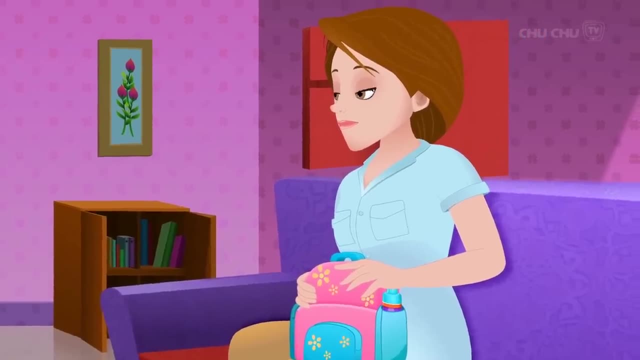 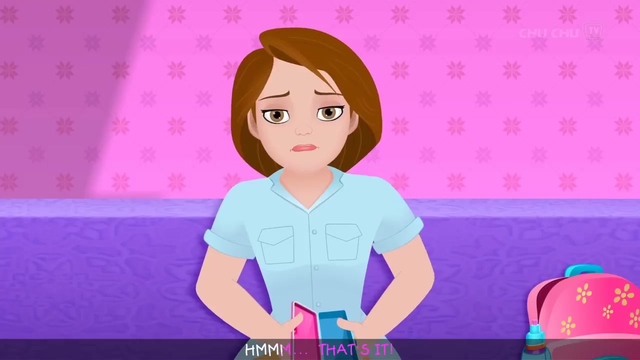 Yes, mommy, I'll be right there. Here it is. I've got to run to the restroom. I'll be right back. Her mom took out her pencil case and found it to be empty. Hmm, that's it. I've had enough of her losing her school supplies. 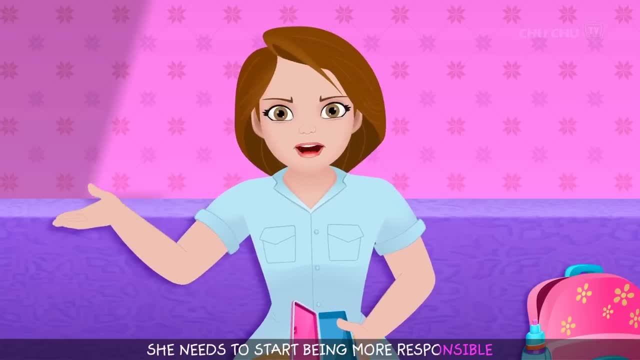 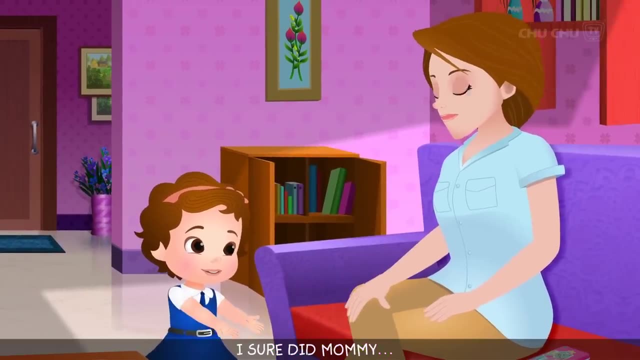 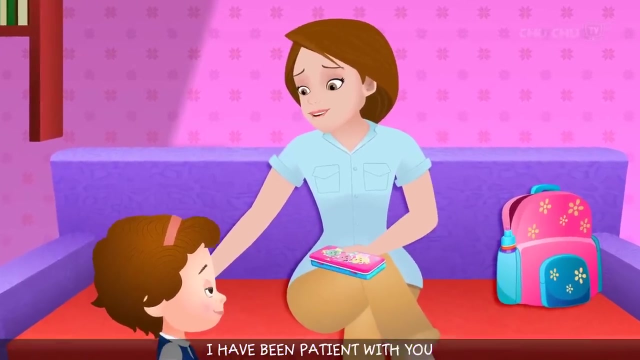 This needs to stop. She needs to start being more responsible. Did you wash your hands? I sure did, mommy. Good job, Listen, young lady. I have been patient with you. I've replenished your empty pencil case with school supplies every single day. 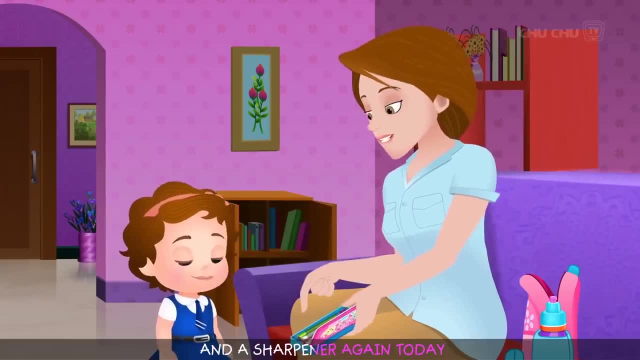 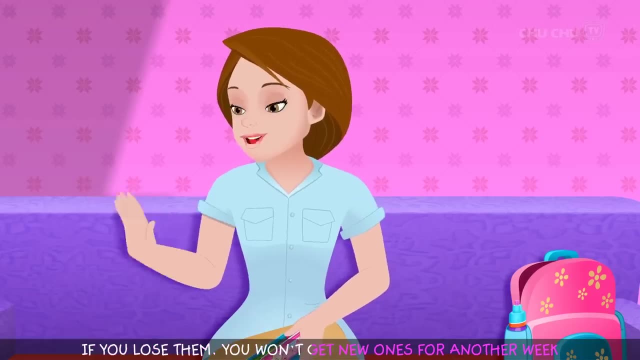 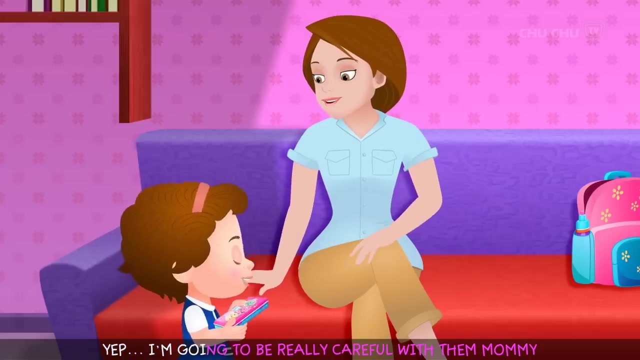 I have replenished it with two new pencils and a sharpener again today. These are going to be your school supplies for the whole week. If you lose them, you won't get new ones for another week. Have I made myself clear? Yep, I'm going to be really careful with them, mommy. 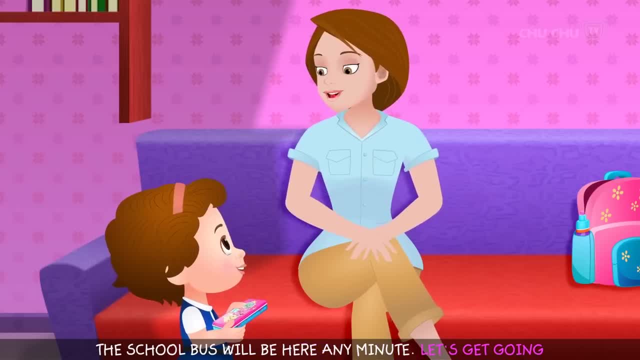 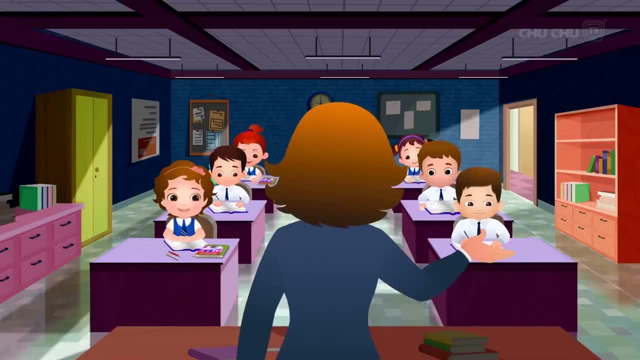 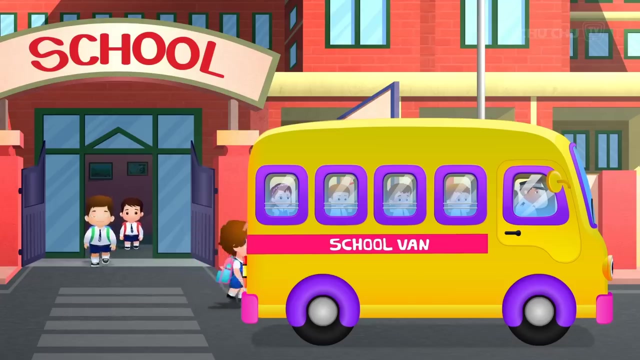 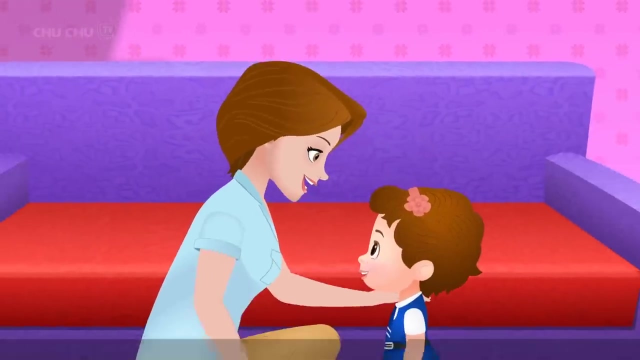 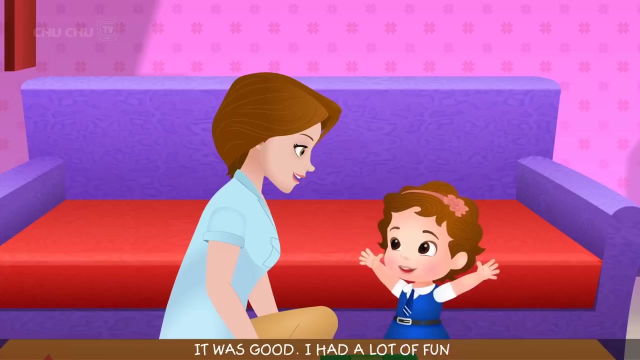 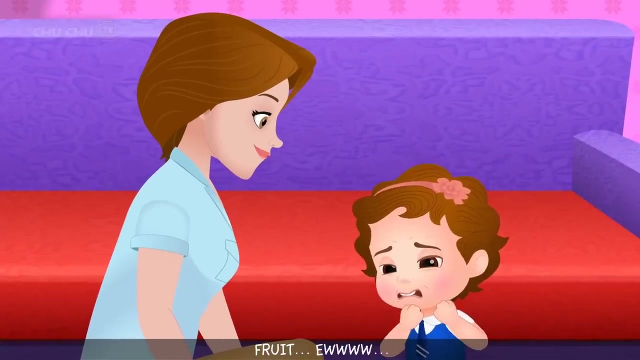 Good, The school bus will be here any minute. Let's get going. So how was your day at school? It was good. I had a lot of fun. Okay, Time to grab a fruit Fruit. Ewww, I will pretend I didn't hear that. 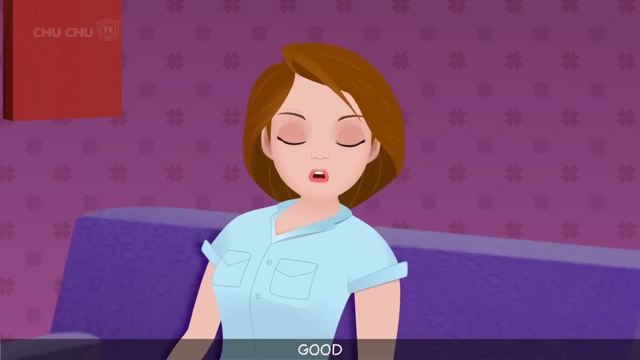 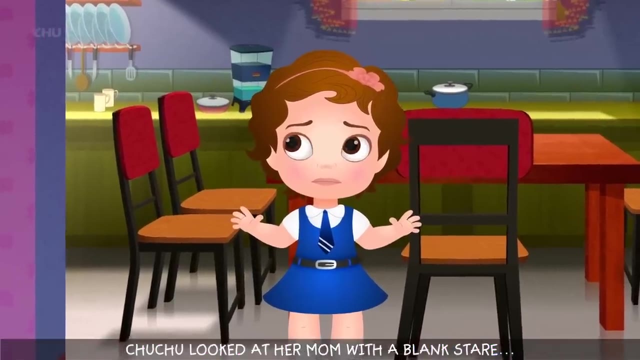 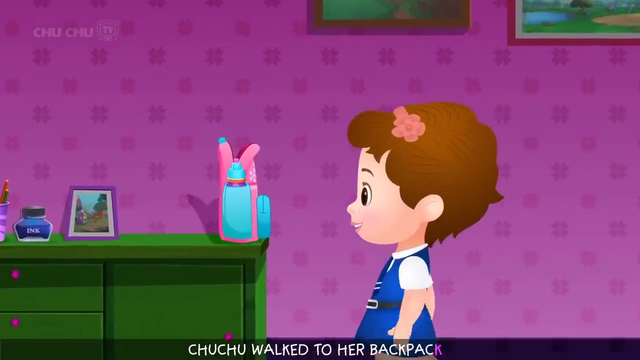 Are you done with the fruit? Yes, Good, Do you have all of your school supplies? Choo-choo looked at her mom with a blank stare. I don't remember. Hmm, Go fetch me your pencil case. Choo-choo walked to her backpack, grabbed her pencil case and gave it to her mom. 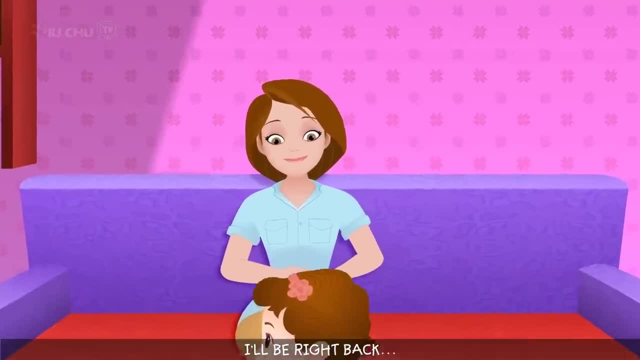 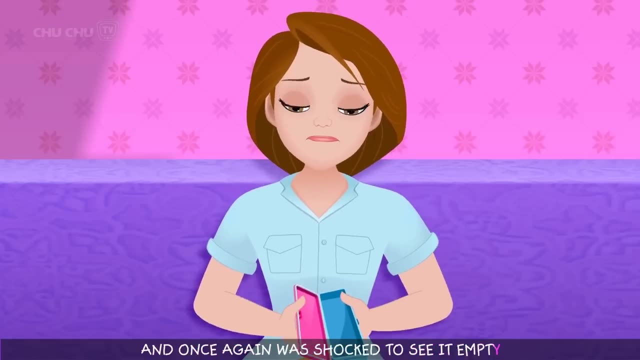 Nature calls, I'll be right back. Choo-choo's mom opened up the pencil case and once again was shocked to see it empty. Now I've had it. This girl needs to learn respect, To learn responsibility. Choo-choo, are you done? 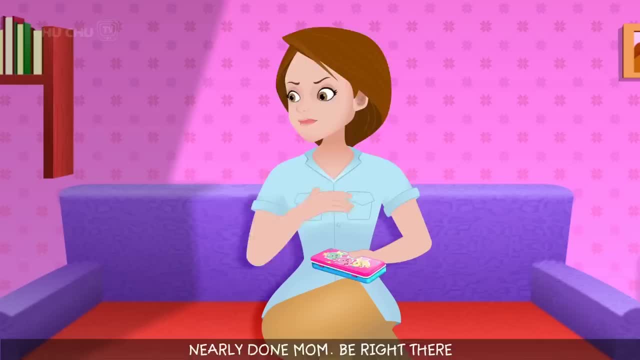 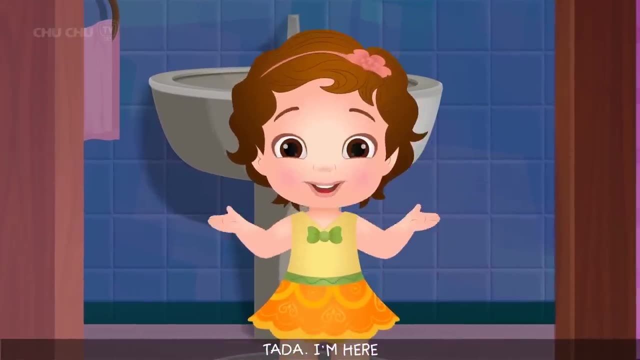 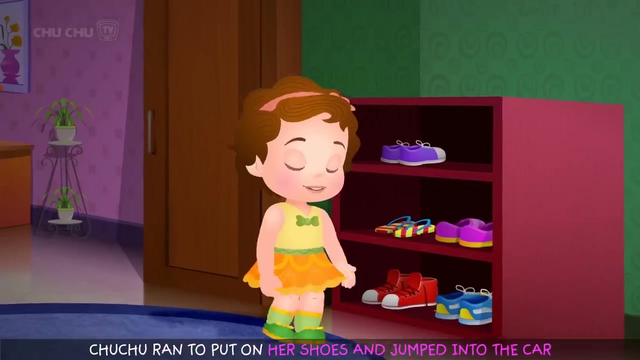 Nearly done. mom, Be right there. Hurry up, We are heading out for some shopping. Ta-da, I'm here, Put on your shoes and hop into the car. Choo-choo ran to put on her shoes and jumped into the car. 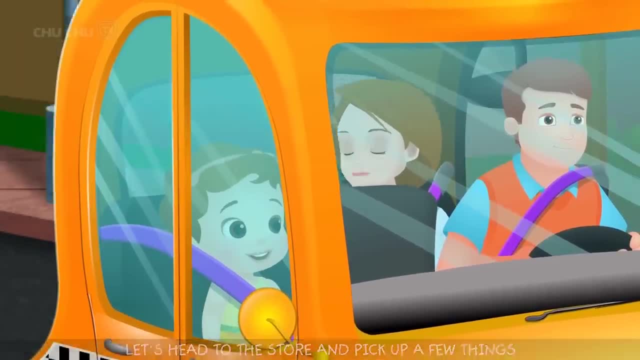 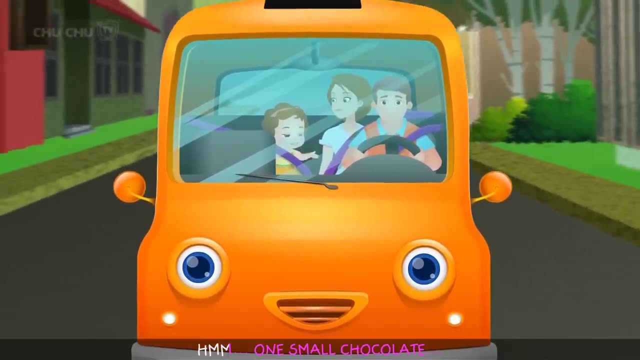 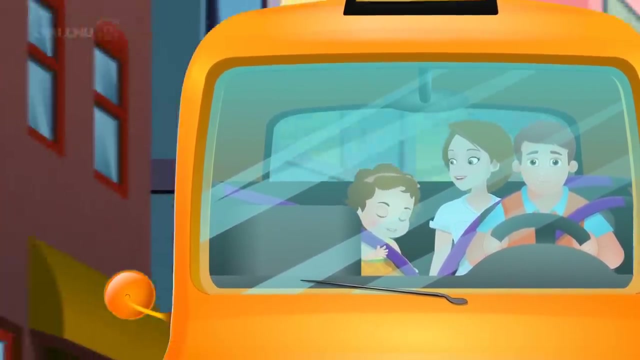 Let's head to the store and pick up a few things. Sure, mom, Uh, do I get a treat? Hmm, One small chocolate And that's it. Yay, Thank you. Choo-choo's mother stopped by the store. 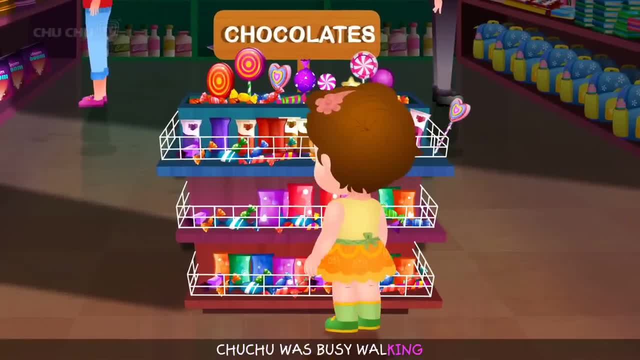 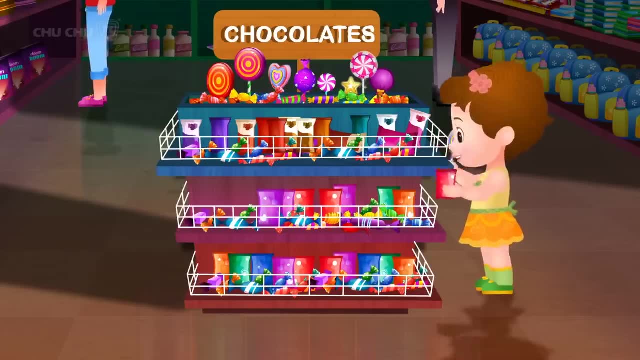 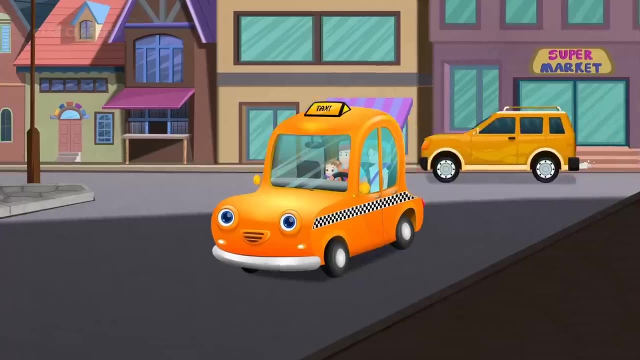 Choo-choo was busy walking along the aisle searching for her chocolate. Her mom picked up a few packs of pencils, A few sharpeners and some chocolates. The car stopped by a small foster home. Come on, Choo-choo. 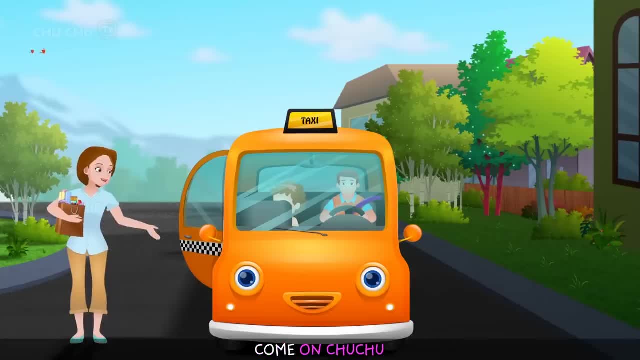 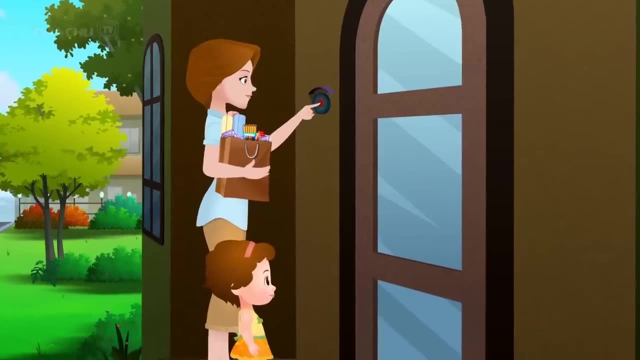 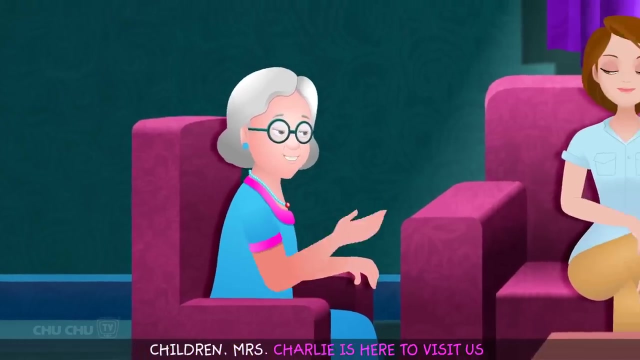 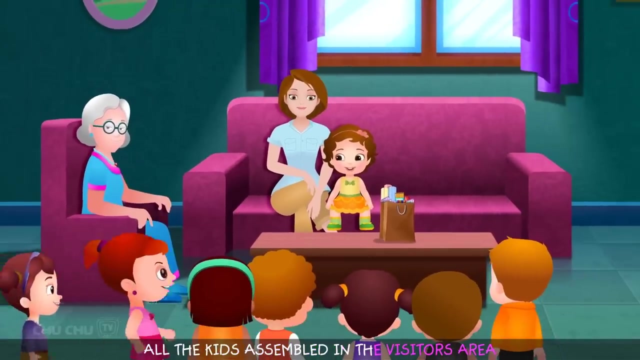 Choo-choo got down and held her mom's hand and walked along Children. Mrs Charlie is here to visit us. Could you all please come here? Yes, ma'am, Could you all please come here? All the kids assembled in the visitor's area. 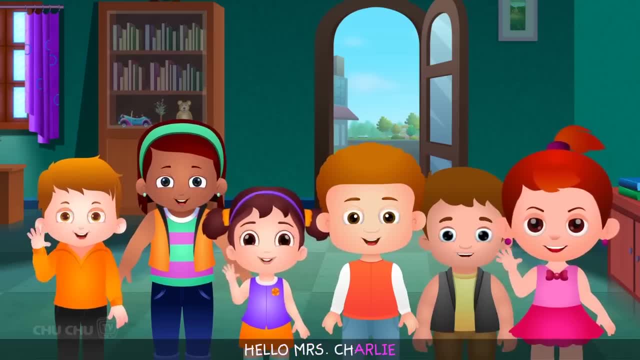 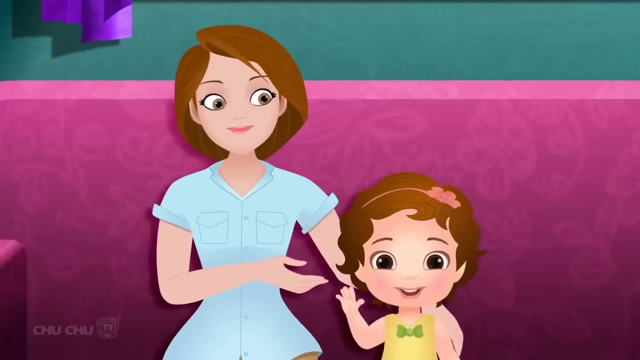 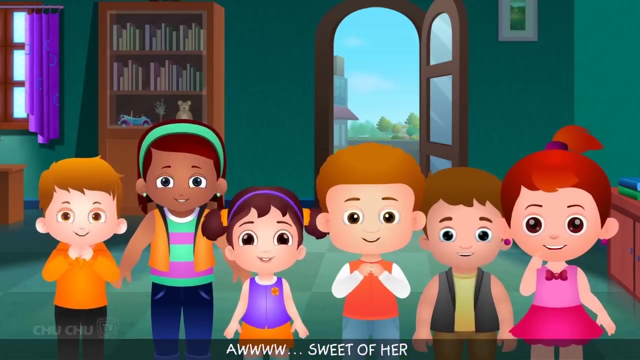 Hello little ones. Hello Mrs Charlie. This is my daughter Choo-choo. Hello Choo-choo. She wanted to visit you all and play with you. Aww, sweet of her. Could you kids teach her how to draw? 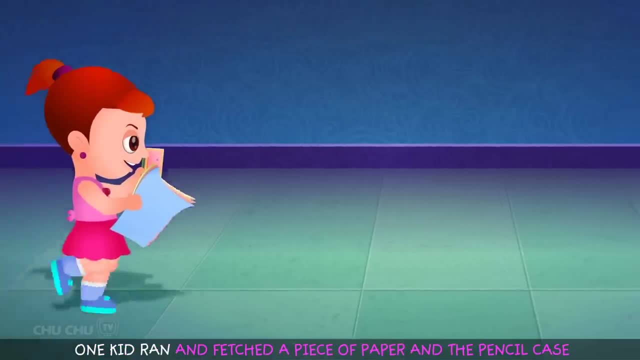 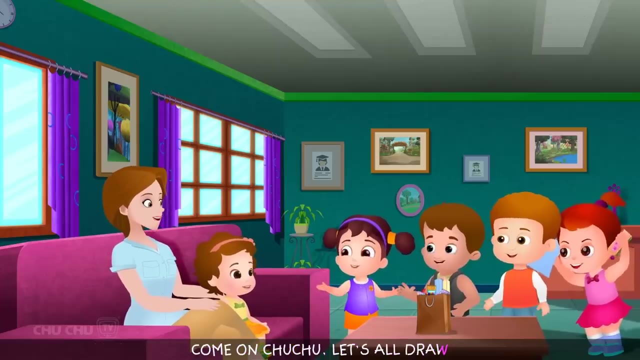 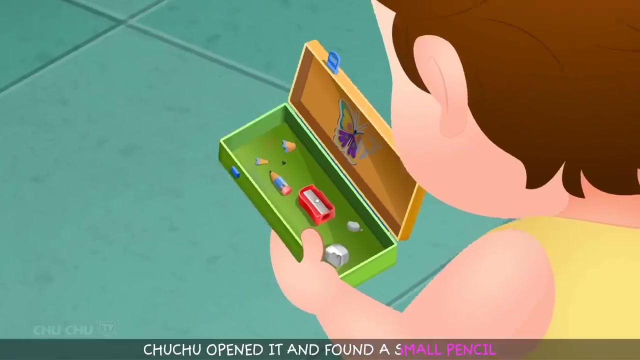 Yes, Mrs Charlie. One kid ran and fetched a piece of paper and the pencil case. Come on, Choo-choo, Let's all draw. The kids gave the pencil case to Choo-choo. Choo-choo opened it and found a small pencil with a broken eraser and a broken sharpener. 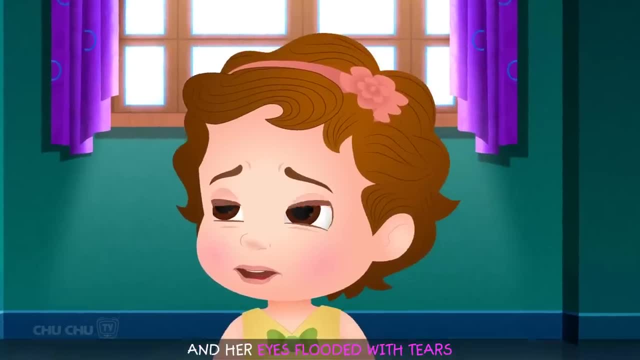 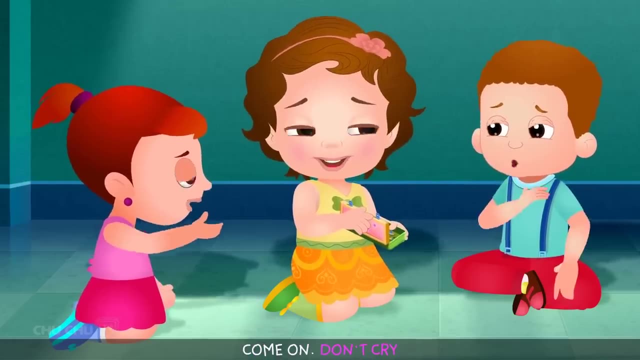 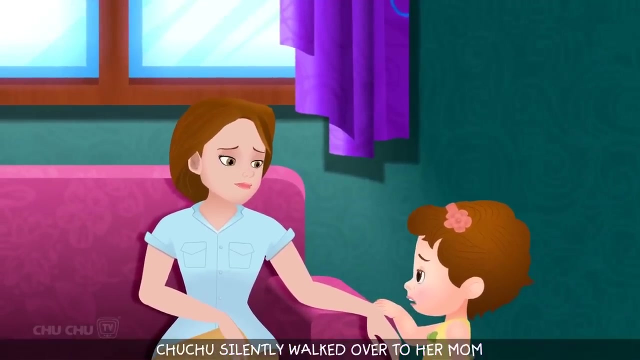 Choo-choo looked at her mom and her eyes flooded with tears. Hey, why are you crying? Come on, Choo-choo, Don't cry. Choo-choo silently walked over to her mom and whispered in her ear: 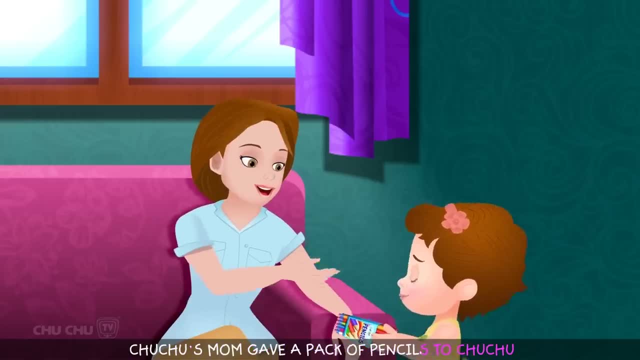 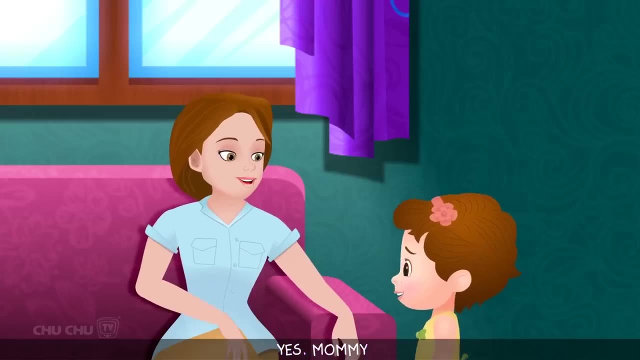 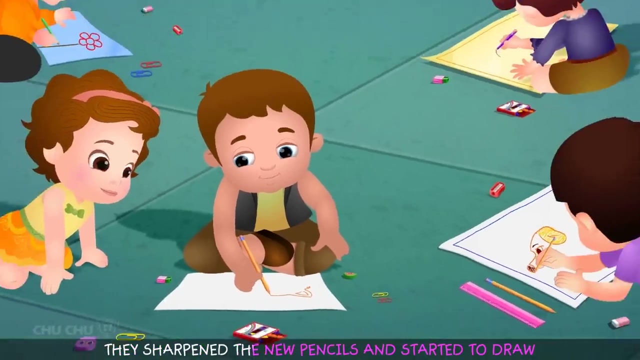 Choo-choo's mom gave a pack of pencils to Choo-choo. Choo-choo, share these pencils with your friends here. Yes, Mommy, All the kids jumped with joy. They sharpened the new pencils. 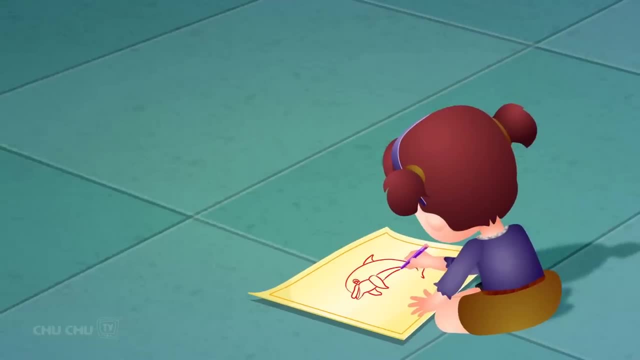 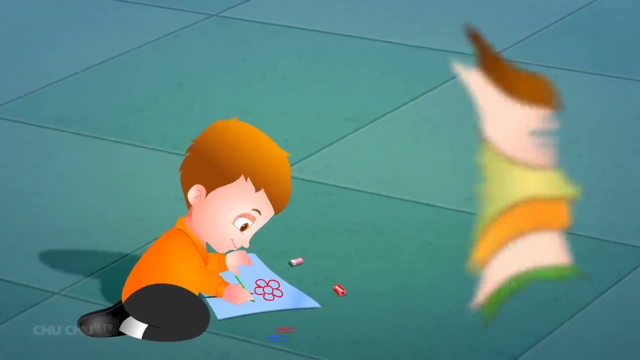 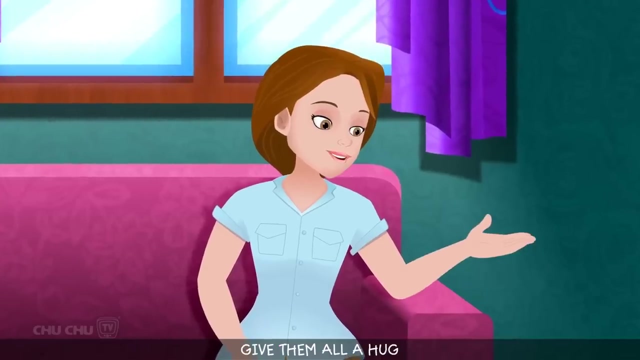 and started to draw. They sharpened the new pencils and started to draw. A few hours went by. Choo-choo, it's getting late. Give them all a hug. I know you will miss them all. Let's come back another day. 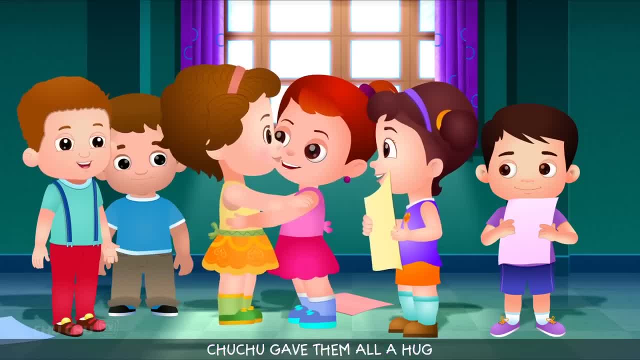 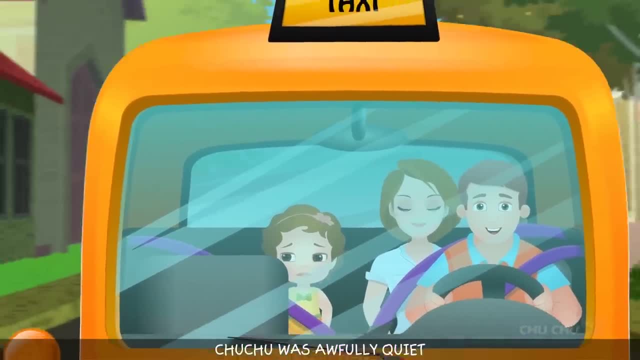 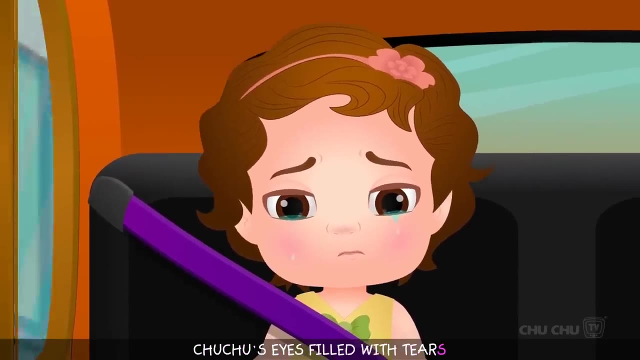 Okay, Mommy Choo-choo gave them all a hug. I'll see you all soon. Choo-choo was awfully quiet. What's wrong, Angel? Choo-choo's eyes filled with tears. She started to talk. 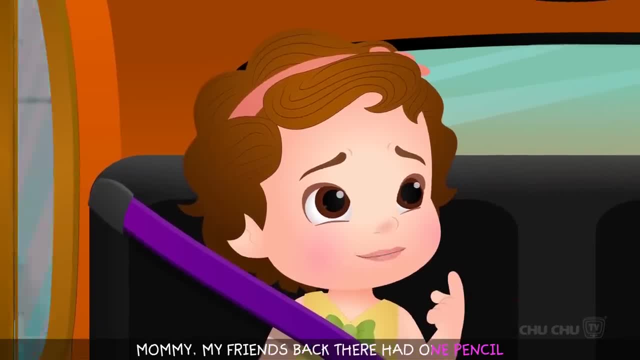 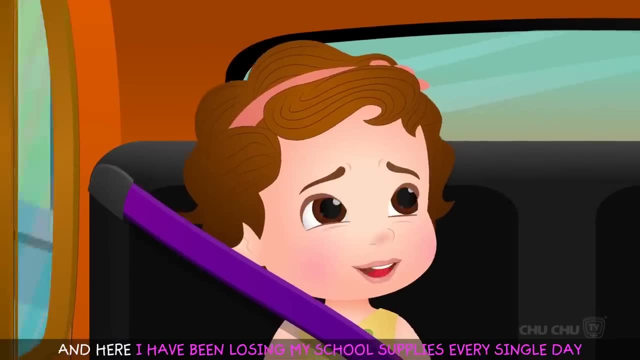 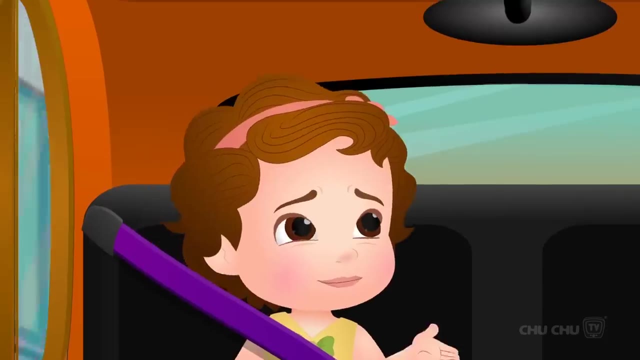 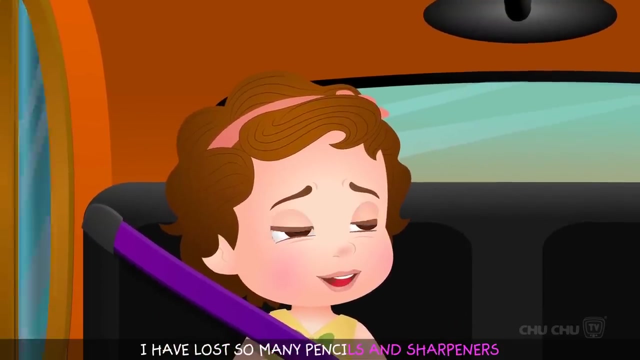 Mommy, my friends back there had one pencil with a broken eraser and a broken sharpener. Yes, they did. And here I've been losing my school supplies every single day. Hmm, I have been careless with my school supplies. I have lost so many pencils and sharpeners. 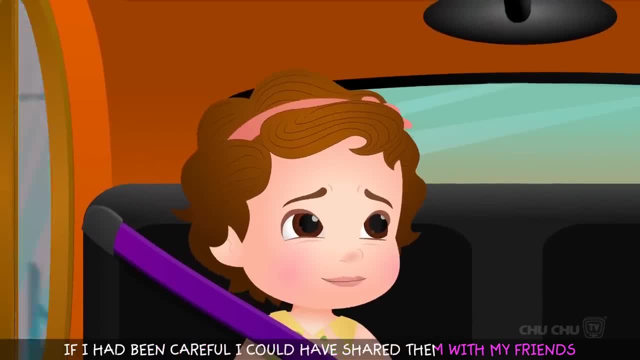 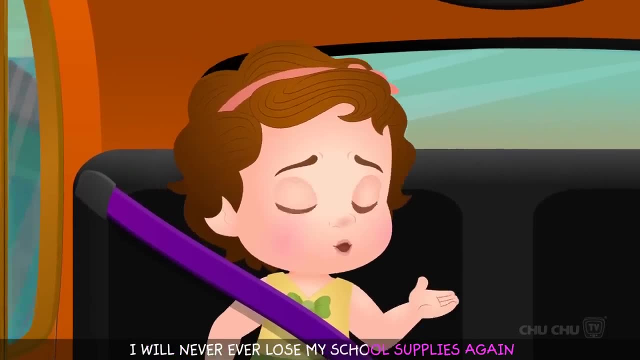 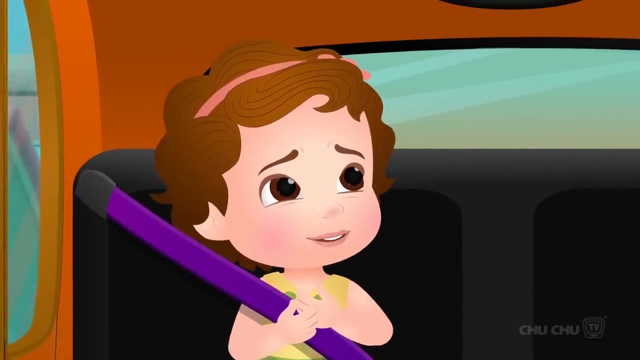 If I had been careful, I could have shared them with my friends. Mommy, Yes, darling, I will never, ever lose my school supplies again. I have realized my mistake. I will be responsible, Mommy. Good sweetheart, I'm glad you realized it. 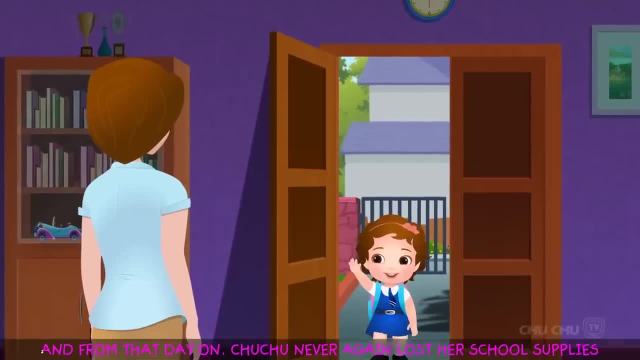 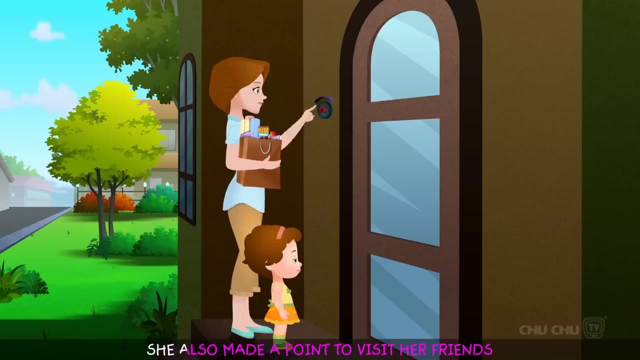 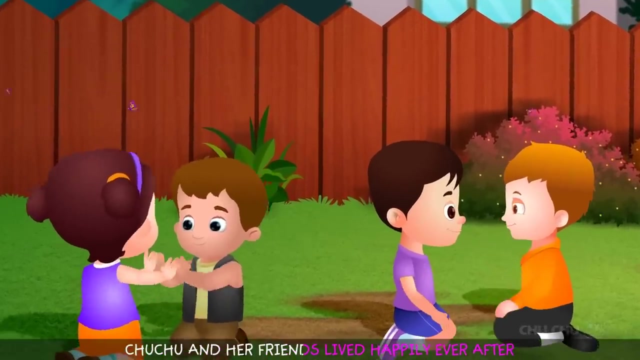 Mommy kissed Choo-choo And from that day on Choo-choo never again lost her school supplies. She also made a point to visit her friends every weekend and play with them. Choo-choo and her friends lived happily ever after. 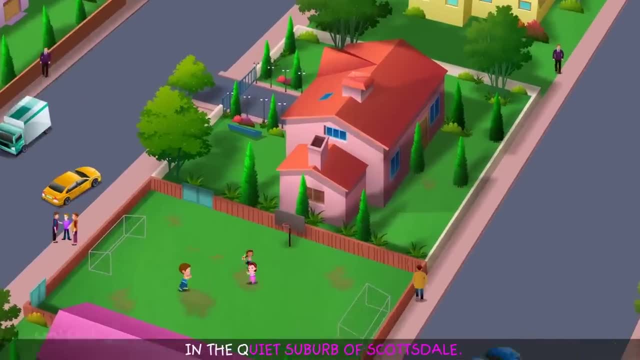 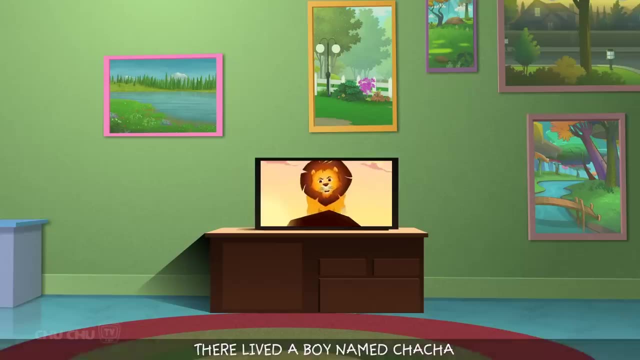 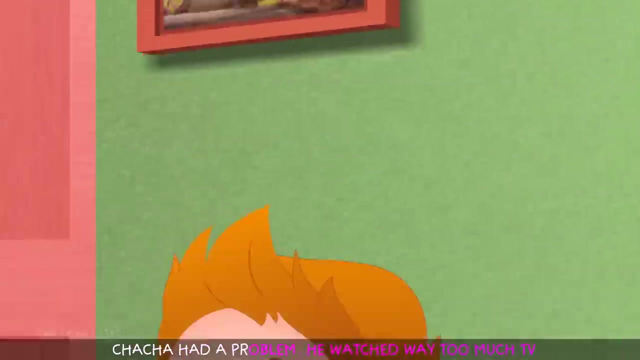 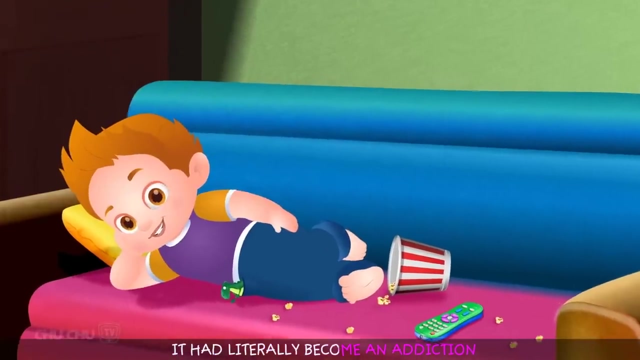 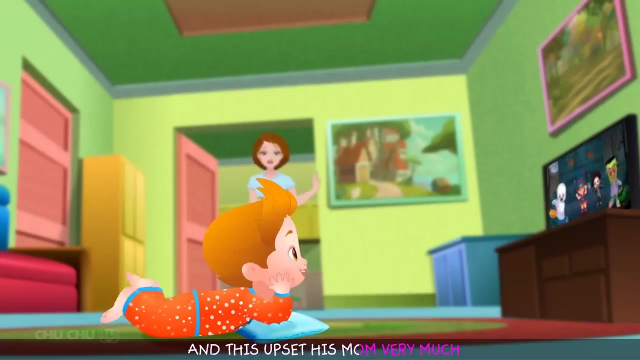 In the quiet suburb of Scottsdale there lived a boy named Cha-cha And strong as steel. Cha-cha had a problem: He watched way too much TV. It had literally become an addiction, Choo-choo- And this upset his mom very much. 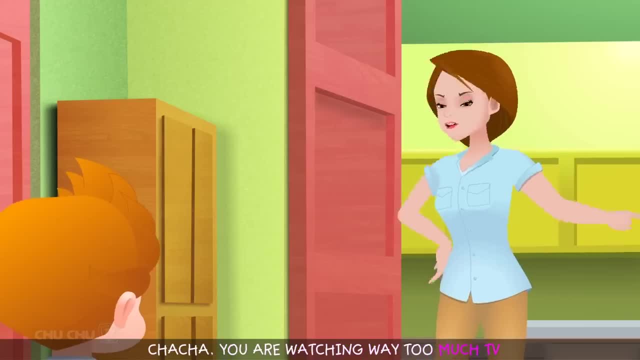 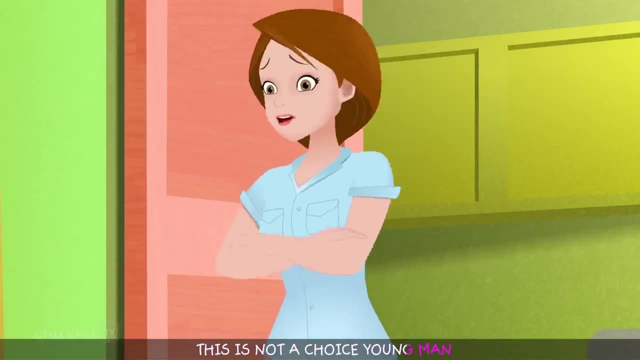 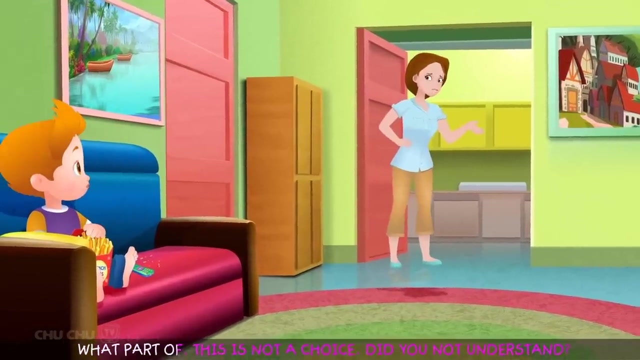 Cha-cha, you are watching way too much TV On your feet. You need to get some exercise. This is not a choice, young man. Mom, give me a break. What part of this is not a choice? did you not understand? 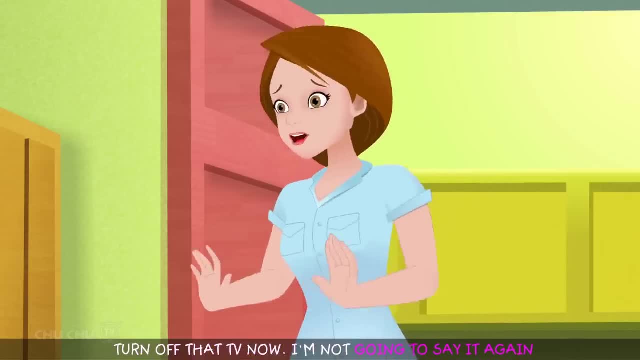 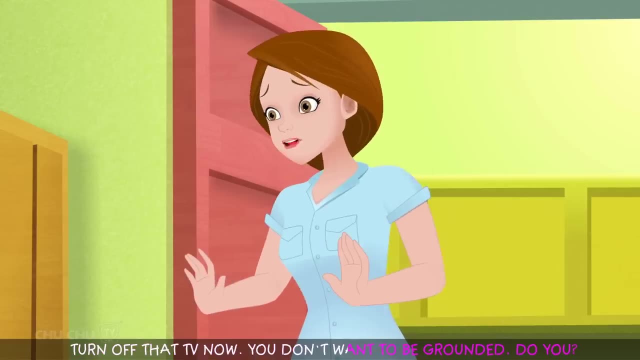 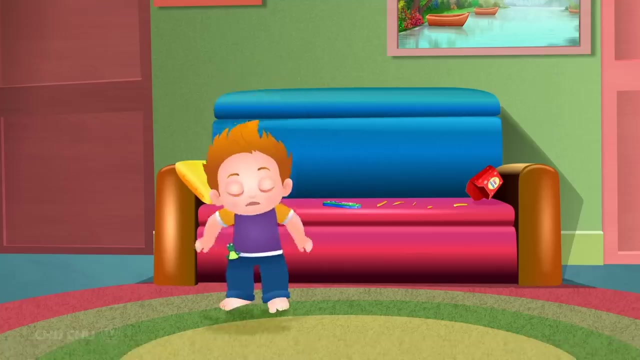 Turn off that TV now. I'm not going to say it again, But but Turn off that TV now. You don't want to be grounded, do you? Okay, stop yelling already. There it's off, Happy Good. 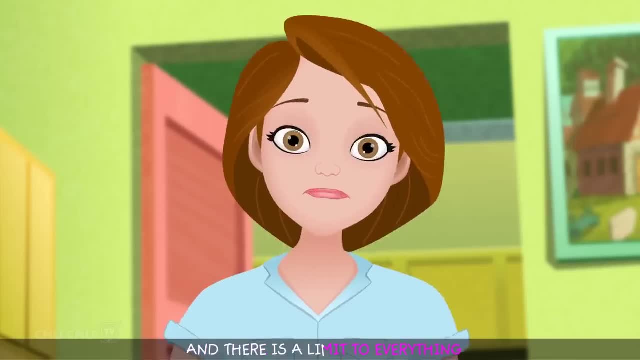 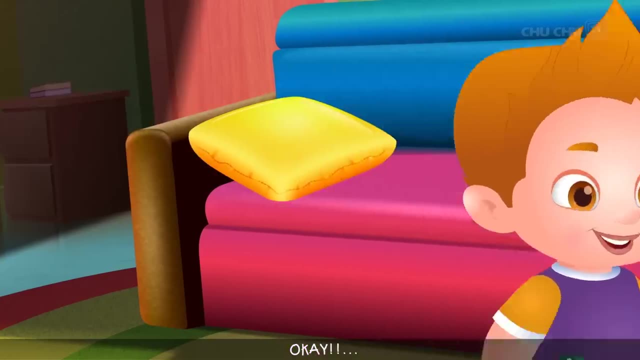 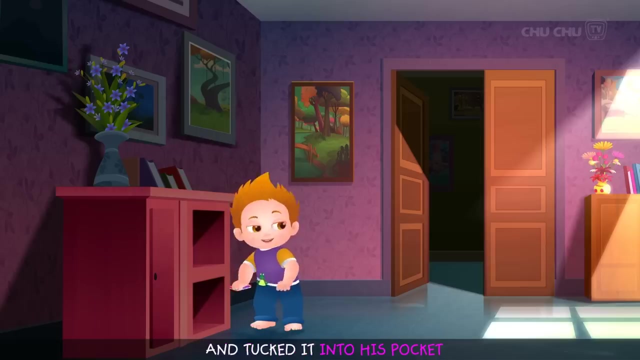 There is a time for everything And there's a limit to everything. Now, put on your shoes and go to bed. Put on your shoes and go out and play. Okay, Cha-cha grabbed his video game console and tucked it into his pocket. 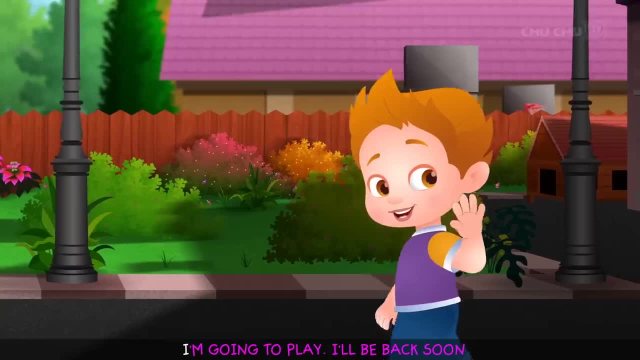 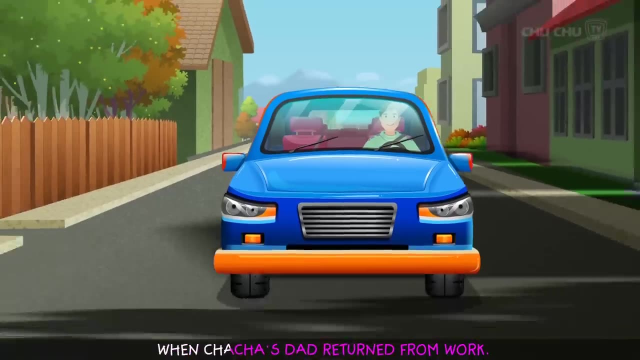 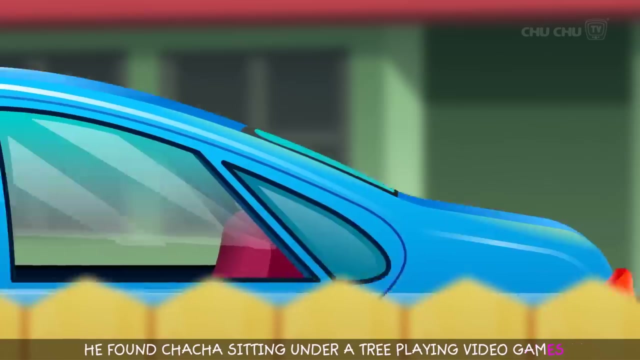 He then put on his shoes and headed out: I'm going to play. I'll be back soon. Be careful, sweetheart. When Cha-cha's dad returned from work, he found Cha-cha sitting under a tree. Cha-cha was sitting under a tree playing video games. 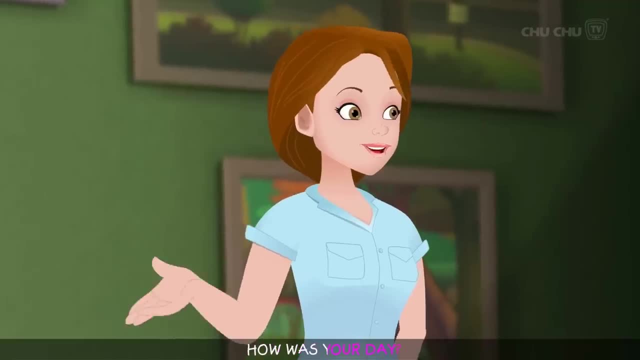 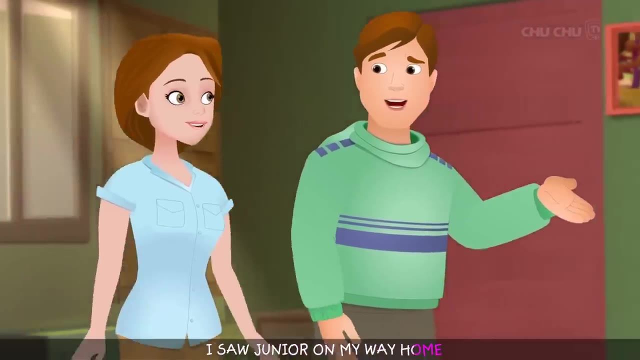 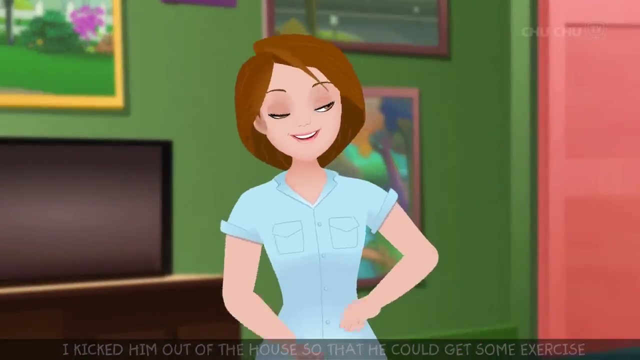 Hey, honey, I'm home. How was your day? It was good. Guess what. I saw Junior on my way home. Yeah, I kicked him out of the house so that he could get some exercise. That's not what I saw. 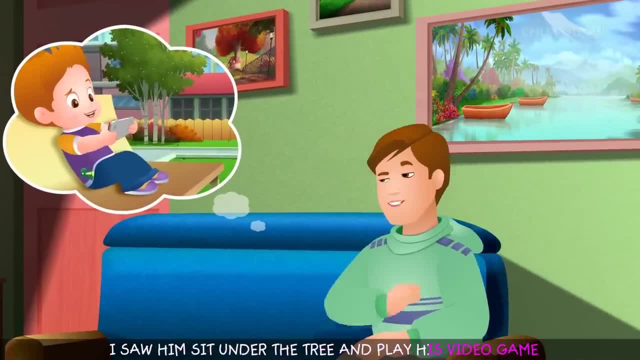 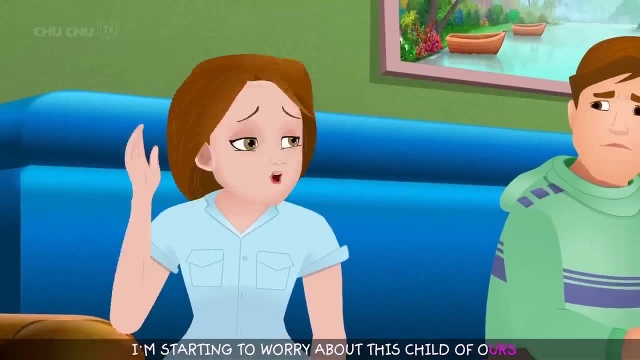 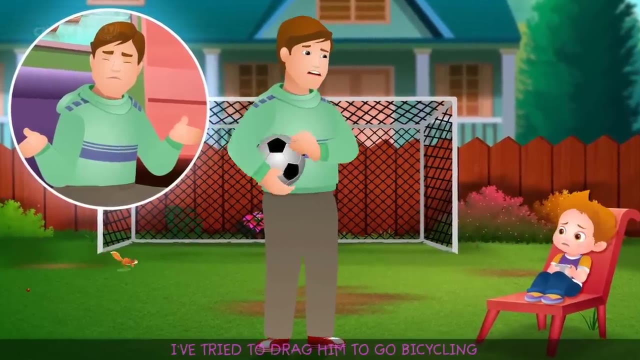 I saw him sit under the tree and play his video game. Oh no, Hmm, I'm starting to worry about this child of ours. Hmm, me too. I've tried to get him to play ball with me. I've tried to drag him to go bicycling. 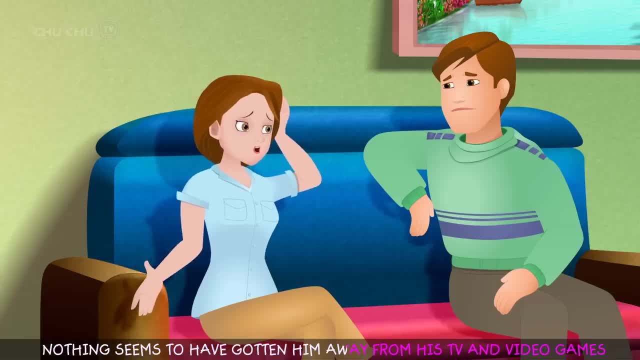 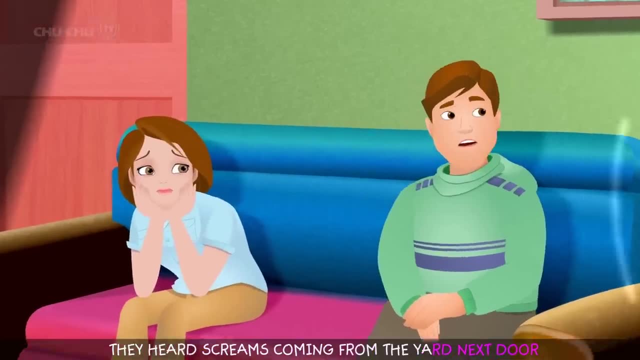 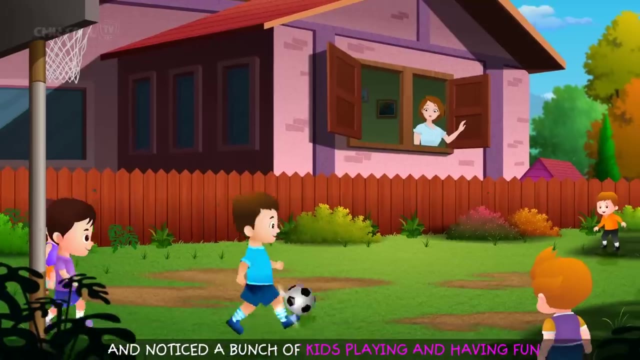 Nothing. Nothing seems to have gotten him away from his TV and video games. While the parents were talking, they heard screams coming from the yard next door. Cha-cha's mom peeked out the window and noticed a bunch of kids playing and having fun. 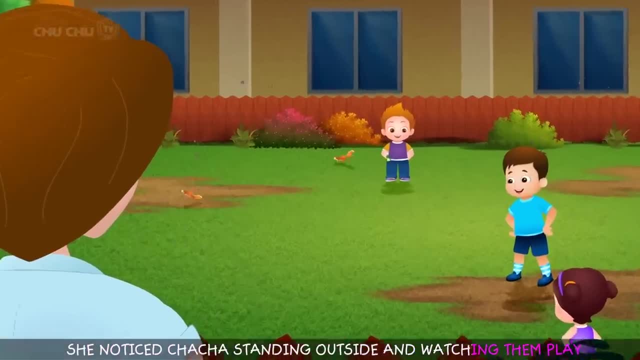 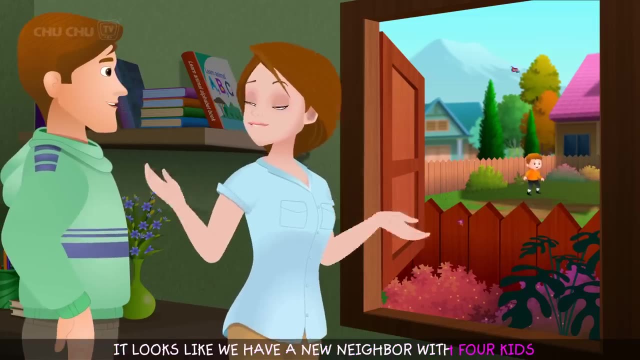 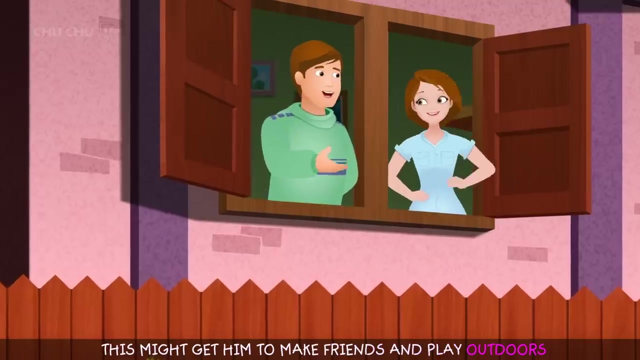 She noticed Cha-cha standing outside and watching them play. What are you looking at, Shh? It looks like we have a new neighbor with four kids. Look how he's staring at them playing. This might get him to make friends and play outdoors. 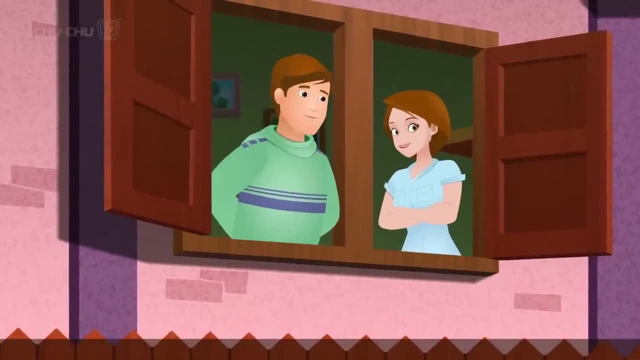 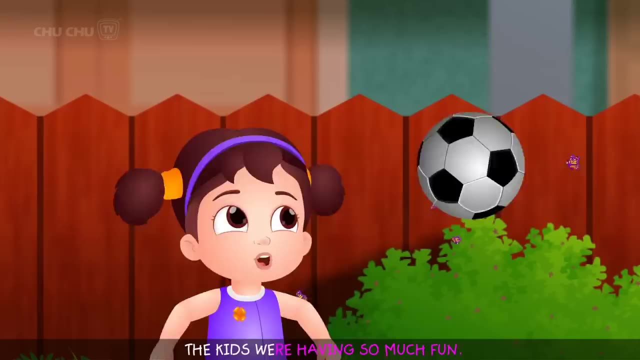 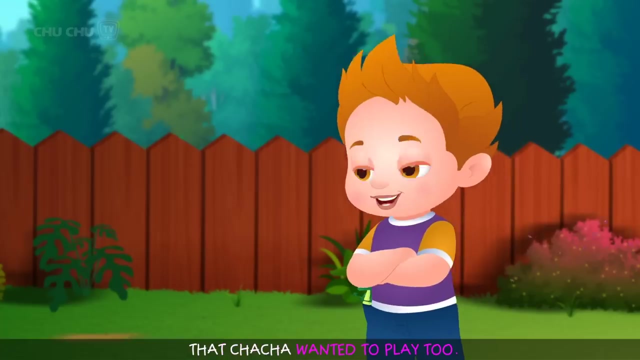 Let's sit and watch what he does. Cha-cha stood there watching the kids play basketball and soccer. The kids were having so much fun that Cha-cha wanted to play too, But Cha-cha had never played these games before, so he didn't know what to do.